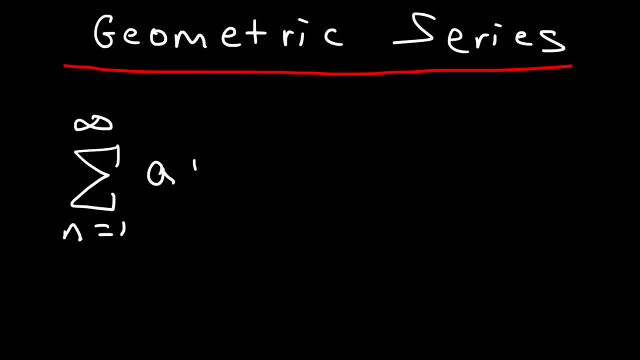 something like this: There's going to be a constant a and then your common ratio, r, is typically raised to the n or n minus 1 power, But your goal is to identify the value of r. So if r, that is, if the absolute value of r, is less, 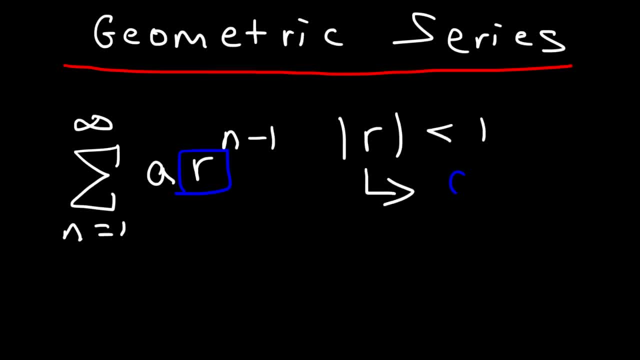 than 1,, then the series is going to converge. Now, if the absolute value of r is greater than or equal to 1, then the series will diverge. Now the next test you need to be familiar with is the p-series test. So the p-series is in the 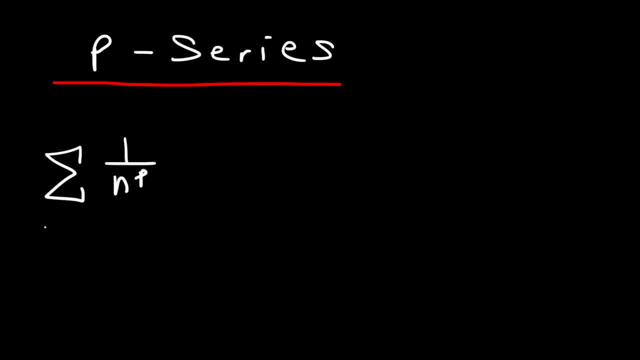 form of 1 over n raised to the p. So what you need to know is that if p is greater than 1, the series will converge, But if p is less than or equal to 1, then the series is going to diverge. 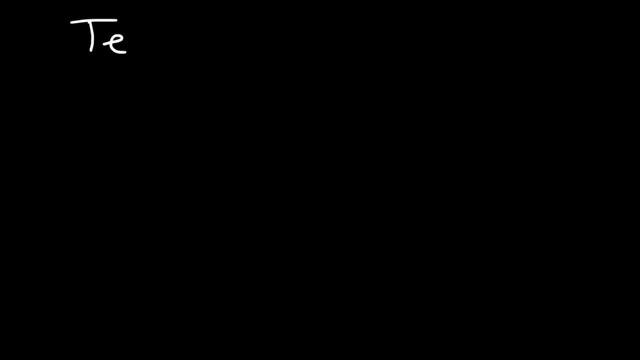 Next we have the telescoping series. Now, let's say, if you have a series where, when you write out the terms, it's like 1 minus 1 over 2 plus 1 over 2 minus 1 over 3 plus 1 over 3 minus 1 over 4.. And 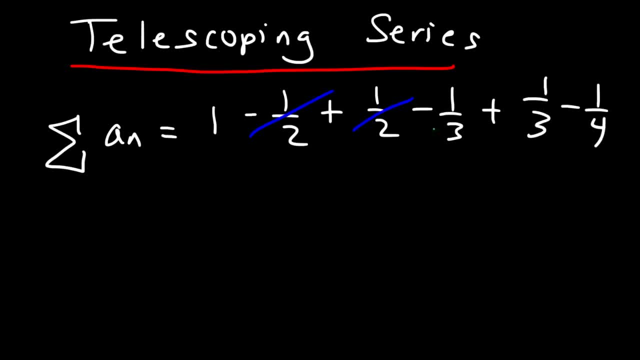 typically you can cancel the terms in the middle. So you can cancel the terms in the middle. Now what you want to do, because this will go to the general formula a-sub-n- You want to write a formula that will give you the partial sum of the telescoping series. It could be 1 minus a-sub-n. 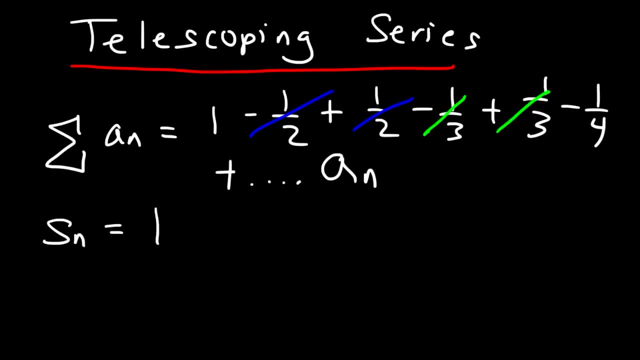 or 1 plus a-sub-n or something of that nature. But once you write the general formula for the partial sum, then you want to evaluate the sum of the series as n approaches infinity, which is going to be the limit, as n goes to infinity, of the partial sum formula. Now, if you get some 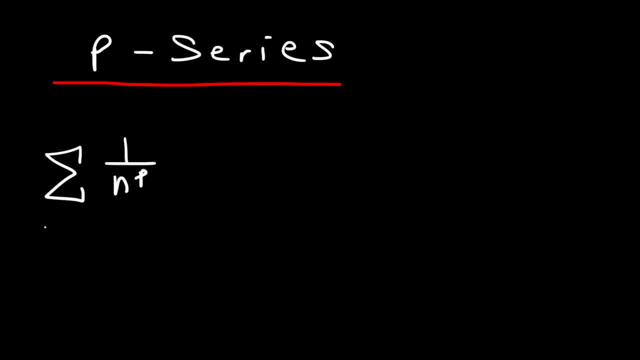 form of 1 over n raised to the p. So what you need to know is that if p is greater than 1, the series will converge, But if p is less than or equal to 1, then the series is going to diverge. 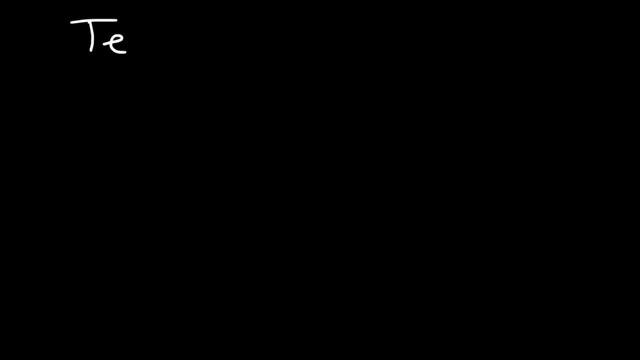 Next we have the telescoping series. Now, let's say, if you have a series where, when you write out the terms, it's like 1 minus 1 over 2 plus 1 over 2 minus 1 over 3 plus 1 over 3 minus 1 over 4.. And 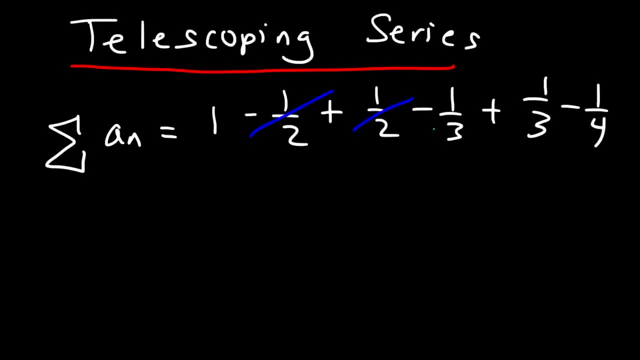 typically you can cancel the terms in the middle. So you can cancel the terms in the middle. Now what you want to do, because this will go to the general formula a sub n. you want to write a formula that will give you the partial sum of the. 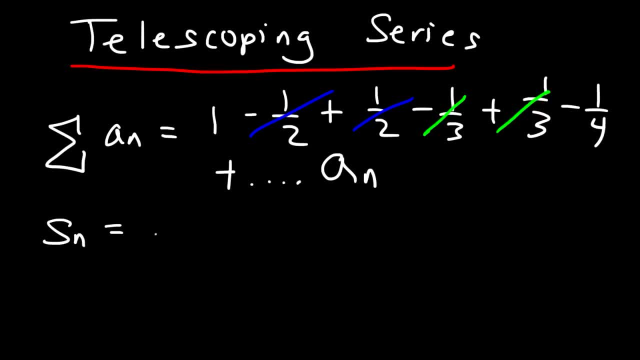 telescope and series. It could be 1 minus a sub n or 1 plus a sub n, or something of that nature. Once you write the general formula for the partial sum, then you want to evaluate the sum of the series as n approaches infinity, which is: 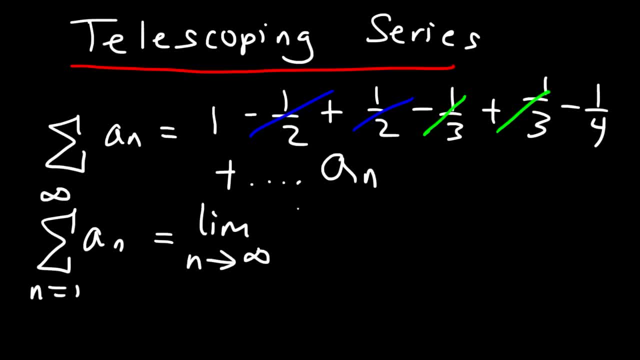 going to be the limit, as n goes to infinity, of the partial sum formula. Now, if you get some finite value, let's call L, then that means that the series converges, which is usually the case. Now, if you get, let's say, plus or minus infinity or doesn't exist, then the 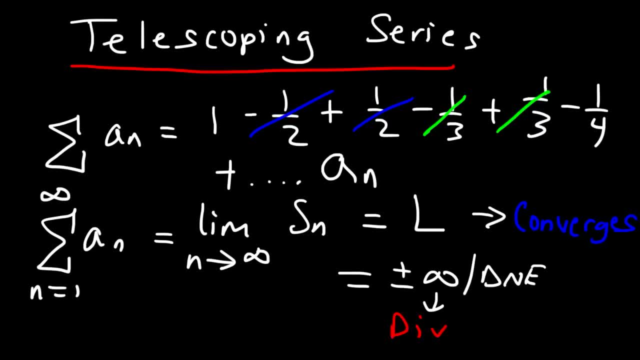 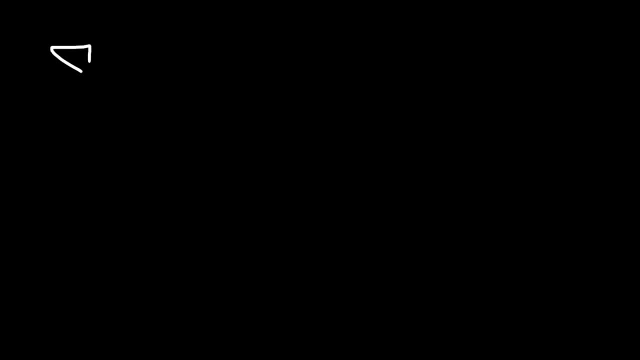 series is divergent. So here is a typical example of a telescoping series problem. Let's say, if you have the series from 1 to infinity of 1 over n minus 1 over n plus 1. That's a telescoping series problem. If you list out the terms, it's. 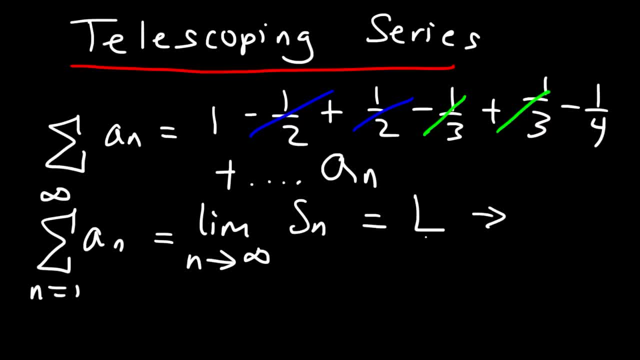 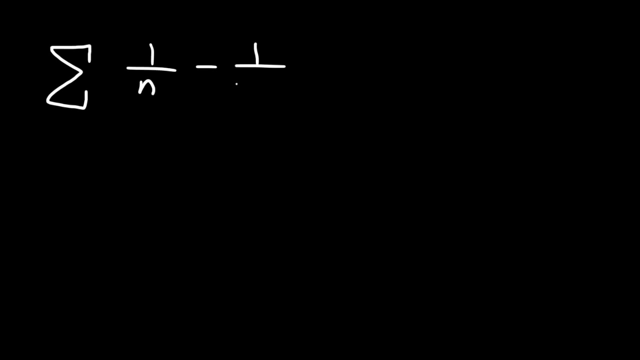 finite value- let's call L- then that means that the series converges, which is usually the case. Now, if you get, let's say, plus or minus infinity, or doesn't exist, then the series is divergent. So here is a typical example of a telescoping series problem. Let's say: if 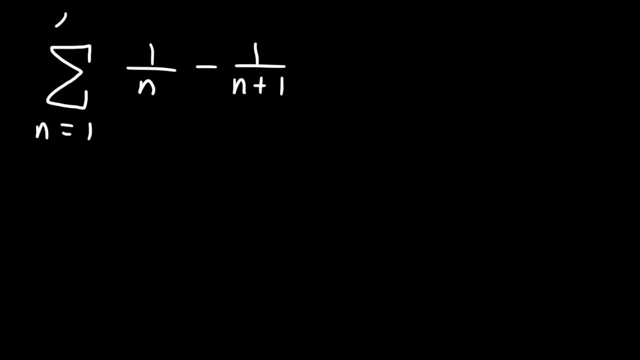 you have the series from 1 to infinity of 1 over n, minus 1 over n plus 1, that's a telescoping series problem. If you list out the terms, it's gonna be 1 over 1, minus 1 over 2, and then plus 1 over 2, minus 1 over 3, and so forth. now 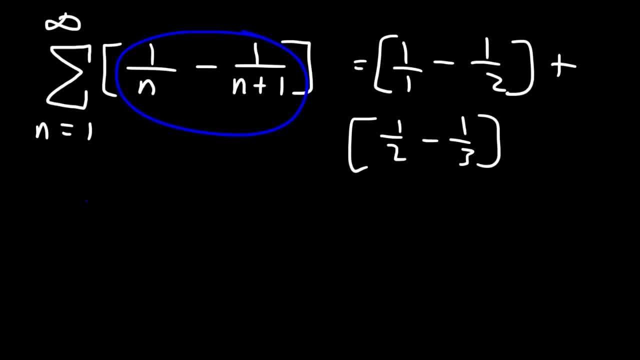 sometimes you may not have two separate fractions. you may only have a single fraction and you need to use partial fraction decomposition to split it into two separate fractions and then you can list out the terms. so watch out for the telescope and series problem. you need to keep an eye out for that one now. the 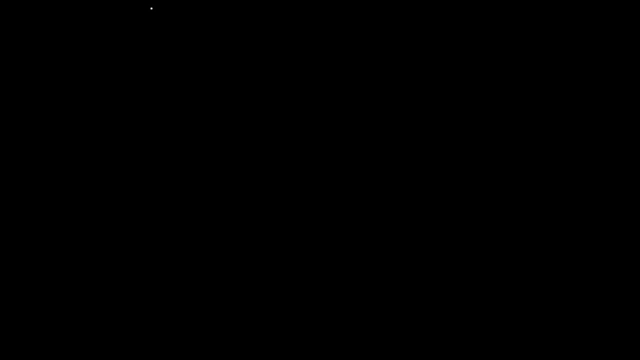 next test you need to be familiar with is the integral test. so what do you recall about the integral tests? so let's say, if we have the sequence a sub n and we're going to make it equal to a function of n, F has whispered: 5, 2, 1, zero. 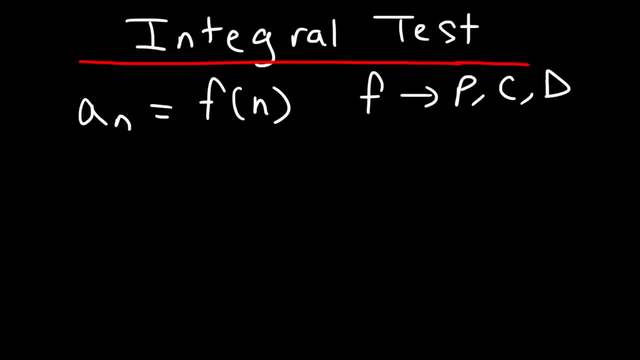 It has to be positive, continuous and a decreasing function And it has to be decreasing from some number n to infinity. So the long-term trend is it has to be decreasing. Sometimes it can go up initially, but as long as it's decreasing for the long run it can work. 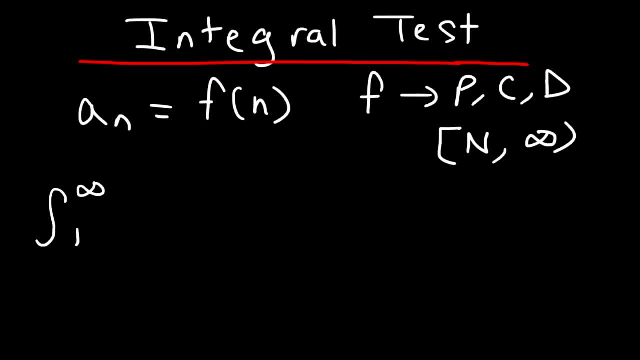 So what you need to do is take the integral from 1 to infinity of f, of x, dx, And let's say: if you get some finite value out, then that means that the series, the original series, converges. Now let's say, if you get plus or minus infinity, or you get an answer where it doesn't exist, then the original series diverges. 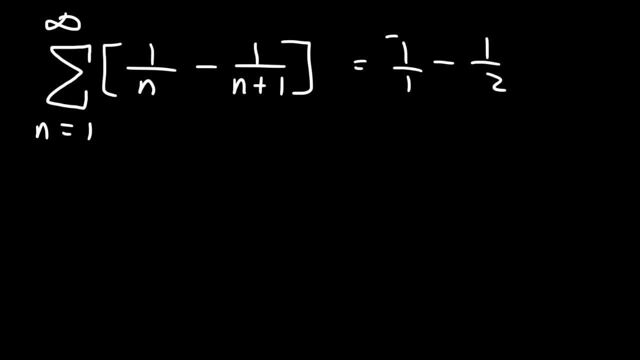 going to be 1 over 1, minus 1 over 2, and then plus 1 over 2 minus 1 over 3, and so forth. Now sometimes you may not have two separate fractions, You may only have a single fraction and 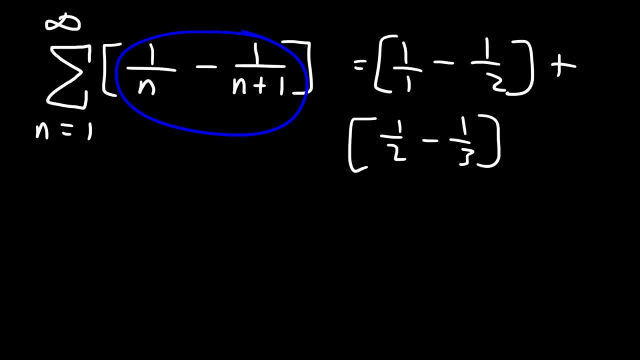 you need to use partial fraction decomposition to split it into two separate fractions and then you can list out the terms. So watch out for the telescoping series problem. You need to keep an eye out for that one. Now the next test you need to be familiar with is the integral test. 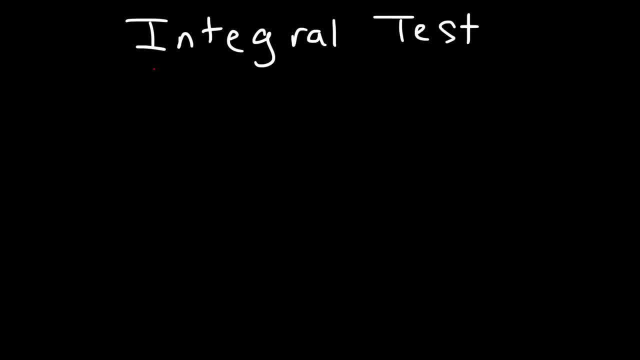 So what do you recall about the integral test? So let's say, if we have a sequence, a sub n, and we're going to make it equal to a function of n, f has to be positive, continuous and a decreasing function, And 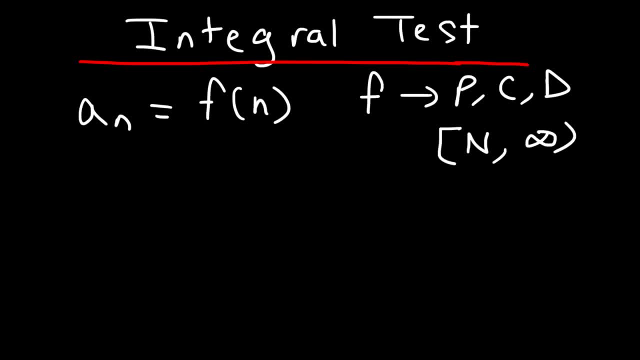 it has to be decreasing from some number n to infinity. So the long-term trend is it has to be decreasing. Sometimes it can go up initially, but as long as it's decrease in for the long run it can work. So what you need to do is take the integral. 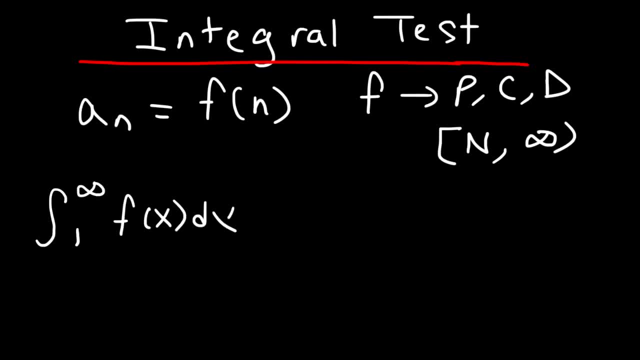 from 1 to infinity of f, dx. and let's say: if you get some finite value out, then that means that the series, the original series, converges. Now let's say, if you get plus or minus infinity or you get an answer where it doesn't exist, then the original 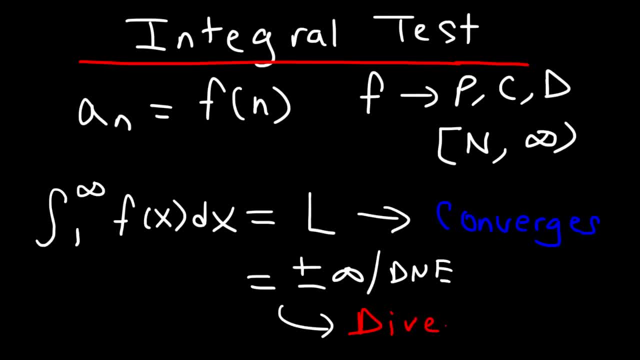 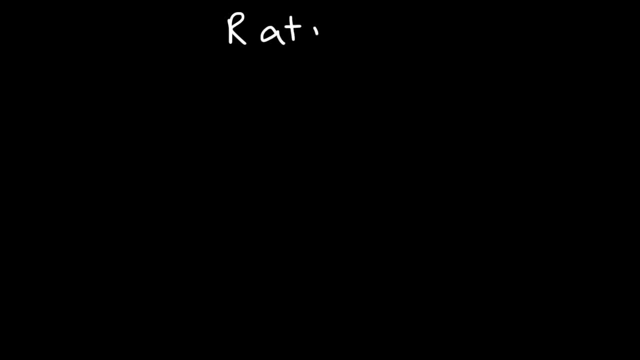 series diverges, And so that's the integral test. The next one we're going to talk about is the ratio test. In this case, you need to take the limit- as n goes to infinity- of the absolute value of a sub n plus 1 divided by a sub n. Now, if your result is less than 1, then the series. 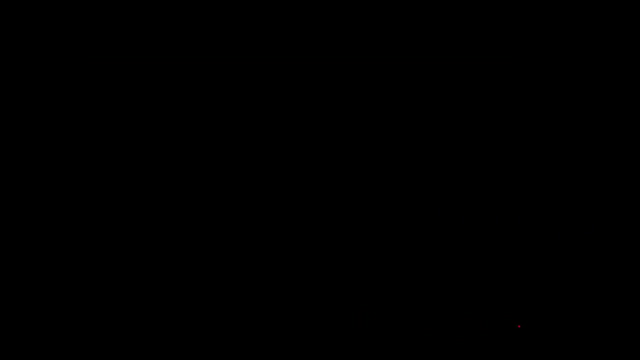 And so that's the integral test. The next one we're going to talk about Is the ratio test. In this case, you need to take the limit- as n goes to infinity- of the absolute value of a sub n plus 1 divided by a sub n. 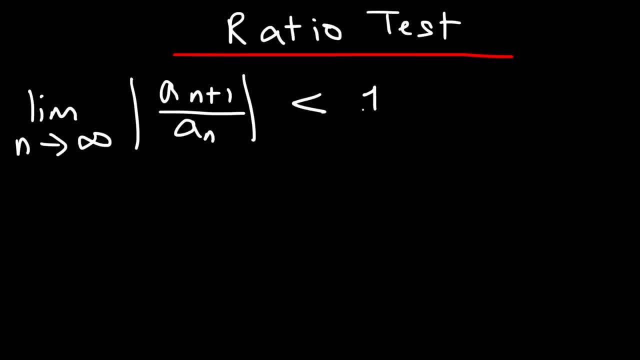 Now, if your result is less than 1,, then the series converges. If your result is greater than 1, or if it goes to, let's say, plus positive infinity. negative infinity won't apply here, because your final answer has to be positive. 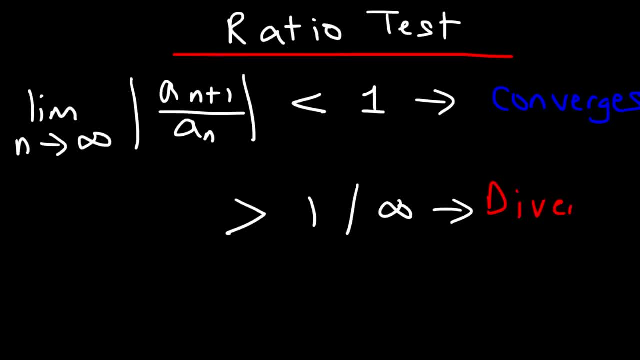 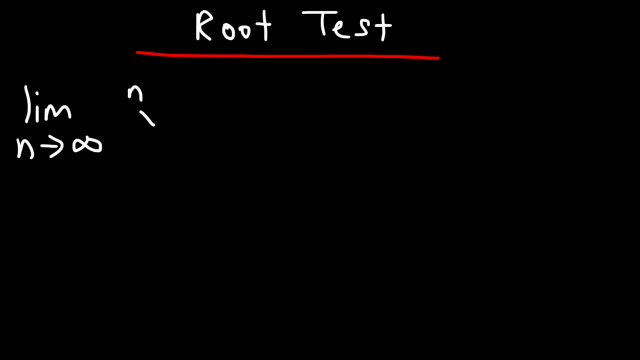 Then the series will diverge. Now, if the limit is equal to 1, then the ratio test is inconclusive. Next up is the root test. So what you need to do is take the limit, as n goes to infinity, of the f root of the absolute value of a sub n. 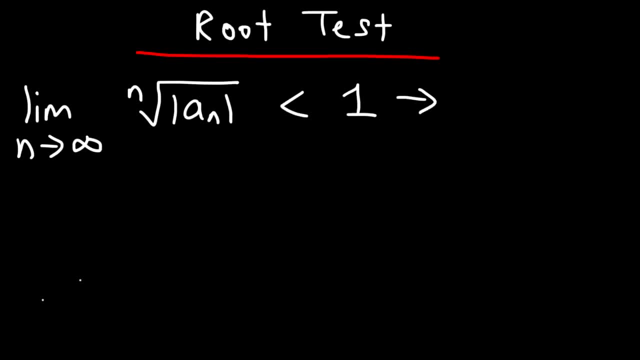 Now, if you get an answer that's less than 1, then the series converges. Now, if you get a value where it's greater than 1, or if it goes to infinity, then the series diverges. If your answer is equal to 1, then, like the ratio test, the root test will become inconclusive. 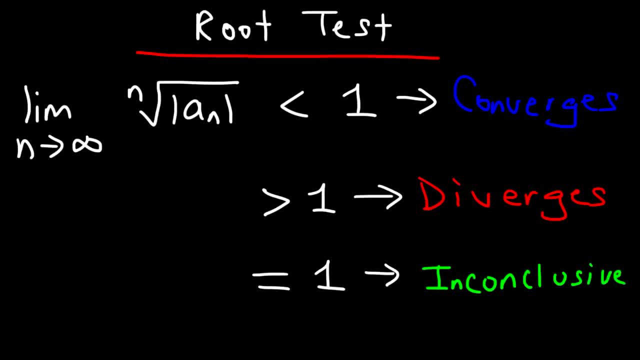 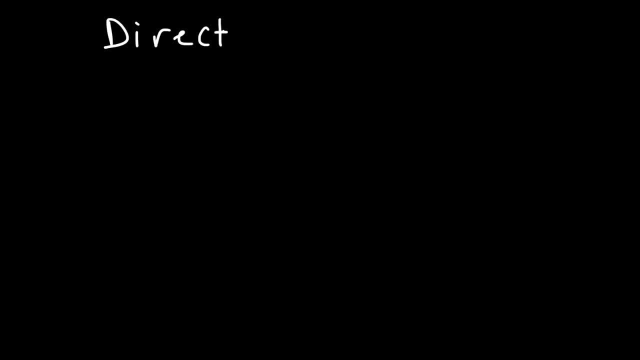 And so you may need to use another test to get the answer, to determine if the series is going to converge or diverge. Now let's talk about the direct comparison test. What do you remember about this test? Well, first, we need to have two sequences: a sub n and b sub n. 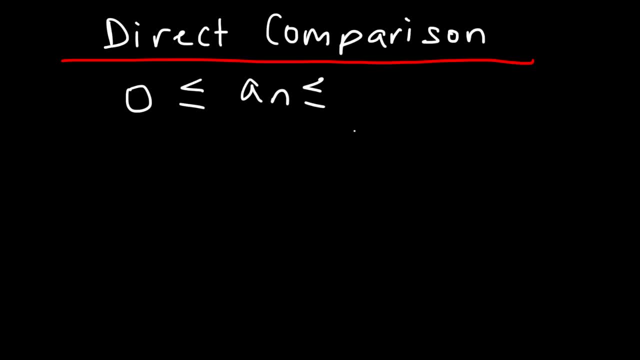 So let's say b sub n is the big sequence and a sub n is the small sequence. And so here's the basic idea behind the direct comparison test. So if the big series converges, then the small series will converge as well. 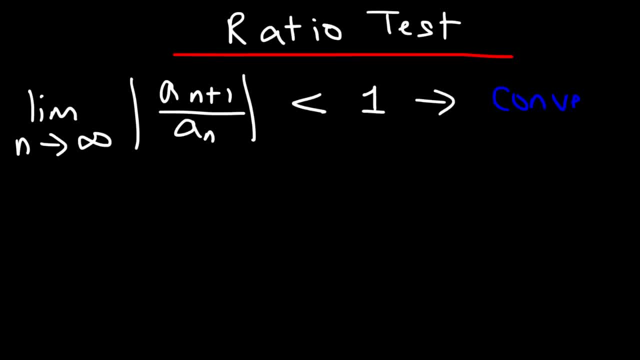 converges. If your result is greater than 1, or if it goes to, let's say, plus positive infinity- negative infinity won't apply here, because your final answer has to be positive- Then the series will diverge. Now, if the limit is equal to 1, then the ratio test is inconclusive. 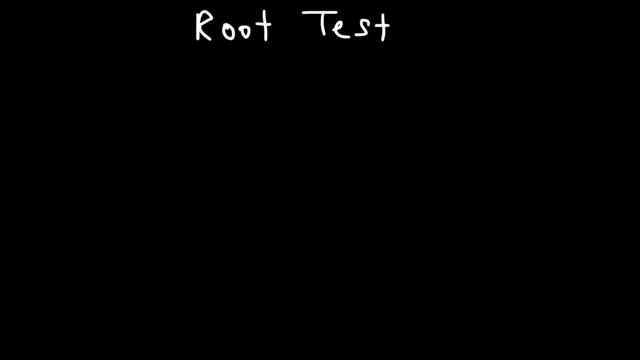 Next up is the root test. So what you need to do is take the limit, as n goes to infinity, of the nth root of the absolute value of a sub n. Now, if you get an answer that's less than 1, then the series converges. 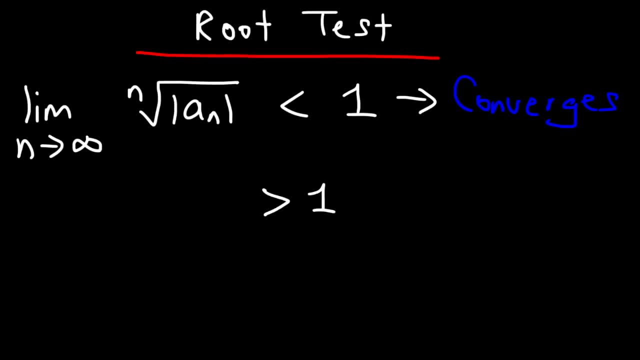 Now, if you get a value where it's greater than 1, or if it goes to infinity, then the series diverges. If your answer is equal to 1, then, like the ratio test, the root test will become inconclusive. 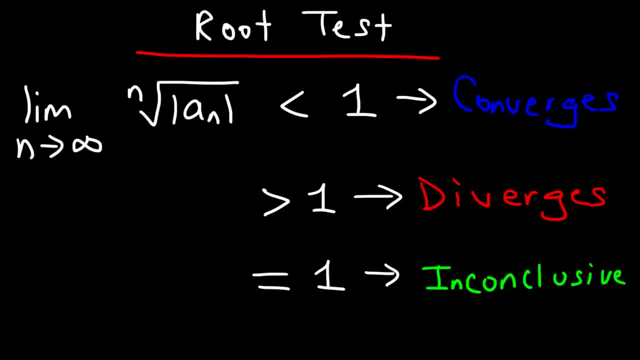 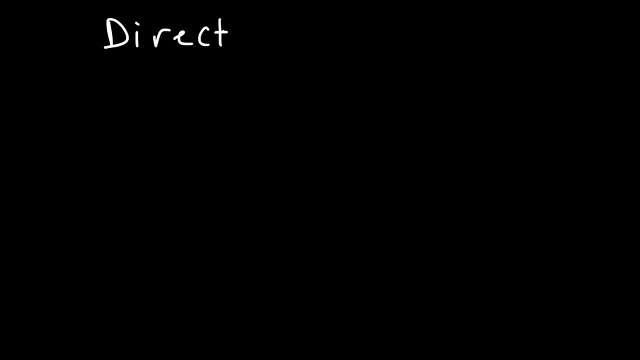 And so you may need to use another test to get the answer, to determine if the series is going to converge or diverge. Now let's talk about the direct comparison test. What do you remember about this test? Well, first we need to have two sequences. 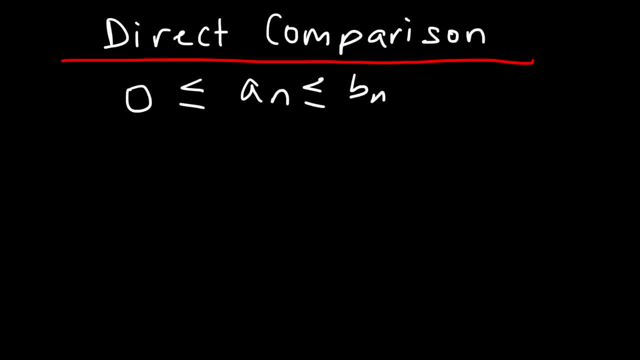 A sub n and B sub n. So let's say B sub n is the big sequence and A sub n is the small sequence. And so here's the basic idea behind the direct comparison test. So if the big series converges, then the small series will converge as well. 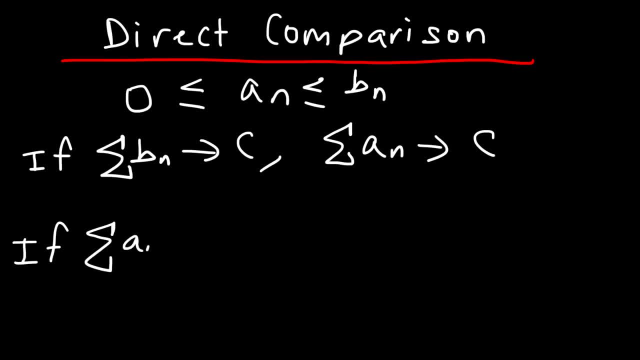 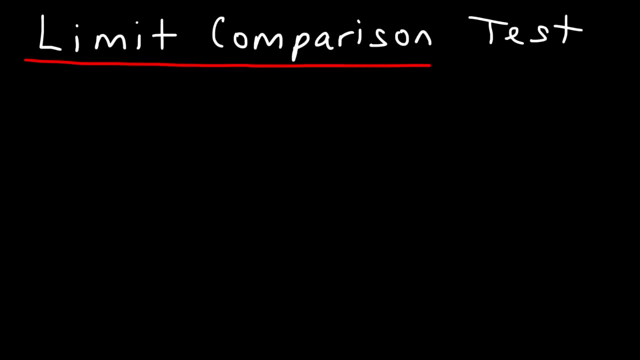 Likewise, if the small series diverges, then the big series diverges as well. Now let's talk about the limit comparison test. This test is very similar to the ratio test. The only difference is you're dealing with two different sequences. 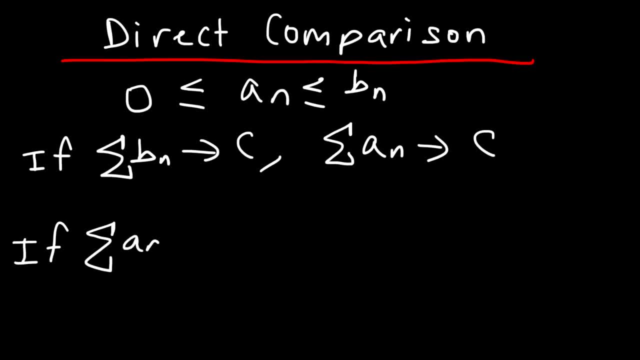 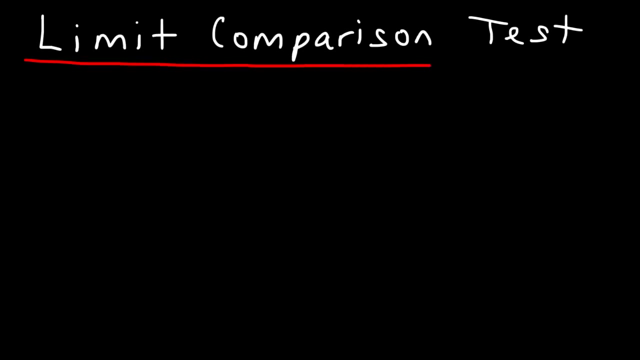 Likewise, if the small series diverges, then the big series diverges as well. Now let's talk about the limit comparison test. This test is very similar to the ratio test. The only difference is you're dealing with two different sequences as opposed to one. 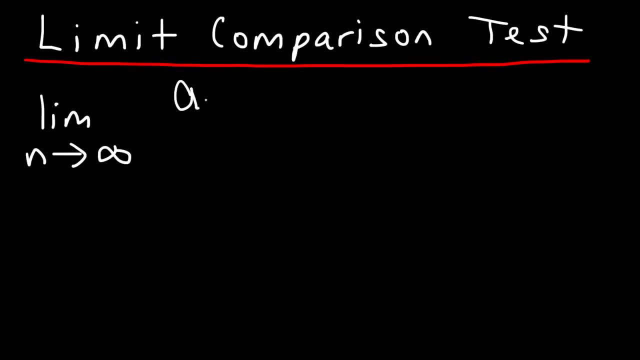 So you need to take the limit- as n goes to infinity- of a sub n divided by b sub n. You need to show that this is equal to some finite positive number, which we'll call l, And if that's the case, then both series will either converge or both series will diverge. 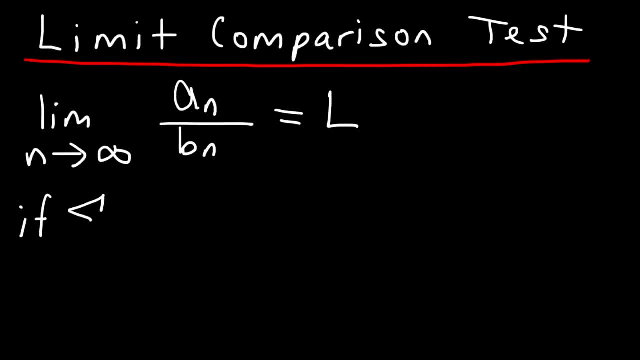 So let's say: if you know that this series converges And if you pass the limit comparison test, then you can say that the series with b, sub n, that's going to converge as well. Or let's say: if this series diverges, then you know this series, the other one will diverge as well. 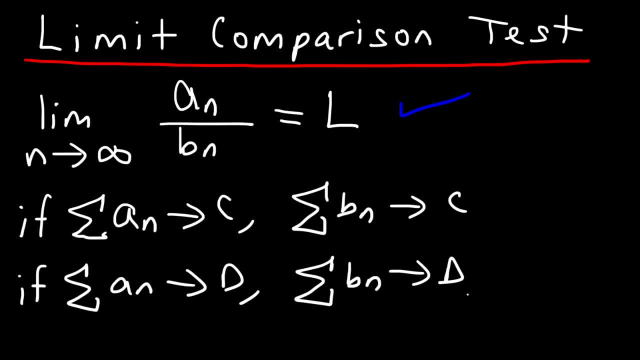 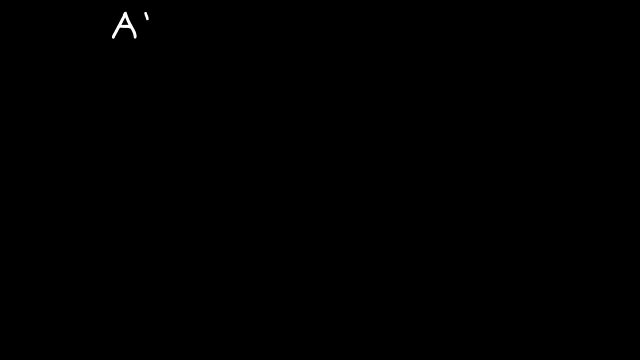 So either they both converge or they both diverge, And that's the basic idea behind the limit comparison test. If you know the convergence or divergence of one series, then you can determine the convergence or divergence of another series. Next up is the alternating series test. 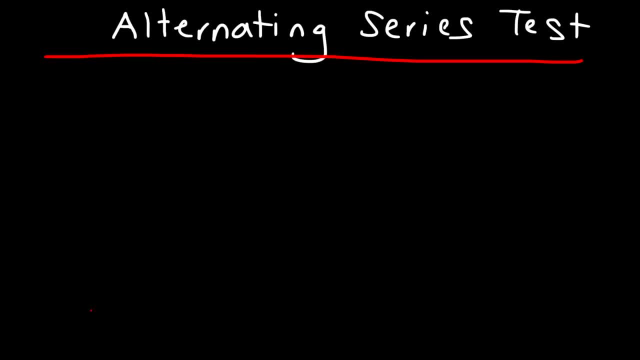 And this is when you have a series with alternating signs. So typically it's in this form: You're going to have negative one raised to the n or n, plus one times some sequence, a sub n, And in order to determine if the series will converge, two conditions must be met. 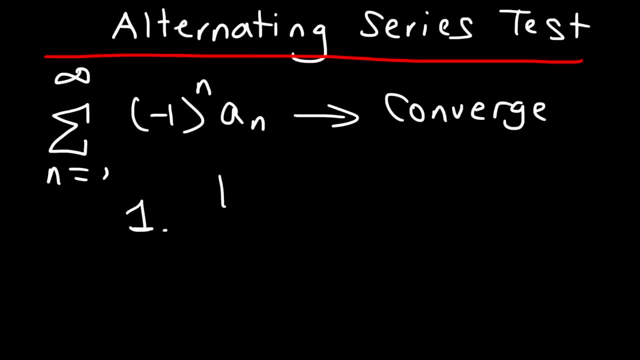 The first condition is that it has to pass the divergence test. So you need to take the limit as n goes to infinity, And you need to show that It's zero. If it's not zero, then the series diverges. If it's zero, then you need to move on to step two. 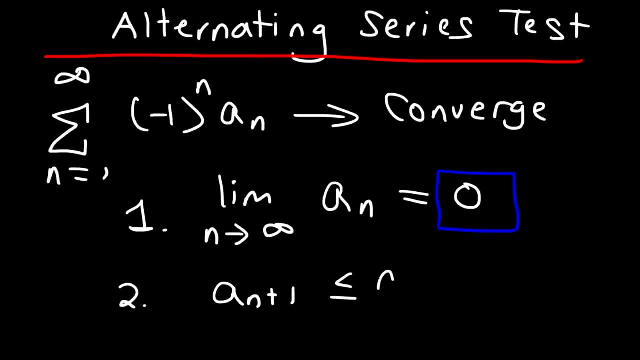 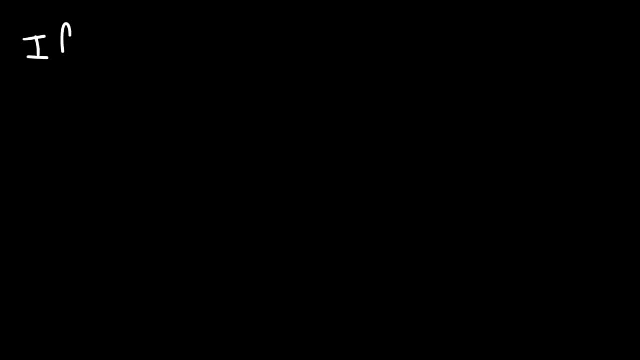 You need to show that the sequence is decreasing. So a sub n has to be equal to or greater than a sub n plus one. The next thing you could try is the absolute value test. So let's say, if The absolute value of the series converges. 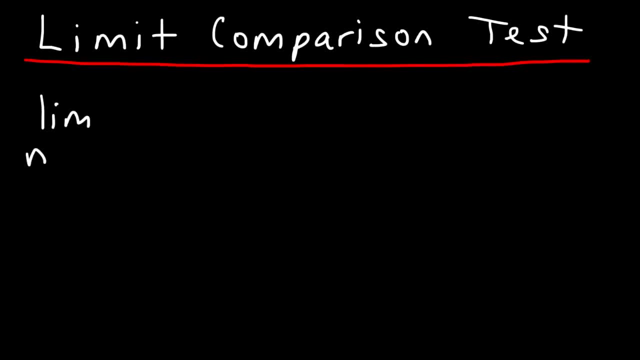 as opposed to one. So you need to take the limit, as n goes to infinity, of A sub n divided by B sub n. You need to show that this is equal to some finite positive number, which we'll call L, And if that's the case, 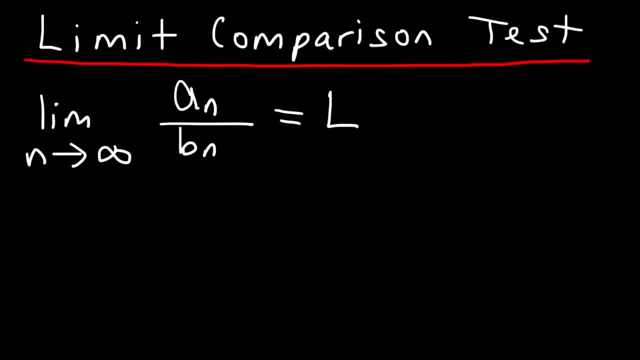 then both series will either converge or both series will diverge. So let's say, if you know that this series converges and if you pass the limit comparison test, then you can say that the series with B sub n, that's going to converge as well. 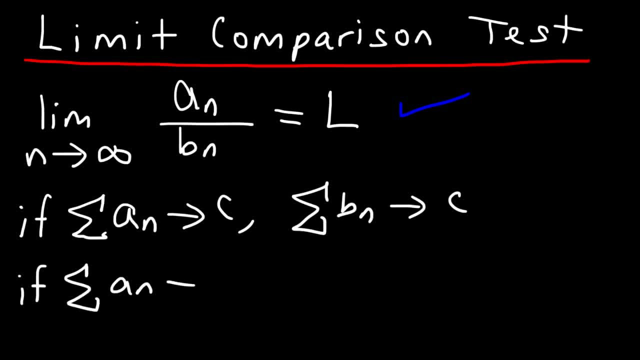 Or let's say: if this series diverges, then you know this series. the other one will diverge as well. So either they both converge or they both diverge, And that's the basic idea behind the limit comparison test. If you know the convergence or divergence of one series, 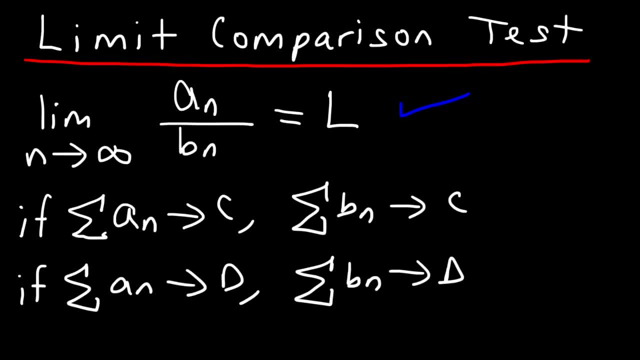 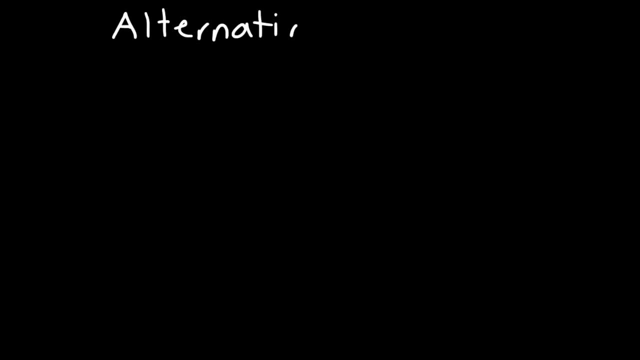 then you can determine the convergence or divergence of another series. Next up is the alternating. It means you can perform a series test with a series of words. So what we're going to do here is we're going to perform a series test with the full number. 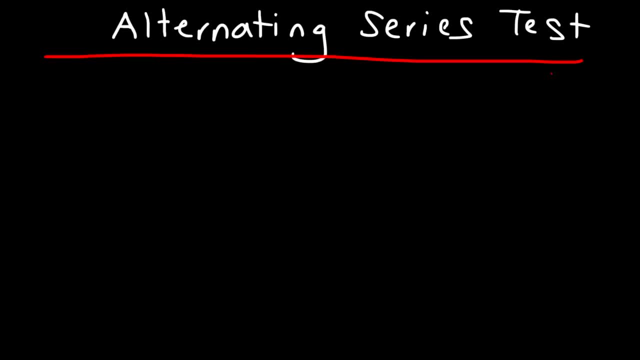 using the Hoang and Song axioms, using the continuous Helm's control system, and this is going to be one such test that we're going to show in the next video. The kicks to that system is a ke tiposime test. This is based on the questions we had. 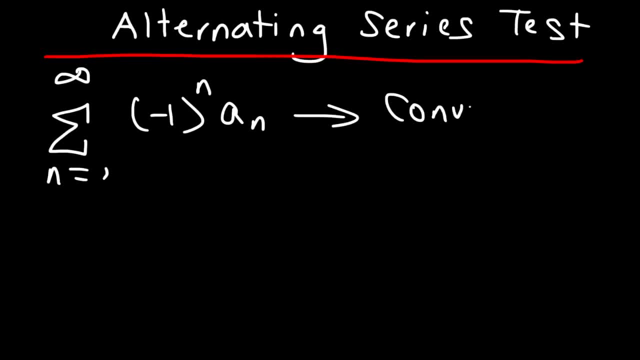 like: where is the lowest string? two conditions must be met. The first condition is that it has to pass the divergence test. So you need to take the limit, as n goes to infinity, and you need to show that it's 0. If it's not 0,, then the series diverges. If it's 0,, then you. 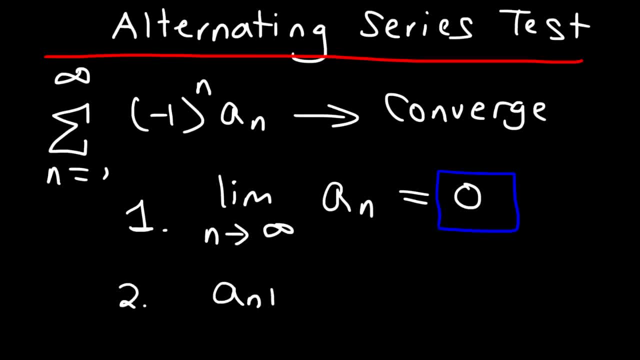 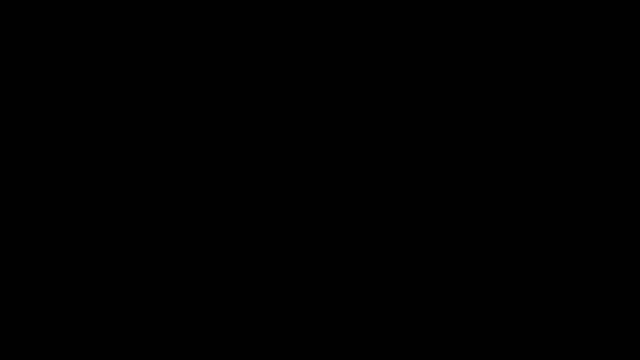 need to move on to step 2.. You need to show that the sequence is decreasing. So a sub n has to be equal to or greater than a sub n plus 1.. The next thing you could try is the absolute value test. So let's say, if the absolute value of the 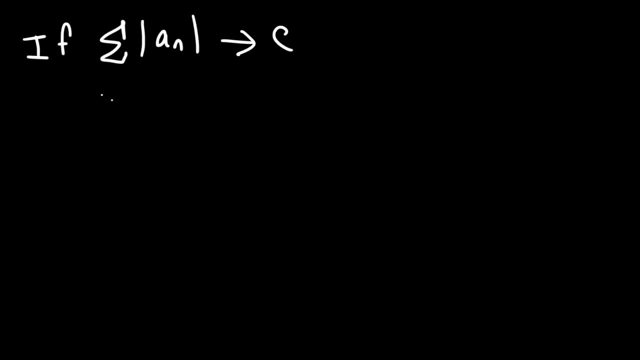 series converges, then the original series will also converge And when this happens, you can say that the series, the original series, is absolutely convergent. Now let's say, if you take the absolute value of the series and you find that it diverges, And you take, you analyze the original series, 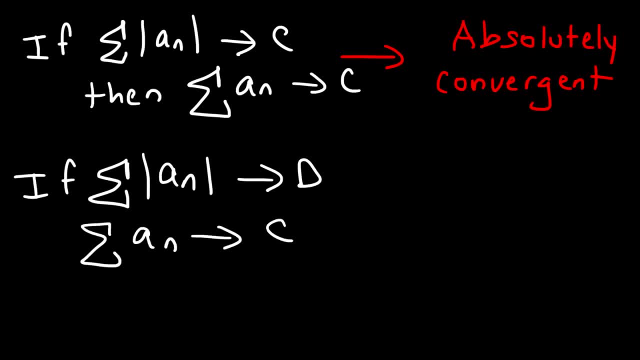 but it doesn't diverge. Let's say it's convergent. If the original series is convergent, then the original series is conditionally convergent. Let's say that the whole series converges and the series diverges. Now let's 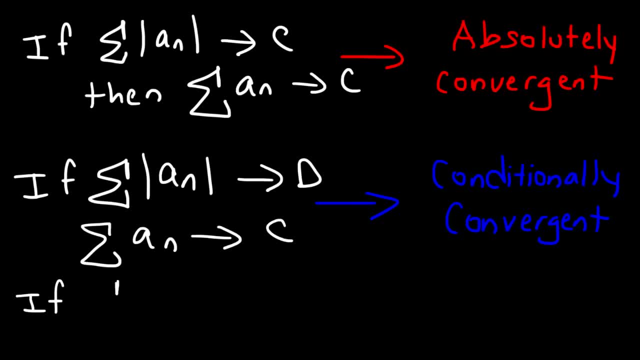 say, if you analyze the absolute value of the series and you find it to be divergent, then you check the original series and that's divergent as well. Then the whole series is simply divergent. There's nothing to be said about it. So let's say: if we have the series, 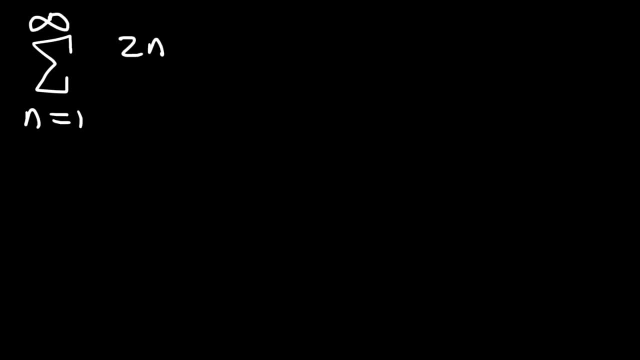 from 1 to infinity: 2n squared plus 5 over 7n squared minus 4.. So what do you think we need to do for this problem? Which test should we use? If you're not sure? it's always good to start with. 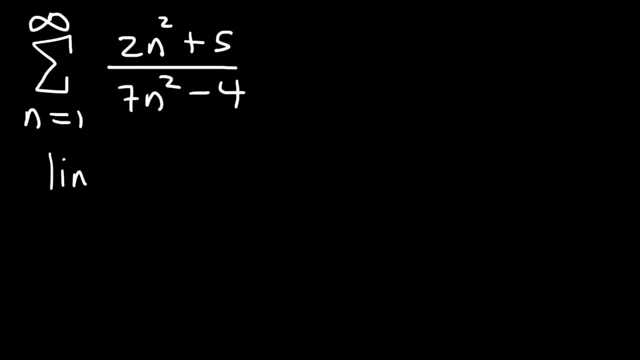 the divergence test. So let's take the limit, as n goes to infinity- of a sub n. Now, a sub n is what we see here. So what's the limit equal to? If you want to, you can use L'Hopital's rule. 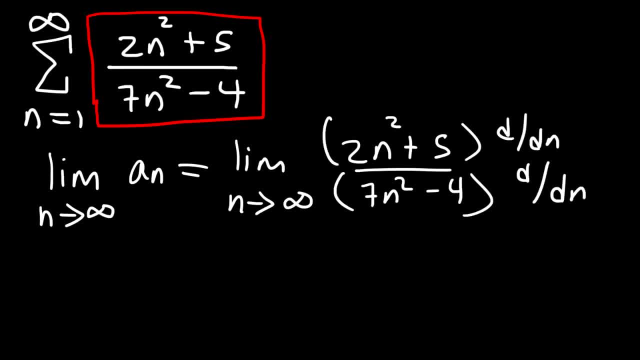 So let's take the derivative of the numerator and the denominator, So the derivative of 2n squared, that's going to be 4n, And the derivative of 7n squared is 14n, And then what we could do is use L'Hopital's rule. one more: 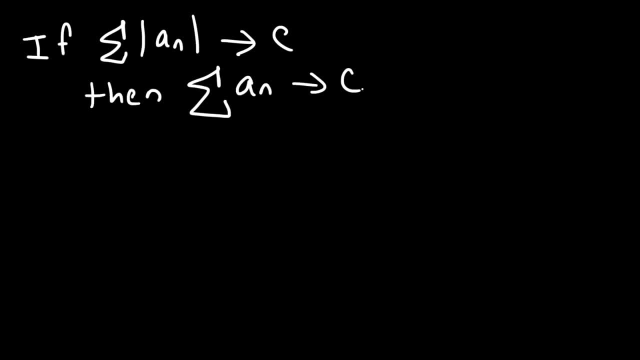 Then the original series will also converge And when this happens, you can say that the series, the original series, is absolutely convergent. Now let's say, if you take the absolute value of the series And you find that it diverges, 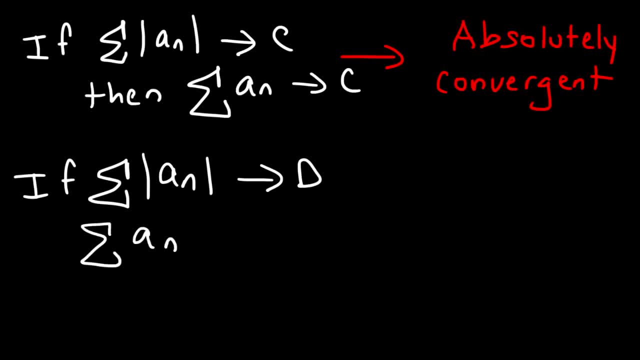 And you take, you analyze the original series, But it doesn't diverge. Let's say it's convergent. If the original series is convergent, Then the original series is conditionally convergent. Now Let's say, if You analyze the absolute value of the series, 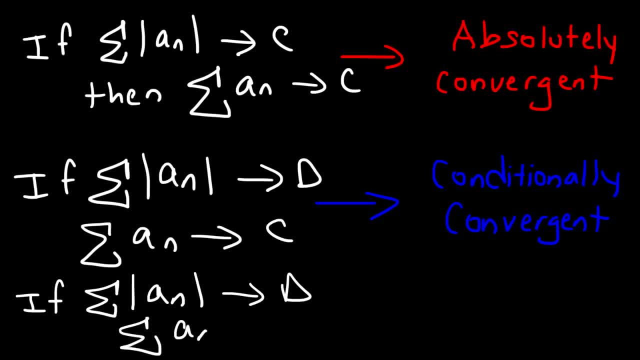 And you find it to be divergent, Then you check the original series And that's divergent as well. Then the whole series is simply divergent. There's nothing to be said about it. So let's say, if we have the series, 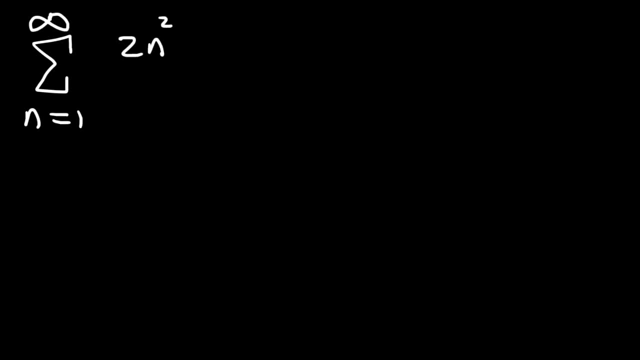 From one to infinity: Two n squared plus five Over seven n squared minus four. So what do you think we need to do for this problem? Which test should we use? If you're not sure, It's always good to start with the divergence test. 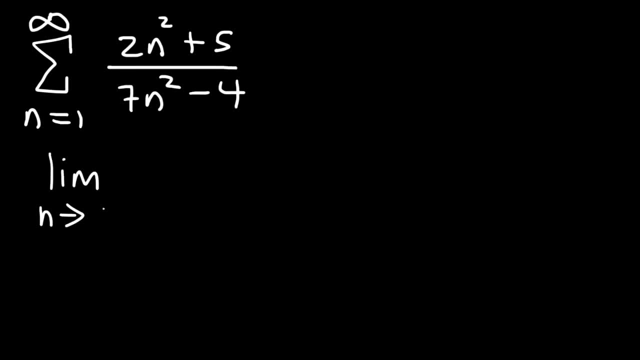 So let's take the limit- As n goes to infinity- Of a sub n. Now, a sub n is what we see here. So what's the limit equal to? If you want to, You can use L'Hopital's rule. 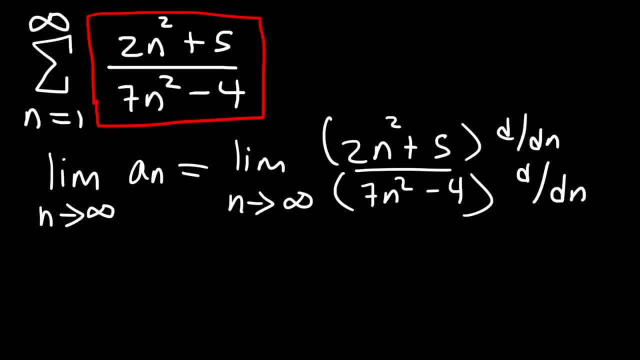 So let's take the derivative of the numerator And the denominator, So the derivative of two n squared, That's going to be four n, And the derivative of seven n squared is fourteen n. And then what we could do Is use L'Hopital's rule one more time. 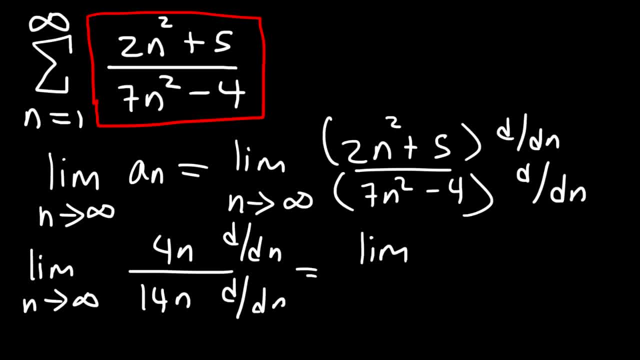 time, And so this is going to be 4 over 14, which reduces to 2 over 7.. So notice that the limit, as n goes to infinity of a sub n, it doesn't equal 0. Therefore, the original series. 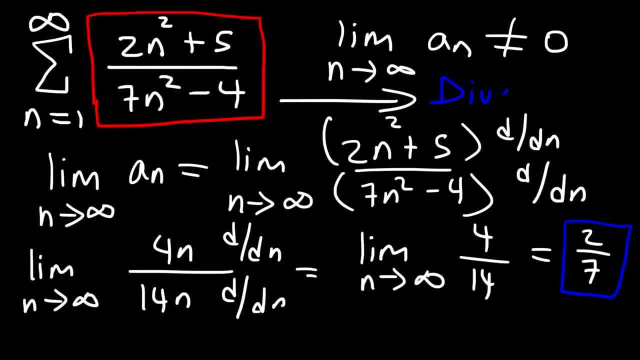 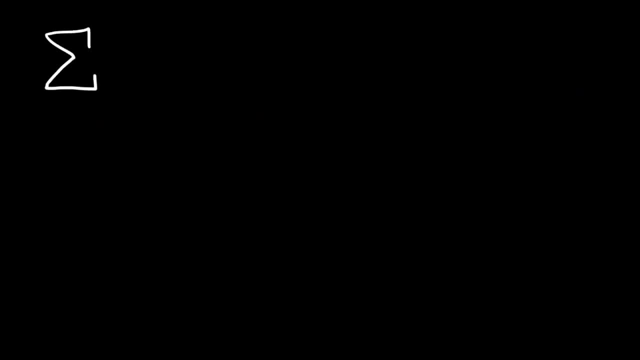 is divergent according to the divergence test. And that's it for this problem. Consider this series. Let's say, if we have the cube root of n divided by n to the fifth power, Will the series converge or will it diverge? So which test would you use here? 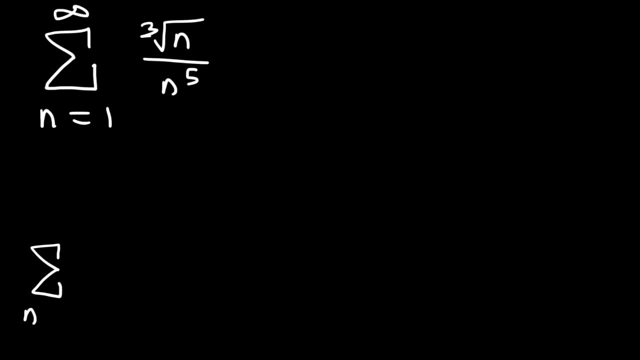 Notice that we can put the series in this form. You can simplify it or reduce it to this form. So we're dealing with a p-series. So the cube root of n, that's n to the one-third, And let's divide it by n to the fifth. 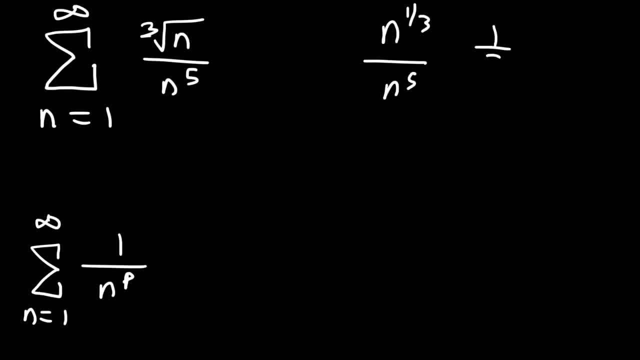 So we need to subtract the exponents. What's 1 over 3 minus 5?? So, again in common denominators, let's multiply this by 3 over 3.. And so this is 1 over 3, minus 15 over 3.. So that's going to be. 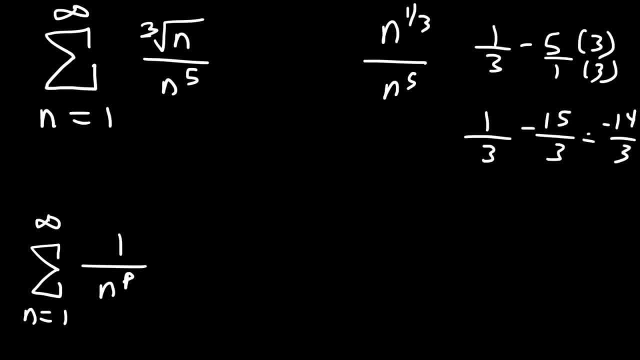 negative 14 over 3.. So we can rewrite the series like this: So we have n to the negative 14 over 3, which we can rewrite that as 1 over n to the 14 over 3.. So now it's in the proper format So we can clearly see. 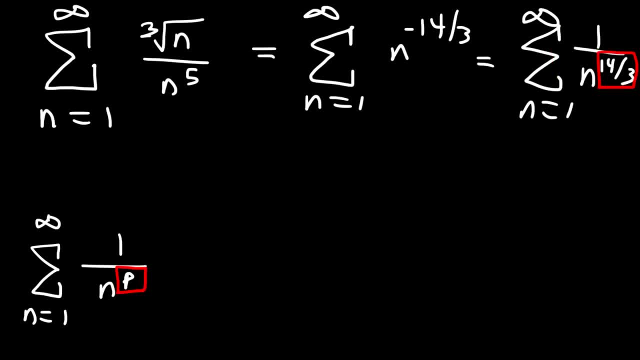 that p is equal to 14 over 3. And 14 over 3 is greater than 1.. So p is greater than 1.. And for the p-series, if p is greater than 1, then the series converges. 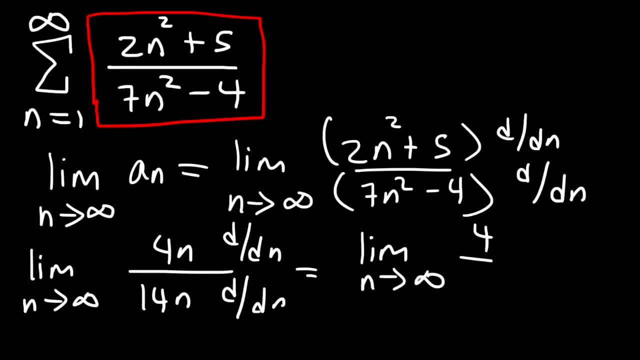 And so this is going to be four over fourteen, Which reduces to two over seven. So notice that The limit As n goes to infinity Of a sub n, It doesn't equal zero. Therefore The original series Is divergent. 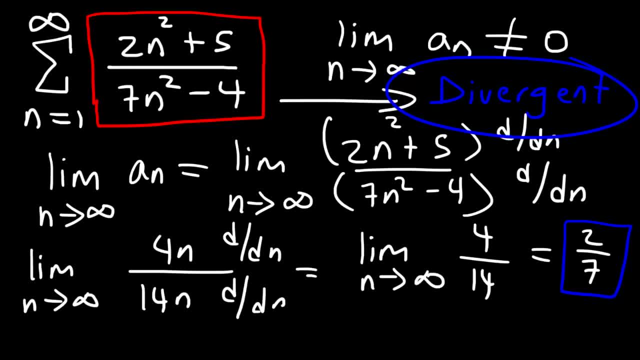 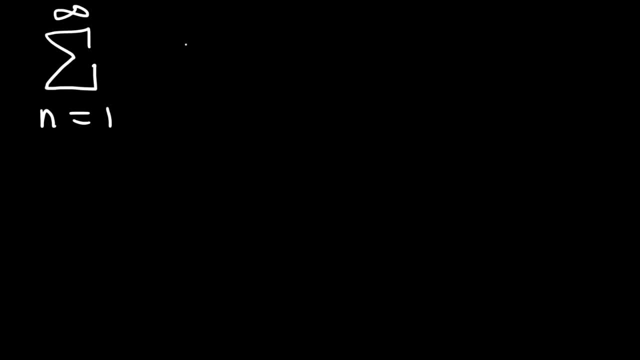 According to the divergence test. And that's it for this problem. Consider this series. Let's say, if we have The cube root of n Divided by n to the fifth power, Will the series converge Or will it diverge? 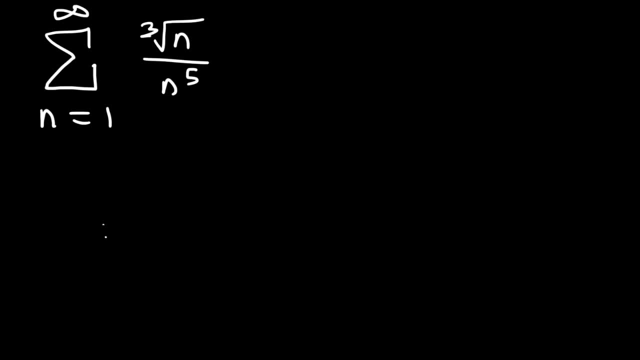 So which test would you use here? Notice that We can put the series In this form. You can simplify it or reduce it To this form. so We're dealing with a p-series. So the cube root of n, That's n to the one third. 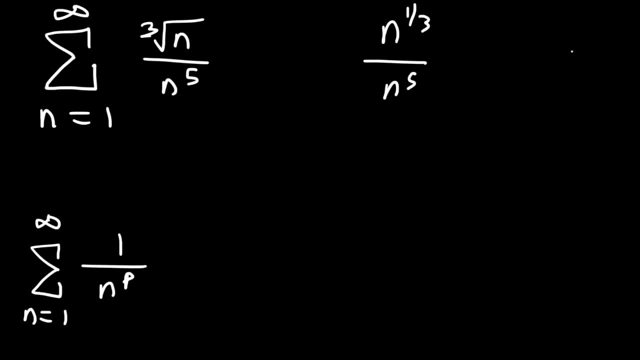 And let's divide it by n to the fifth. So we need to subtract the exponents. What's one over three minus Five. So, again in common denominators, Let's multiply this by three over three, And so this is one over three minus fifteen. 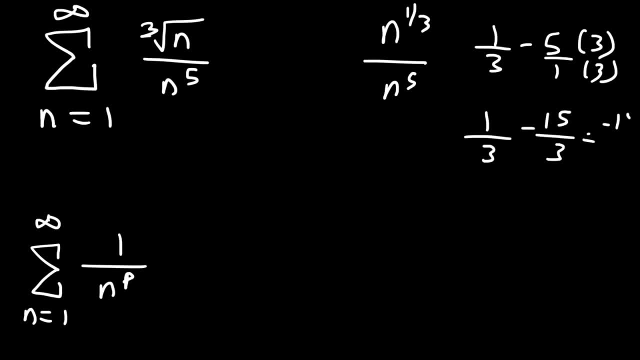 Over three. so that's going to be Negative fourteen over three. So we can rewrite the series Like this: So we have n To the negative fourteen over three, Which we can rewrite that As one over n To the fourteen over three. 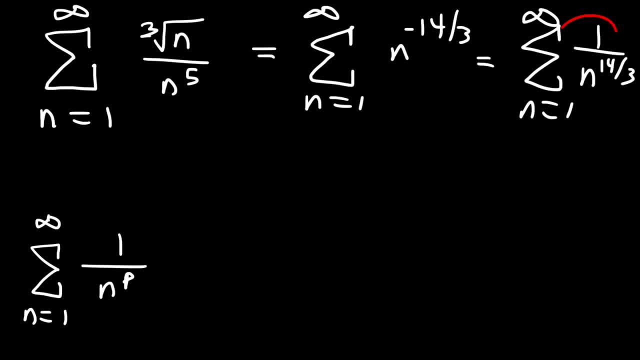 So now It's in the proper format. So we can clearly see that p Is equal to fourteen over three, And fourteen over three Is greater than one, so p Is greater than one In this case. If p is greater than one, 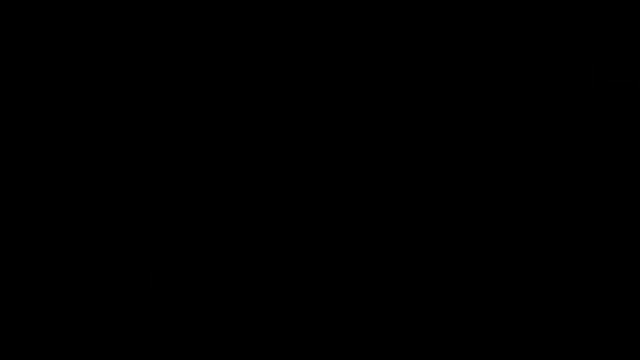 Then the series Converges. Now let's try another problem. So let's say, this is five Times one, fourth Raised to the n minus one. What type of series do we have? Notice that it's in this form. So what we have is a geometric series. 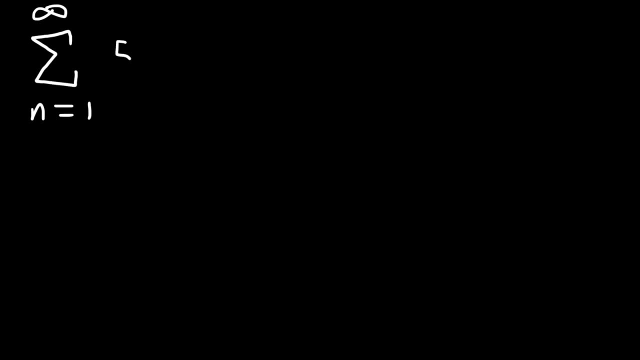 Now let's try another problem. So let's say this is 5 times 1, fourth raised to the n minus 1.. What type of series is this? What series do we have? Notice that it's in this form. So what we have is a geometric series. So the common ratio is 1 over 4.. 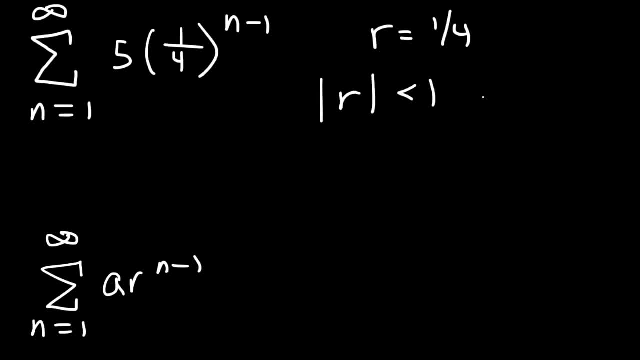 Now recall that if the absolute value of r is less than 1, the series converges for geometric series, And if it's greater than or equal to 1, the series diverges. 1 fourth is certainly less than 1.. So we can say that this particular geometric series 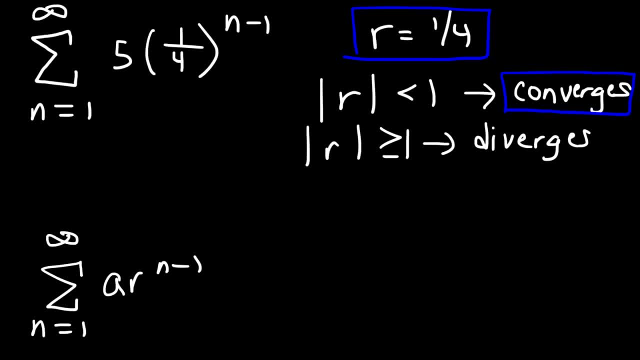 it converges. Now what if we wanted to find the sum of the geometric series as it goes to infinity? If r is less than 1,, then the sum is equal to the first term divided by 1 minus the common ratio. So to find the first term, we need to find the jumbo. 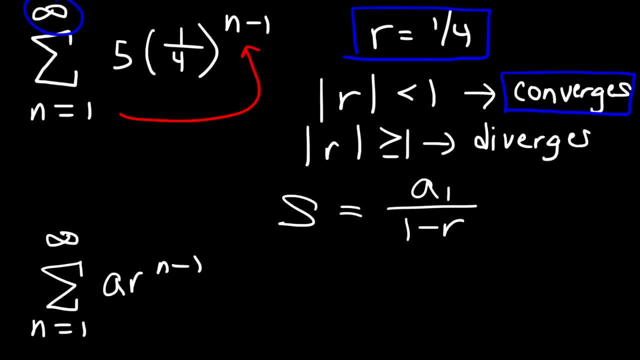 the first term we need to plug in n equal 1.. So that's going to be 5 times 1 over 4 raised to the 1 minus 1, or 0.. 1. fourth, raised to 0, power is 1, and so we get 5.. So 5 is. 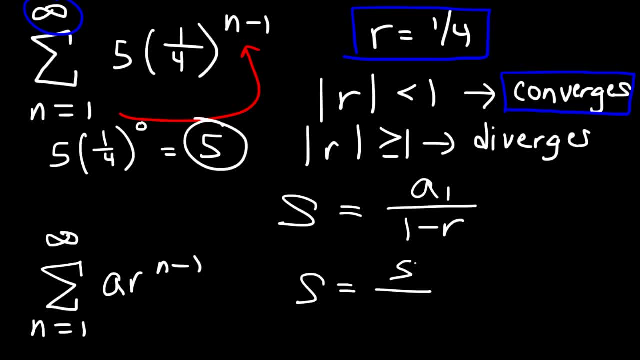 the first term. So it's going to be 5 divided by 1 minus 1 fourth. So we need to multiply the top and the bottom by 4.. 5 times 4 is 20, and then distribute the 4. 4 times 1 is. 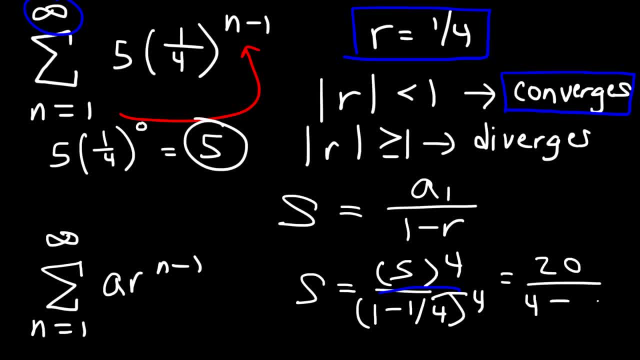 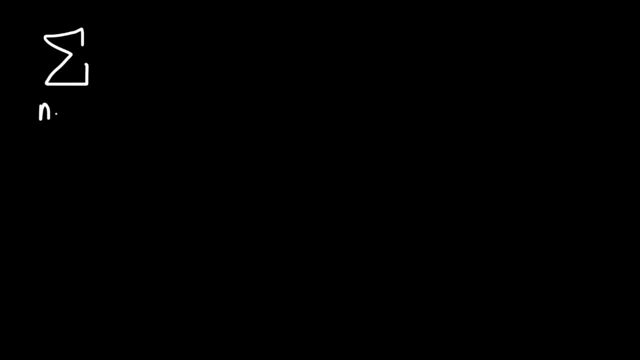 4, and 4 times a fourth is 1.. So the sum is going to be 20 over 3.. So the value of this series is equal to this number. Now let's try this one. So let's say we have. 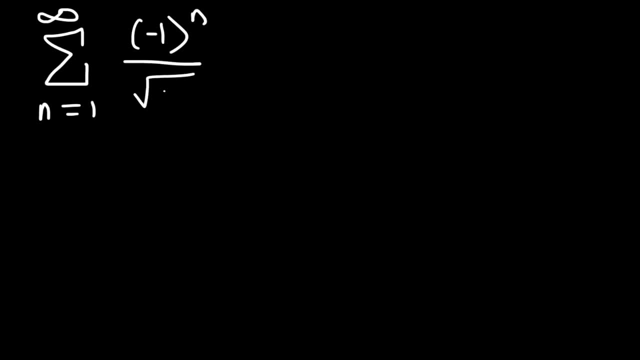 negative 1 raised to the n power divided by the square root of n. So what type of series are we dealing with here? Well, let's write out the first few numbers. So we have 2 terms. When n is 1, it's going to be negative 1 divided by the square root of 1.. And when 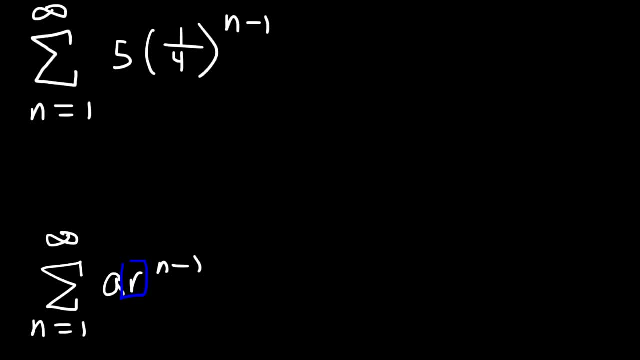 So the common ratio Is one over four. Now recall that If the absolute value of r is less than one, The series converges For geometric series, And if it's greater than or equal to one, The series Diverges. 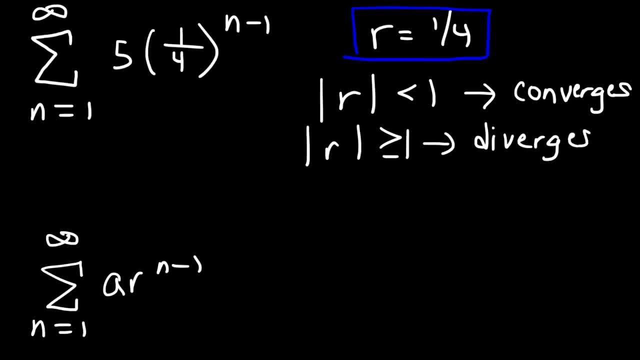 One fourth Is certainly less than one. So we can say that This particular geometric series, It converges. Now what if we wanted to find the sum Of the geometric series As it goes to infinity, If r is less than one? 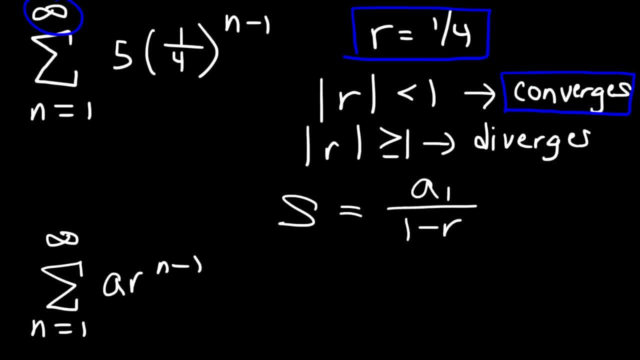 Then the sum Is equal to the first term Divided by one minus the common ratio. So to find the first term We need to plug in n equal one. So that's going to be five Over four Raised to the one minus one or zero. 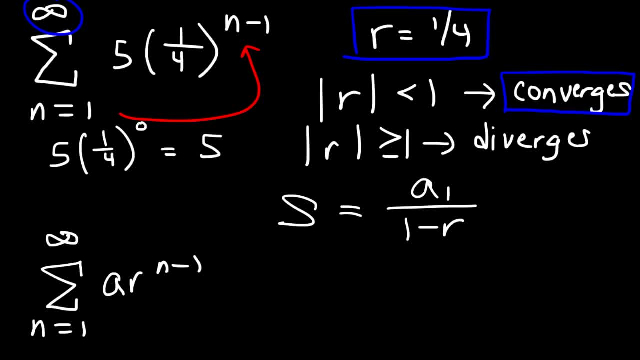 One fourth raised to the zero power is one, And so we get five. So five is the first term, So it's going to be five Divided by one minus one fourth. So we need to multiply the top And the bottom by four. 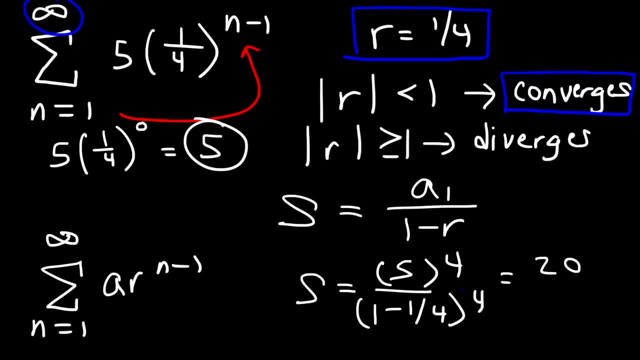 Five times four is twenty. And then distribute the four Four times one is four And four times the fourth is one. So the sum Is going to be twenty over three. So the value of this series Is equal to this number. 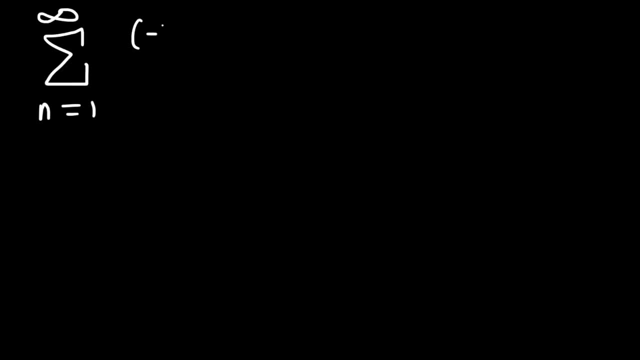 Now let's try this one. So let's say we have negative one Raised to the n power Divided by the square root of n. So what type of series Are we dealing with here? Well, let's write out the first few terms. 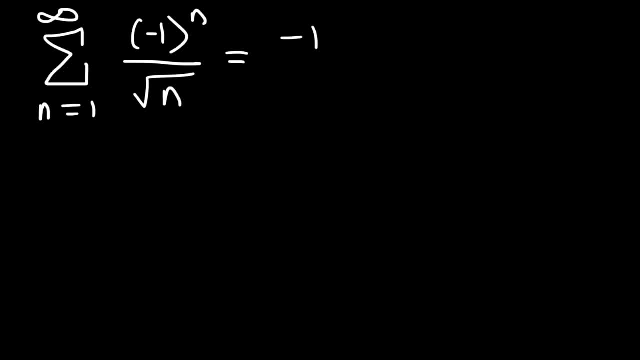 When n is one, It's going to be negative, one Divided by the square root of one. So this two is going to be Negative. one squared is positive, one Divided by the square root of two. And then it's going to be negative, one over the square root of three. 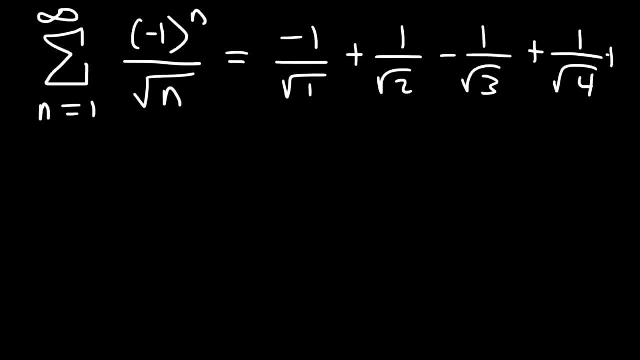 And so forth. So notice that we have an alternating series. So what should we do here? How can we determine If the alternating series Will converge or diverge? Two conditions must be met. First, it has to pass the divergence test. 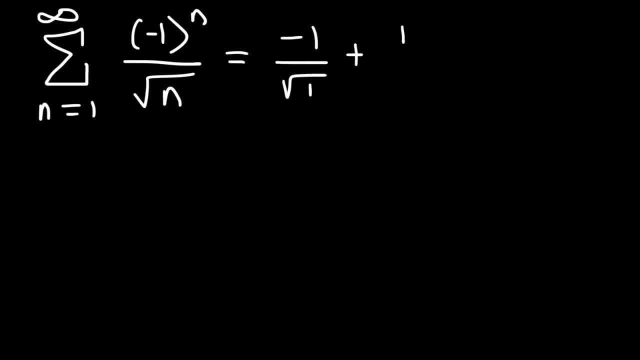 n is 2, it's going to be negative: 1 squared is positive 1 divided by the square root of 2, and then it's going to be negative: 1 over the square root of 3, and so forth. So notice. 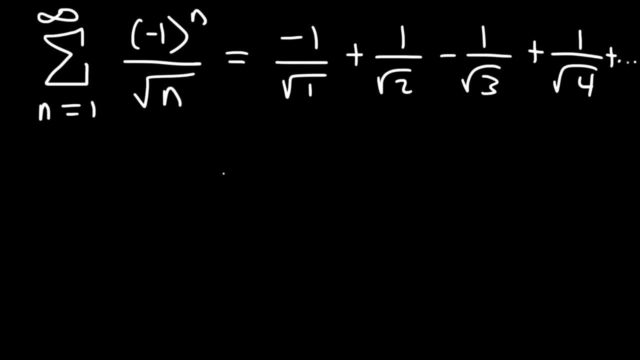 that we have an alternating series. So what should we do here? How can we determine if the alternating series will converge? Two conditions must be met. First, it has to pass the divergence test. So if we take the limit as n approaches infinity of a sub n, Now you need to know what a sub n is in. 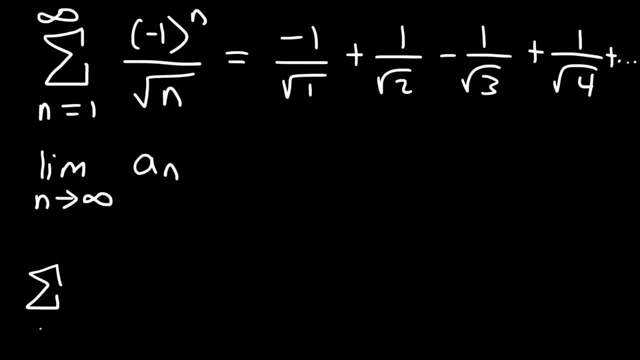 this problem. So for the alternating series it's typically in this form. It's going to be negative: 1 to the n power times a sub n. So a sub n is everything except this. This could be n plus 1 too, by the way. Just keep that in mind. 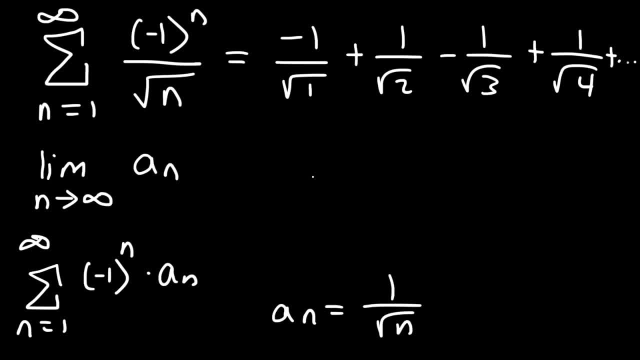 So a sub n is 1 divided by the square root of n. So if we take the limit, as n goes to infinity, of 1 divided by the square root of n, then this is going to go to 0. So it passes the divergence test. Now the second thing that we need to show is that the next term 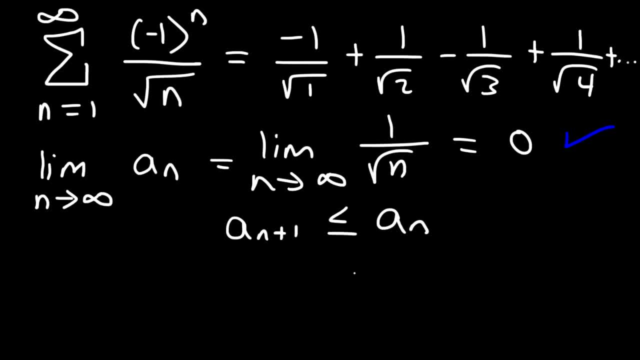 is less than or equal to the previous term. So the previous term being 1 divided by the square root of n of n, and the next term is going to be 1 over the square root of n plus 1.. So the denominator of 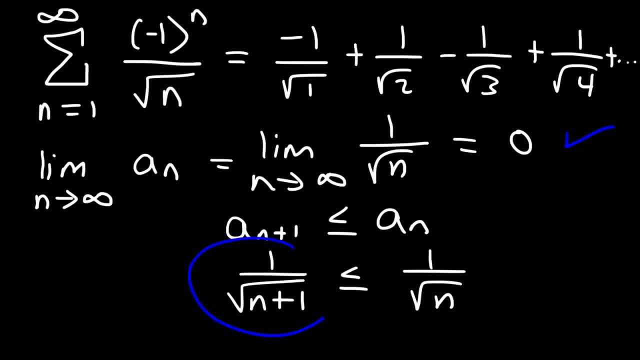 this fraction is bigger, which means the value of this fraction is smaller. So this is a true statement. Therefore, we could say that this series, according to the alternating series test, is convergent. Now, is it absolutely convergent or is it conditionally convergent? What would you say? 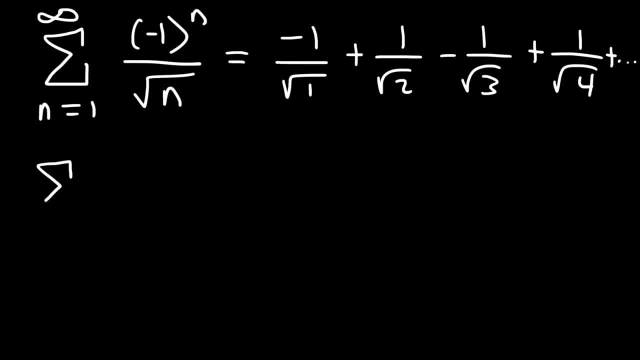 So let's analyze the convergence of the absolute value of the series. So if we take the absolute value of negative 1 to the n divided by the square root of n, the negative 1 to the n, it produces the alternating signs 1, negative 1, negative 1, 1, and so forth. 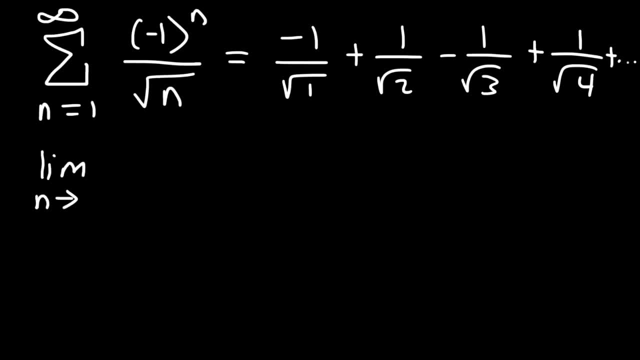 So if we take the limit As n approaches infinity, Of a sub n, Now you need to know what a sub n is In this problem. So for the alternating series It's typically in this form: It's going to be negative one to the n power. 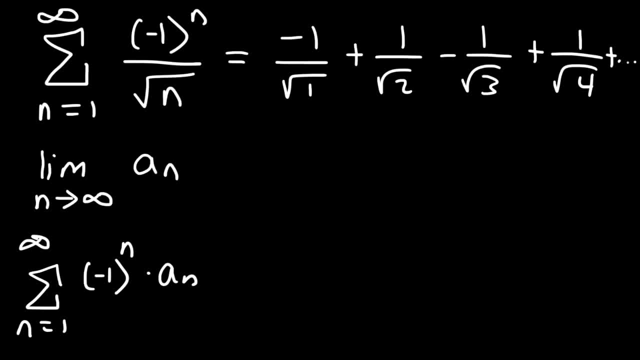 Times a sub n. So a sub n is everything Except this. This could be n plus one too, by the way. Just keep that in mind. So a sub n is one Divided by the square root of n. So if we take the limit, 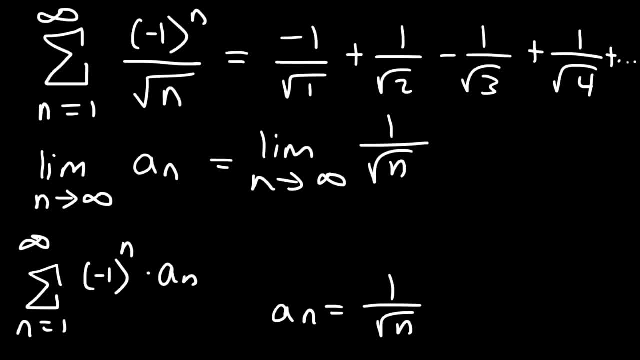 As n goes to infinity Of one divided by the square root of n, Then this is going to go to zero, So it passes the divergence test. Now the second thing that we need to show Is that The next term Is less than or equal to the previous term. 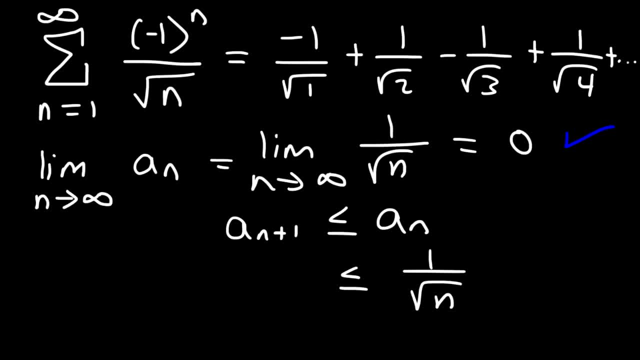 So, the previous term being One divided by the square root of n, And the next term is going to be one over the square root of n plus one, So The denominator of this fraction Is bigger, Which means the value of this fraction is smaller. 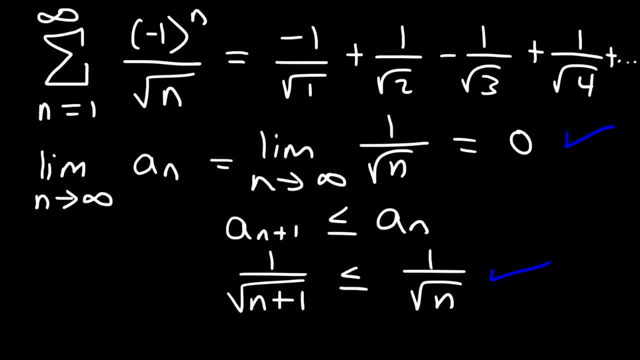 So this is a true statement. Therefore, we could say That this series, According to the alternating series test, Is convergent. Now, Is it absolutely convergent, Or is it conditionally convergent? What would you say? So let's analyze. 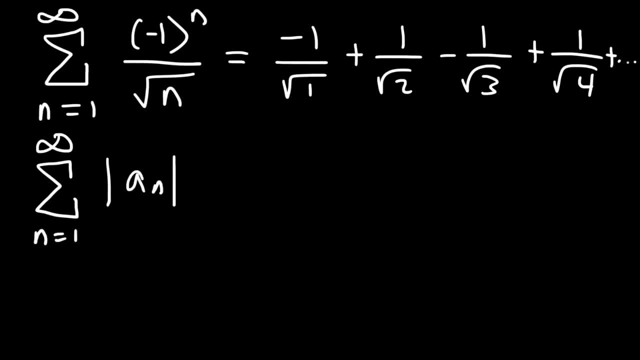 The convergence Of the absolute value of the series. So if we take the absolute value Of negative one to the n Divided by the square root of n, The negative one to the n, It produces the alternating signs: One negative one. 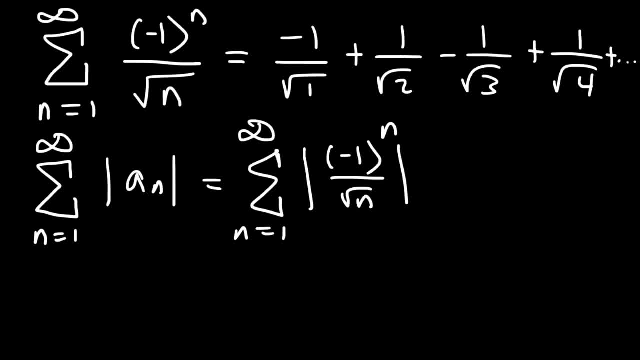 Negative one, one And so forth. So if you take the absolute value of that, The negative one and the one, So then We're going to get this series. So it's going to be one Divided by the square root of n. 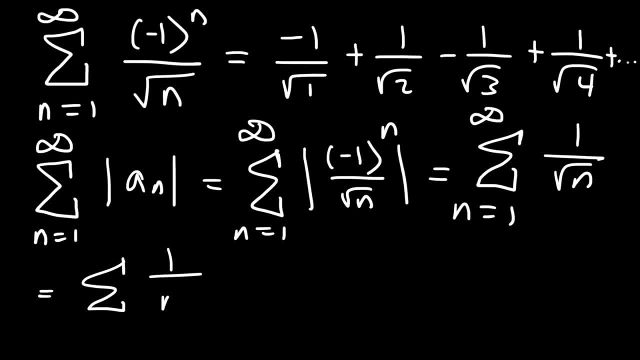 And the square root of n Is n To the one half. So what type of series Do we have? Notice that we have the p series. It's in the form one over n to the p, So we can clearly See that p. 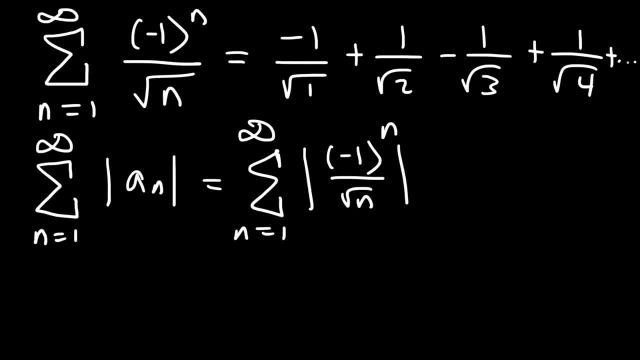 So if you take the absolute value of that, the negative 1 and the 1 will just be 1.. So then we're going to get this series. So it's going to be 1 divided by the square root of n and the square 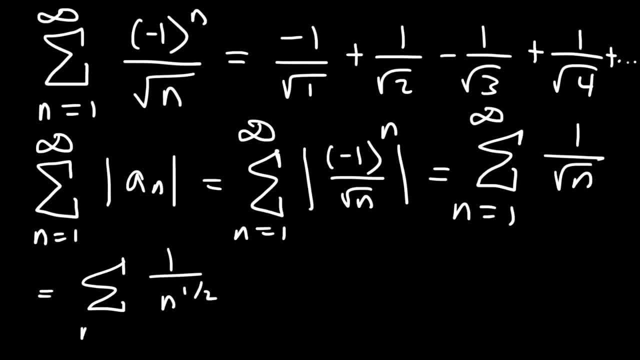 root of n is n to the 1 half. So what type of series do we have? Notice that we have the p series. It's in the form 1 over n to the p, So we can clearly see that p is 1 half. So if p is 1 half, will the series converge or will it? 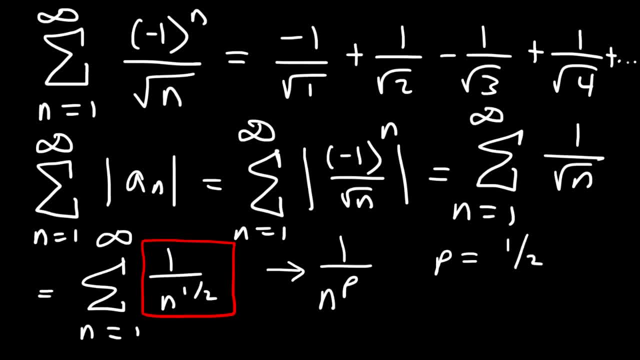 diverge. In order for the series to converge, p has to be greater than 1.. But because p is less than or equal to 1, this series is divergent. So because the original series converges but the absolute value of the series diverges, then we say that the original series is conditionally. 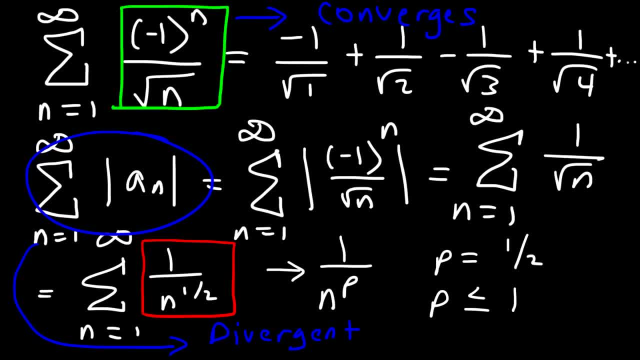 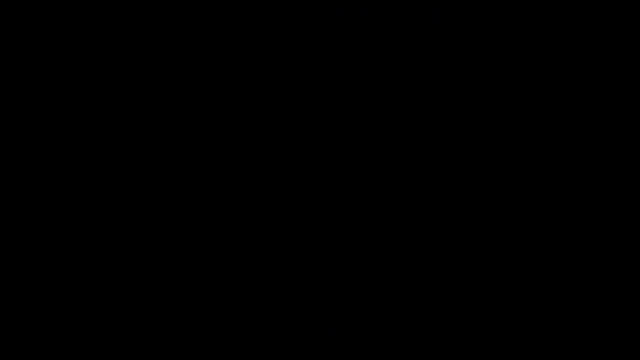 convergent. In order for it to be absolutely convergent, the original series must converge and the absolute value of the series must converge as well. Now let's move on to our next example. So let's say: this is 1 over n times n plus. 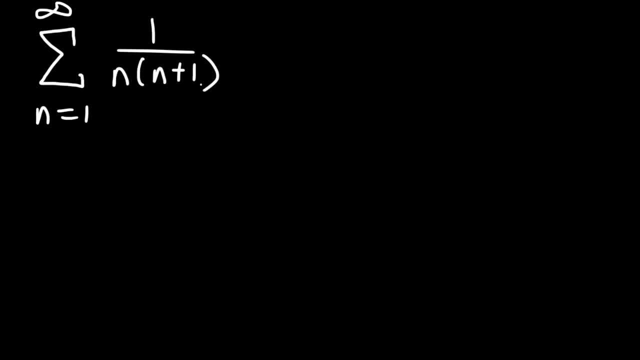 n, Will the series converge or diverge? Well, let's check with divergence tests. So what happens when n goes to infinity? So we can rewrite this as the limit, as n goes to infinity, of 1 over n squared plus n. And if we multiply the top and the bottom by 1 over n squared, 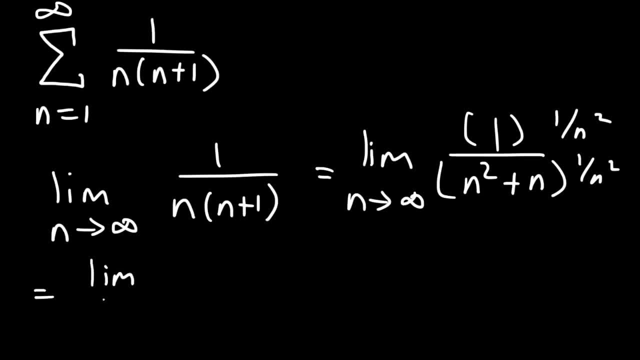 we're going to get the limit as n goes to infinity: 1 over n squared divided by 1 plus 1 over n, So 1 over n squared, that's going to go to 0.. And 1 over n is going to go to 0.. 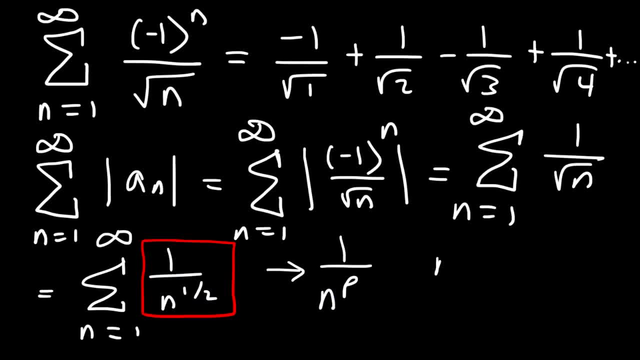 Is one half. So if p is one half, Will the series converge Or will it diverge? In order for the series to converge, P has to be greater than one, But because p is Less than or equal to one, This series 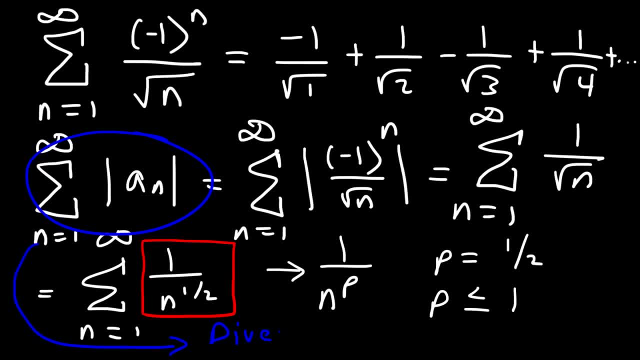 Is divergent. So because the original Series Converges But the absolute value of the series Diverges, Then we say that The original series Is conditionally convergent In order for it to be absolutely convergent. 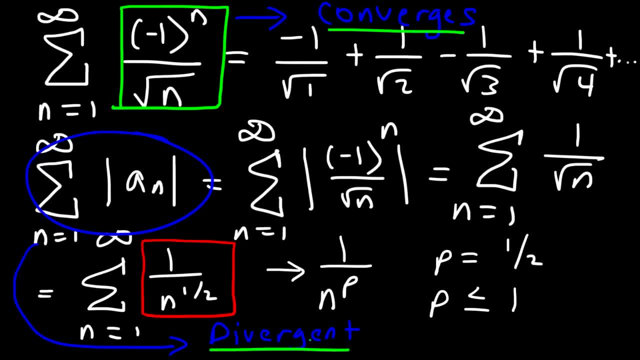 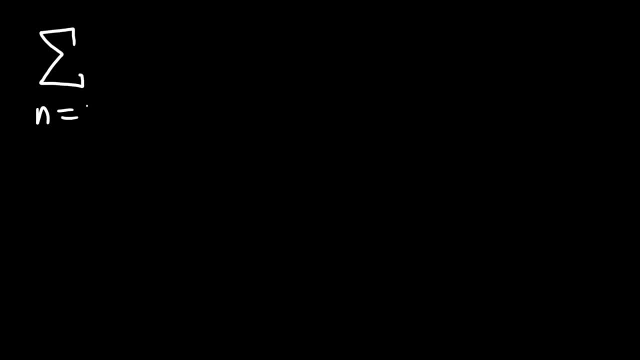 The original series must converge And the absolute value of the series Must converge as well. Now let's move on To our next example. So let's say this is one Over n Times n plus one. Will the series converge? 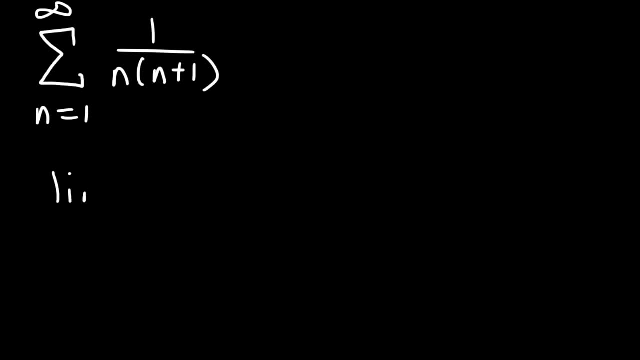 Or diverge. Well, let's check with divergence tests. So what happens When n goes to infinity? So we can rewrite this As the limit, As n goes to infinity, Of one over n squared plus n, And if we multiply. 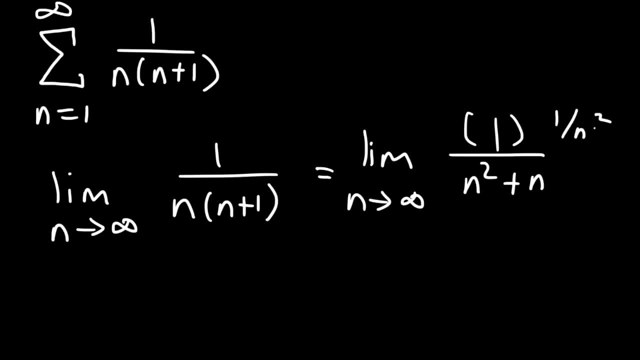 The top and the bottom by One over n squared, We're going to get the limit Of infinity: One over n squared Divided by one plus one over n, So one over n squared. That's going to go to zero. 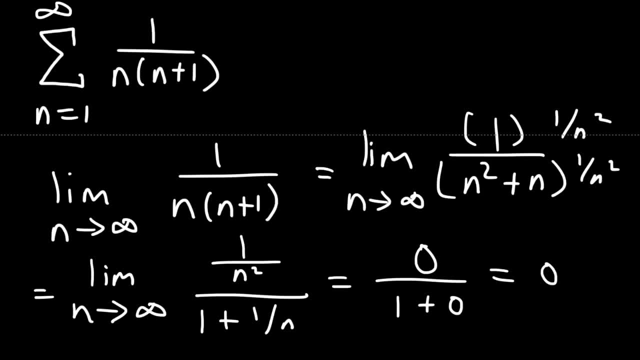 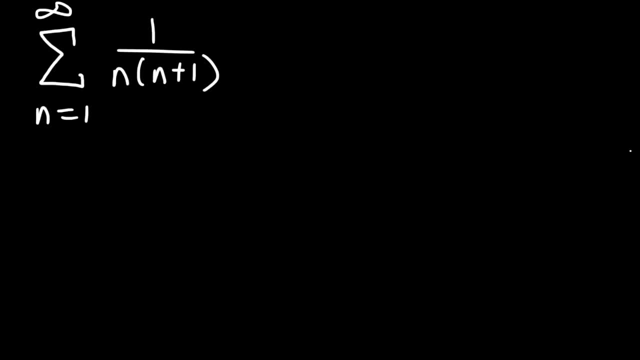 And one over n is going to go to zero, So it equals zero. So the divergence test is inconclusive. So what do you think we need to do here? This problem Can be solved If we recognize it to be a Telescope and series problem. 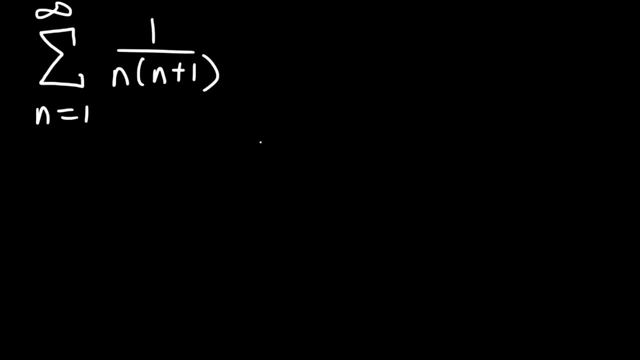 So first Let's set one over n Times n plus one To a over n Plus B over N plus one, And let's multiply both sides By n times n plus one, So these will cancel And that's going to give us one. 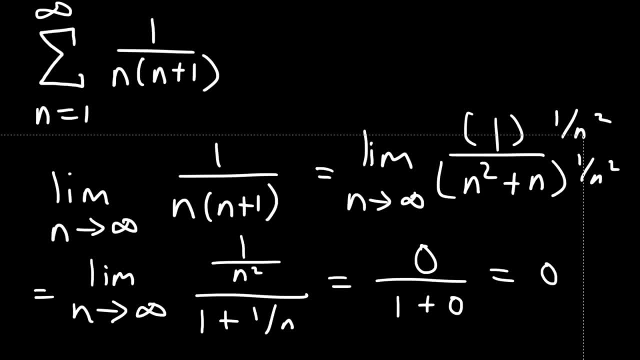 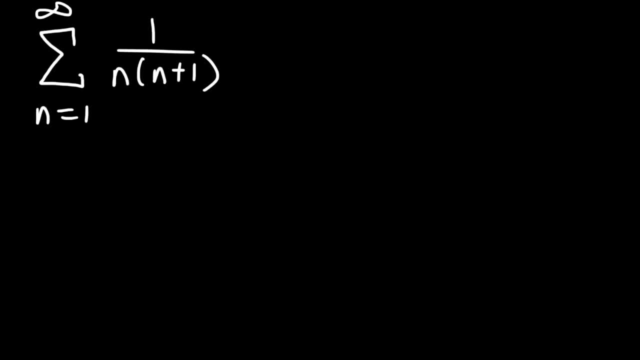 So it equals 0.. So the divergence test is inconclusive. So what do you think we need to do here? This problem can be solved if we recognize it to be a telescope and series problem. So first we need to use partial fraction decomposition. So let's set 1 over n times. 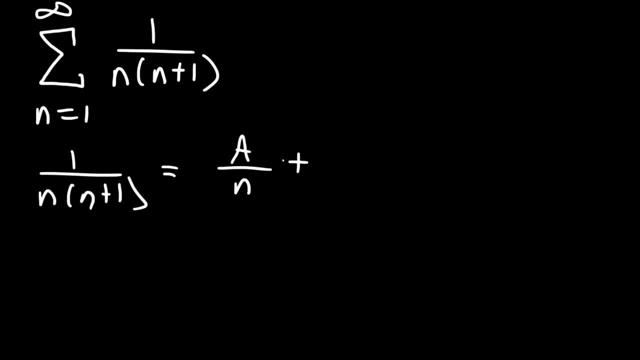 n plus 1 to a over n plus b over n plus 1.. And let's multiply both sides by n times n plus 1.. So these will cancel And that's going to give us 1.. And then n will cancel leaving. 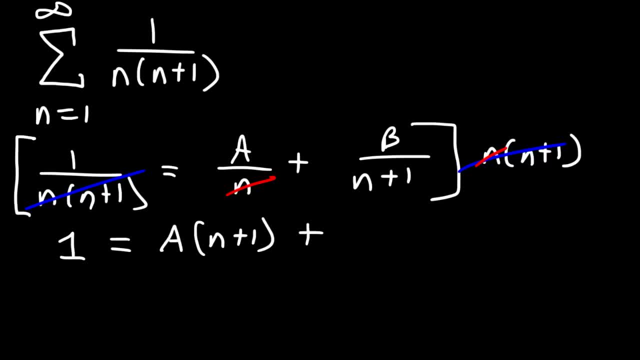 behind a times 1.. n plus 1 and then n plus 1 will cancel, leaving behind b times n. now let's say: if n is equal to 0, that means b and disappears. so 1 is equal to a times 0 plus 1, which means a is equal to 1. now, if n is equal to negative 1, this will 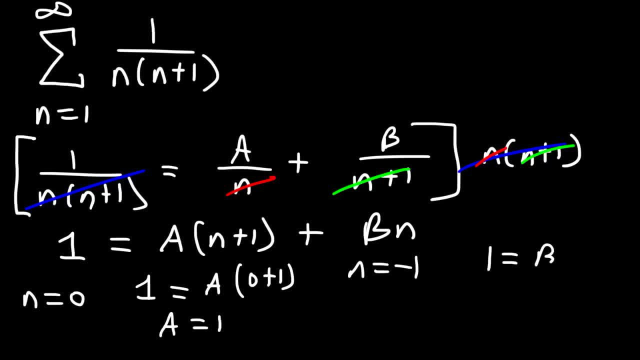 disappear, that will be 0. so 1 is equal to B times negative 1, which means B is negative 1. so we can rewrite this expression like this: so instead of 1 over n times n plus 1, we can replace a with 1, so it's going to be 1 over n and. 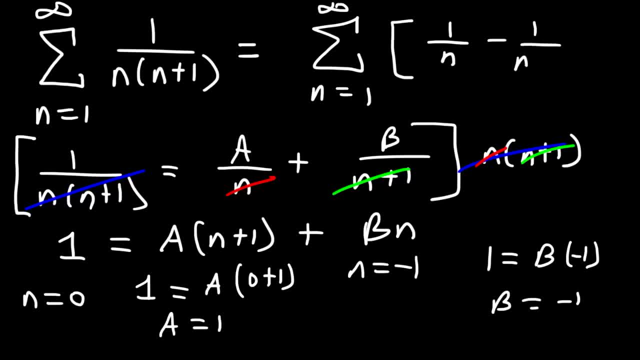 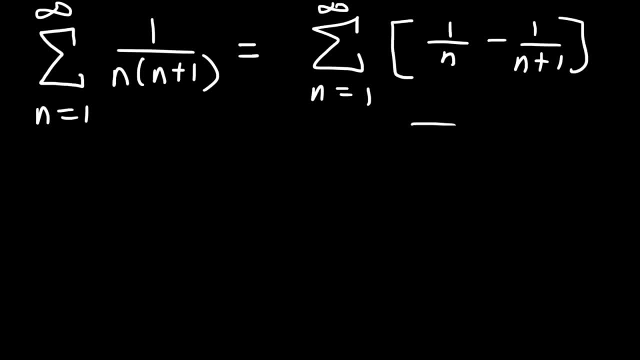 then we can replace B with negative 1, so it's negative 1 over n plus 1. so now you can see that we have a telescope in series, so let's write out a few terms. okay, so we have a telescope in series, so let's write out a few terms. 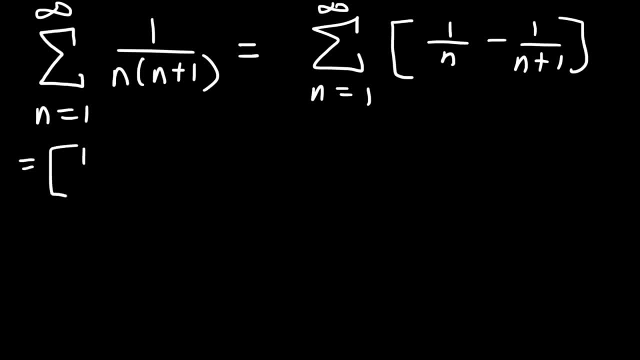 okay. so we have a telescope in series, so let's write out a few terms. so when n is 1, this is going to be 1 over 1. so when n is 1, this is going to be 1 over 1. so when n is 1, this is going to be 1 over 1 minus 1 over 2. so this is the first. 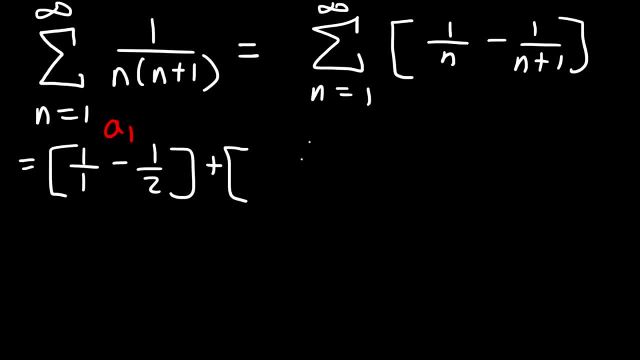 minus 1 over 2. so this is the first minus 1 over 2. so this is the first term, and then the second term when n is 2 is term, and then the second term when n is 2 is term, and then the second term when n is 2 is going to be plus 1 over 2, minus 1 over. 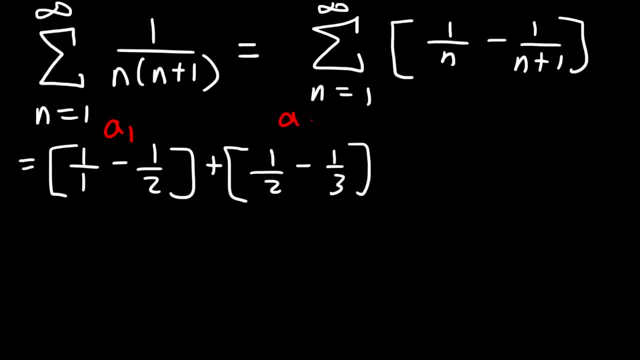 going to be plus 1 over 2 minus 1 over. going to be plus 1 over 2 minus 1 over 3, so that's a sub 2. and then when n is 3, 3, so that's a sub 2. and then when n is 3, 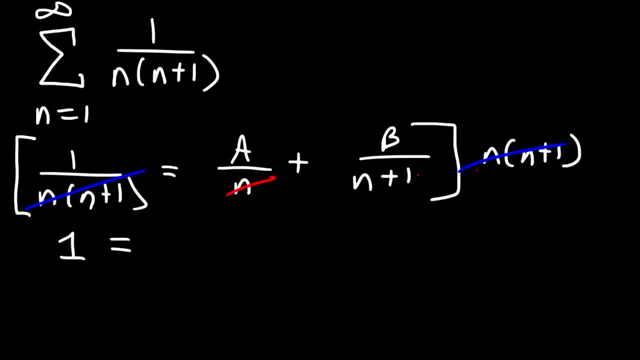 And then n Will cancel Leaving behind A times n plus one, And that's going to give us. And then n plus one will cancel Leaving behind B times n. Now let's say if N is equal to zero, 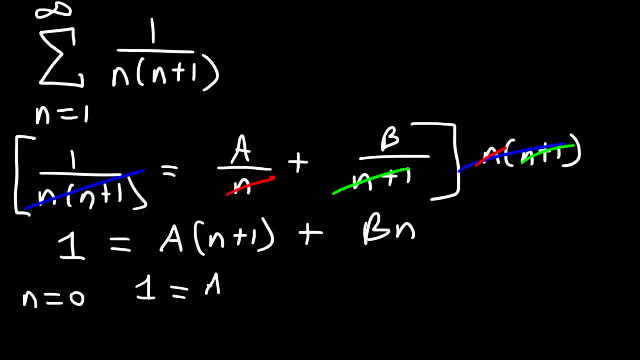 That means bn disappears. So one is equal to a Times zero plus one, Which means a is equal to one. Now, if n is equal to negative one, This will disappear. That will be zero. So one is equal to b times negative one. 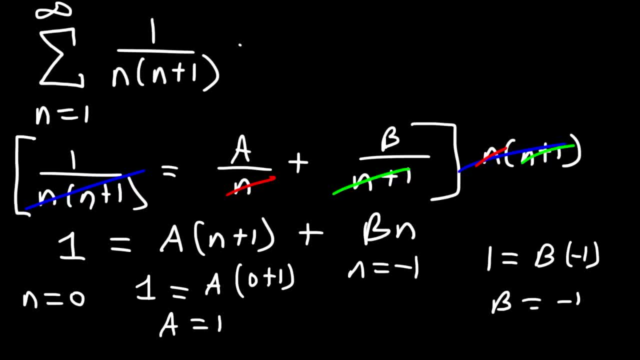 Which means b Is negative one. So we can rewrite this expression Like this: So instead of one over n Times n plus one. We can replace a with one, So it's going to be One over n, And then we can replace b with negative one. 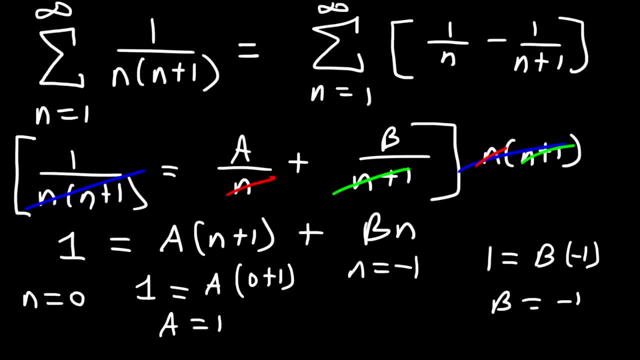 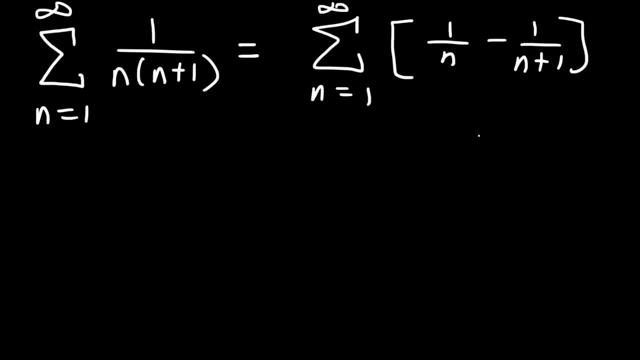 So it's negative. one over n plus one. So now you can see that We have a telescope in series. So let's write out a few terms. So when n is one, This is going to be One over one, Minus one over two. 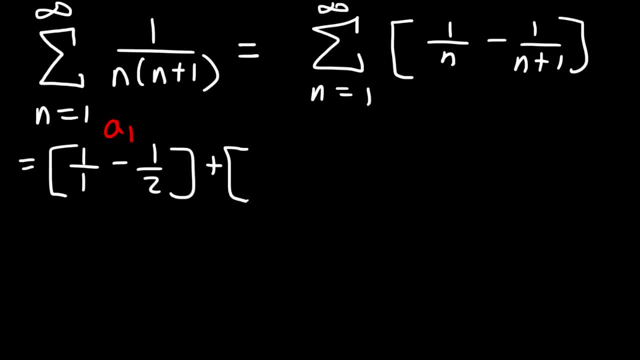 So this is the first term, And then the second term, When n is two Is going to be, plus One over two, minus one over three, So that's a sub two, And then when n is three Is going to be. 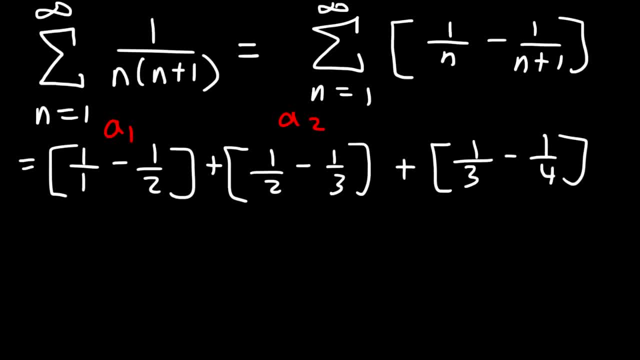 One over three minus one over four. So that's the third term. Now Let's write The a sub n minus one term. So if we replace this with n minus one, It's just going to be one over n minus one. 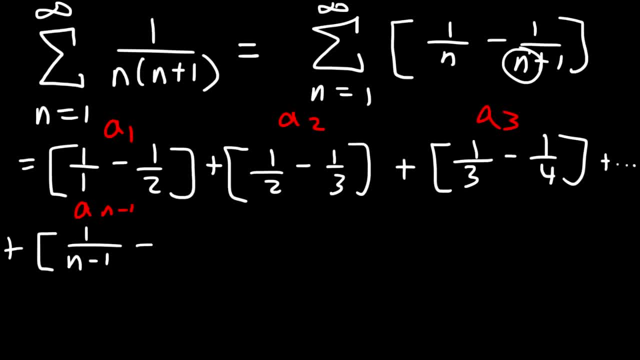 And then if we replace this with n minus one Plus one, It's just going to be one over n. Now, the last term, That is the a sub N term. It's just going to be what you see here. So one over n. 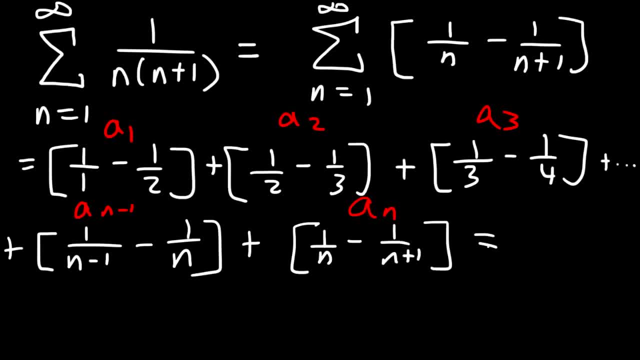 Minus one over n plus one. So all of this Is the sum Of the first n terms. So this is the partial sum. Now let's see what we can cancel. So we can cancel Negative one half and one half. 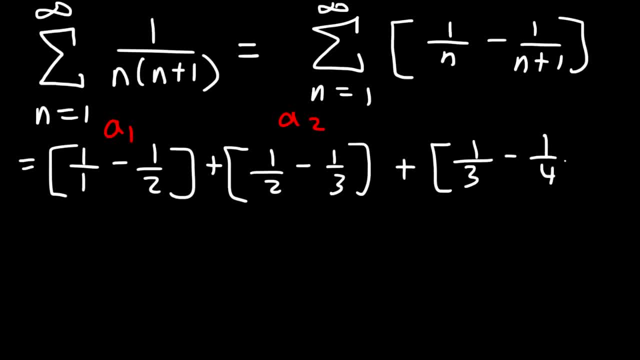 3, so that's a sub 2. and then when n is 3, is going to be 1 over 3 minus 1 over 4, so is going to be 1 over 3 minus 1 over 4, so that's a third term. 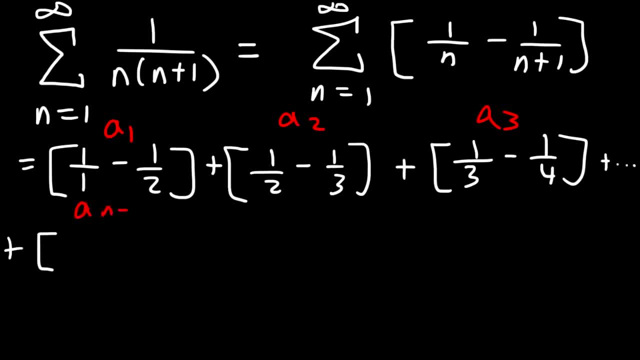 now let's write the a sub n minus 1. now let's write the a sub n minus 1. now let's write the a sub n minus 1 term. so if we replace this with n minus 1 term, so if we replace this with n minus 1, 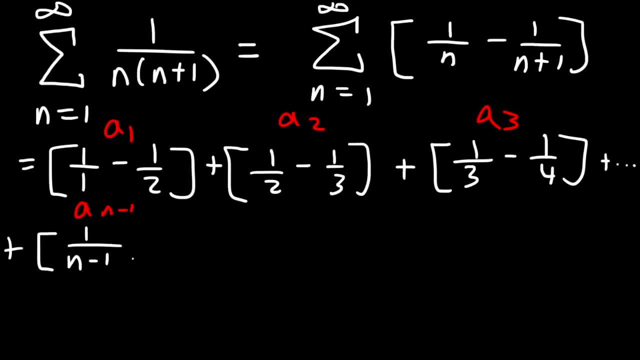 term. so if we replace this with n minus 1, it's just going to be 1 over n minus 1, it's just going to be 1 over n minus 1, it's just going to be 1 over n minus 1. and then if we replace this with n minus, 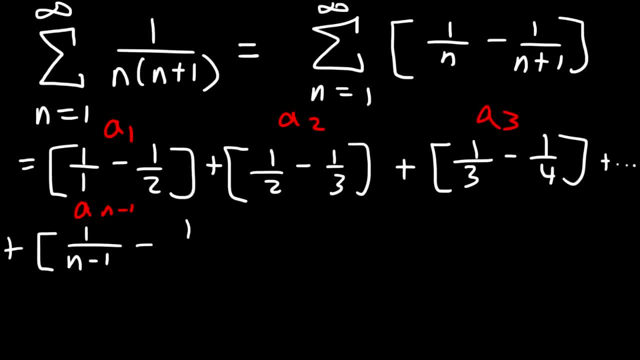 and then if we replace this with n minus, and then if we replace this with n minus, 1 plus 1, it's just going to be 1 over n. 1 plus 1: it's just going to be 1 over n. 1 plus 1: it's just going to be 1 over n. now the last turn, that is, the a sub n. 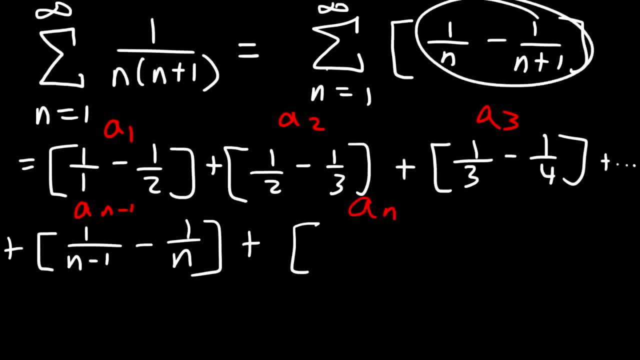 now the last turn, that is the a sub n. now the last turn. that is the a sub n. term: it's just going to be what you see. term: it's just going to be what you see. term: it's just going to be what you see here. so, 1 over n minus 1 over n plus 1. 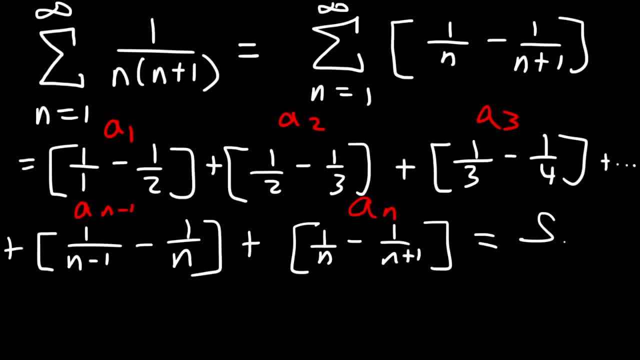 here. so 1 over n minus 1 over n plus 1 here. so 1 over n minus 1 over n plus 1. so all of this is the sum of the first. so all of this is the sum of the first. so all of this is the sum of the first n terms. so this is the partial sum. now, 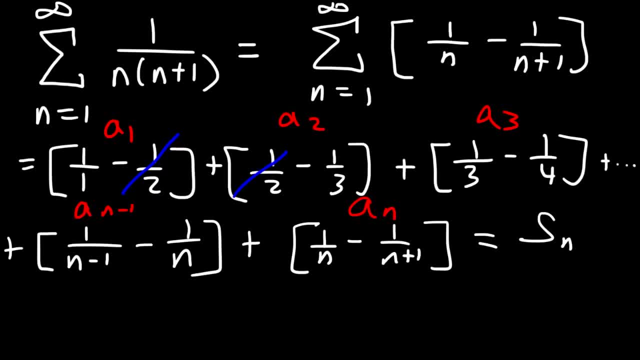 n terms. so this is the partial sum now n terms. so this is the partial sum now let's see what we can cancel, so we can. let's see what we can cancel, so we can. let's see what we can cancel. so we can cancel negative 1 half and 1 half. 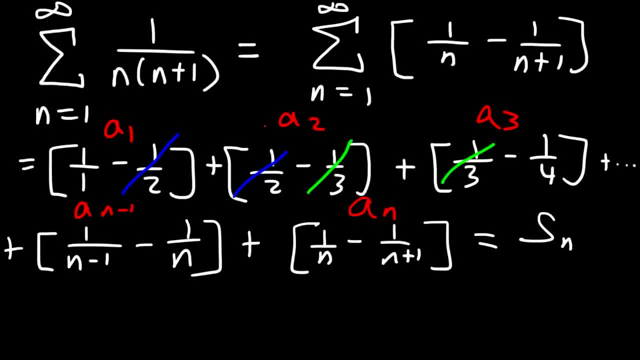 cancel negative 1 half and 1 half. cancel negative 1 half and 1 half. negative 1 third and 1 third and then negative 1. fourth will cancel with 1 negative. 1. fourth will cancel with 1 negative 1. fourth will cancel with 1. fourth, which is somewhere in the middle. 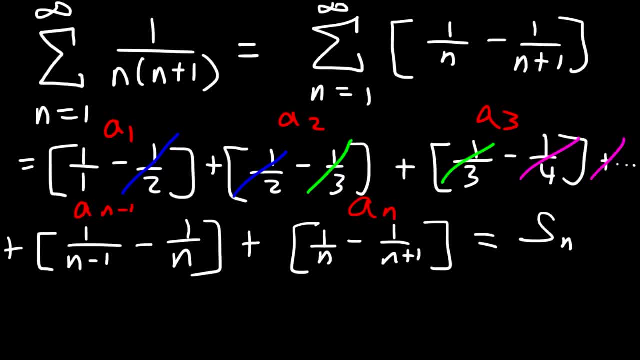 fourth, which is somewhere in the middle. fourth, which is somewhere in the middle of the sequence, and then we can cancel negative 1 over n plus 1 over n- now 1 negative 1 over n plus 1 over n- now 1 negative 1 over n plus 1 over n- now 1 over n minus 1 will cancel with another. 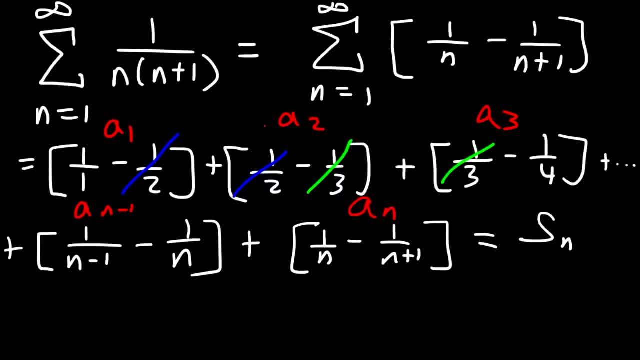 Negative one third and one third, And then Negative one fourth will cancel with one fourth Which is somewhere in the middle of the sequence, And then we can cancel Negative one over n plus one over n. Now N minus one will cancel with. 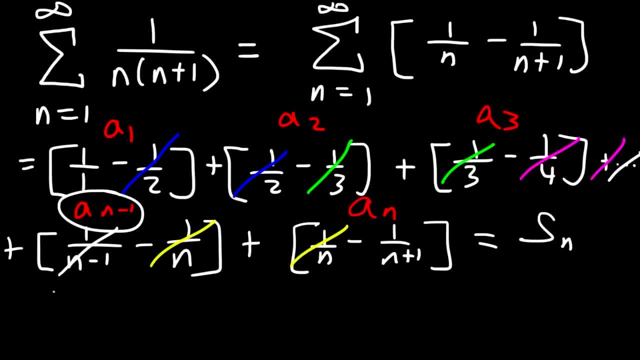 Another one over n minus one If you write out the a sub n minus Two term, So the only thing that's going to remain Is one And negative one over N plus one. So this allows us to write the general formula. 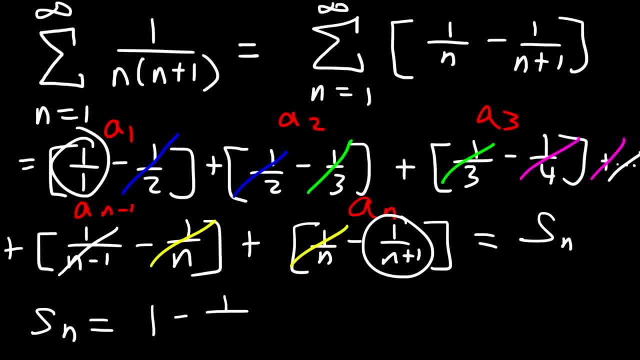 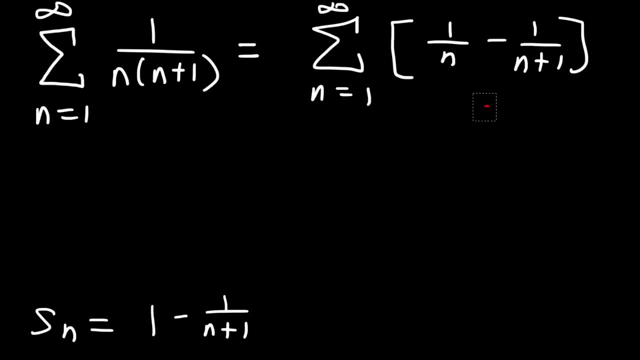 For the partial sum, So it's one minus one over n plus one. Let's get rid of this too. So now We'll need to calculate The sum of the sequence. So let's take the limit As n approaches infinity. 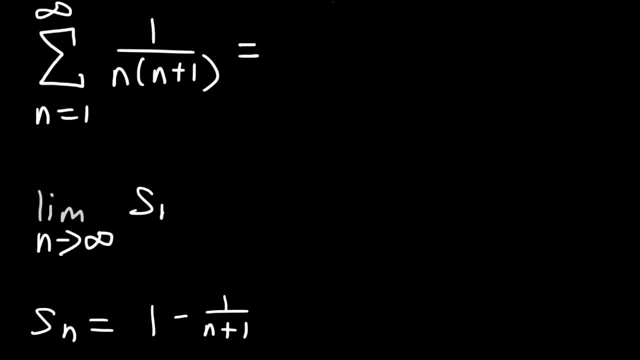 Of the partial sum formula S sub n. So that's one minus One over n plus one. So that's one minus One over n plus one. So this is equal to one Minus the limit, As n goes to infinity. 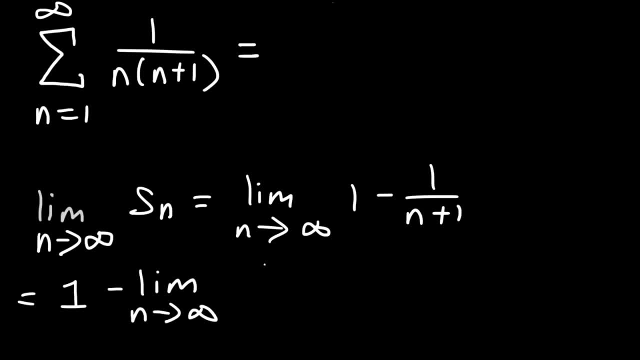 Of one over n plus one, And this is going to go to zero. So it's one minus zero, Which is one. So therefore, The sum of this series Is equal to one, And because It's equal to a finite positive number, 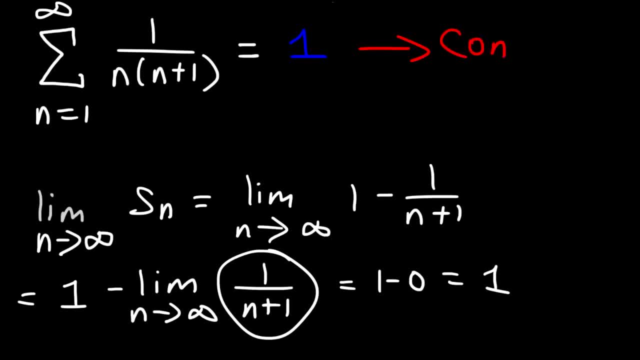 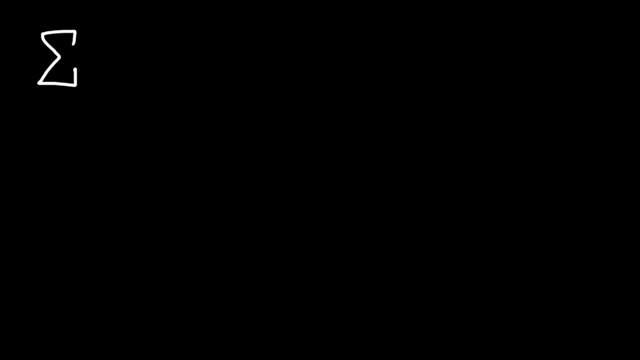 And not infinity. The original series we say Converges. Here's another one That you could try. Let's say, If it's one over N squared plus four. So what can we do For this problem? How can we determine? 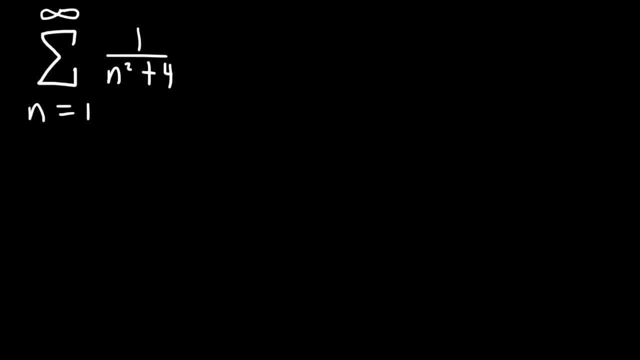 If the series is going to converge Or diverge, What test would you recommend? The best thing to do Is to compare it, To use the direct comparison test. Notice that If we take away the four, This becomes a p series problem. 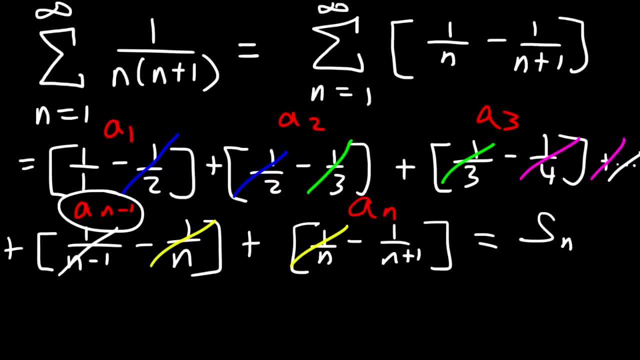 over n minus 1 will cancel with another over n minus 1. will cancel with another 1 over n minus 1 if you write out the a 1 over n minus 1, if you write out the a 1 over n minus 1, if you write out the a sub n minus 2 term. so the only thing. 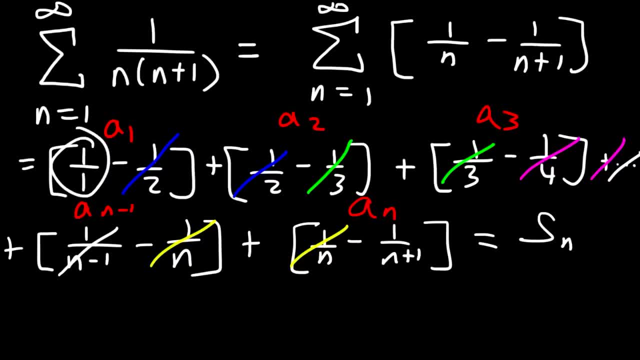 sub n minus 2 term. so the only thing sub n minus 2 term. so the only thing that's going to remain is 1, and that's going to remain is 1, and that's going to remain is 1 and negative 1 over n plus 1, so this allows. 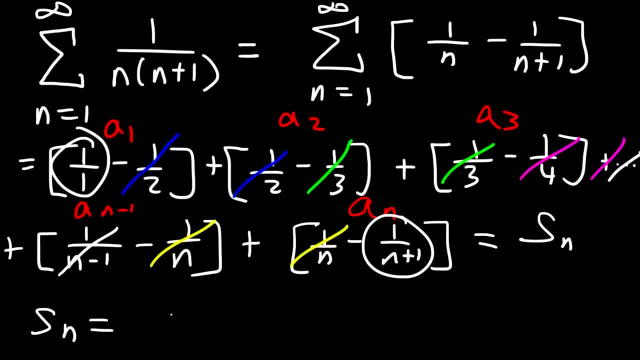 negative 1 over n plus 1. so this allows negative 1 over n plus 1. so this allows us to write the general formula for the us, to write the general formula for the us, to write the general formula for the partial sum. so it's a 1 minus 1 over n. 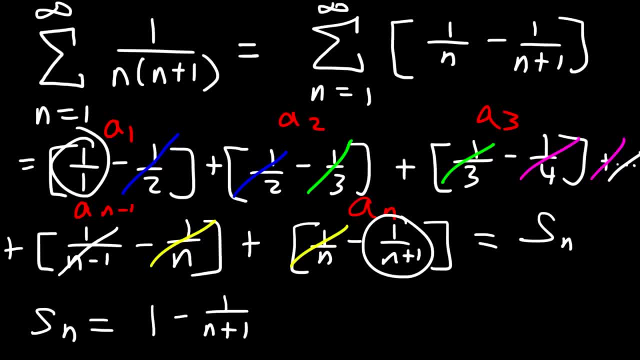 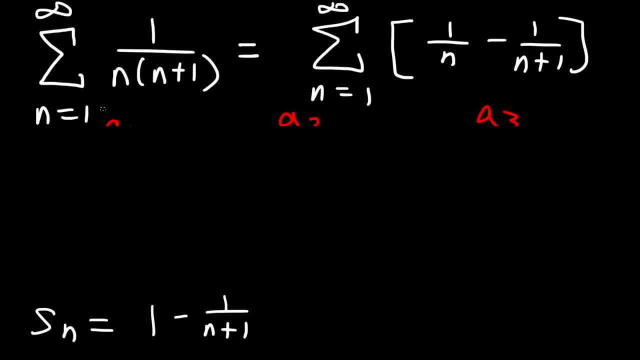 partial sum, so it's a 1 minus 1 over n partial sum. so it's a 1 minus 1 over n plus 1. let's get rid of this too. so now, so now. so now we need to calculate the sum of the. we need to calculate the sum of the. 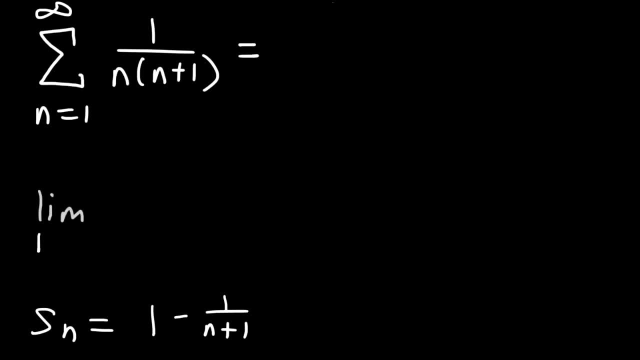 we need to calculate the sum of the sequence. so let's take the limit as n sequence. so let's take the limit as n sequence. so let's take the limit as n approaches infinity of the partial sum, approaches infinity of the partial sum, approaches infinity of the partial sum formula s sub n. so that's 1 minus 1 over. 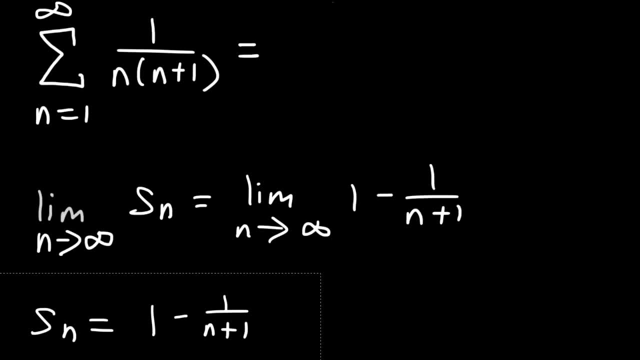 formula s sub n, so that's 1 minus 1 over formula s sub n, so that's 1 minus 1 over n plus 1, so this is equal to 1 minus the n plus 1, so this is equal to 1 minus the. 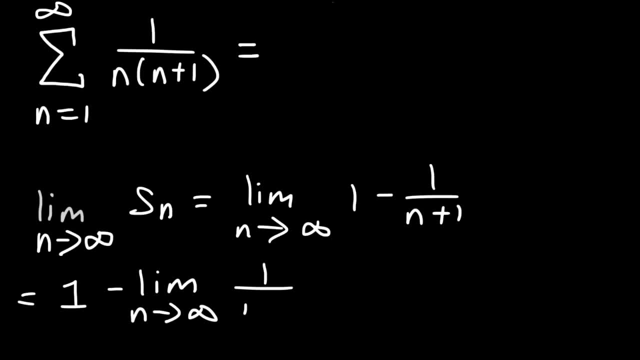 n plus 1, so this is equal to 1 minus the limit, as n goes to infinity of 1 over n limit, as n goes to infinity of 1 over n limit, as n goes to infinity of 1 over n plus 1, and this is going to go to 0. so plus 1, and this is going to go to 0. so plus 1, and this is going to go to 0. so it's 1 minus 0, which is 1. so therefore, it's 1 minus 0, which is 1, so therefore. 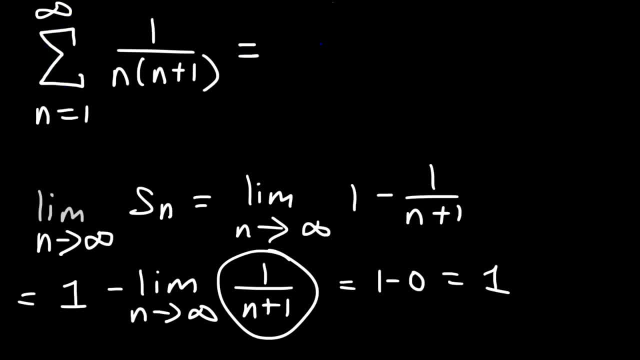 it's 1 minus 0, which is 1, so therefore, the sum of this series is equal to 1 and the sum of this series is equal to 1, and the sum of this series is equal to 1 and because it's equal to a finite positive. 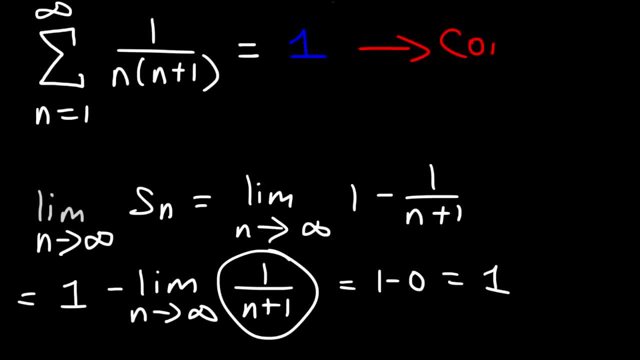 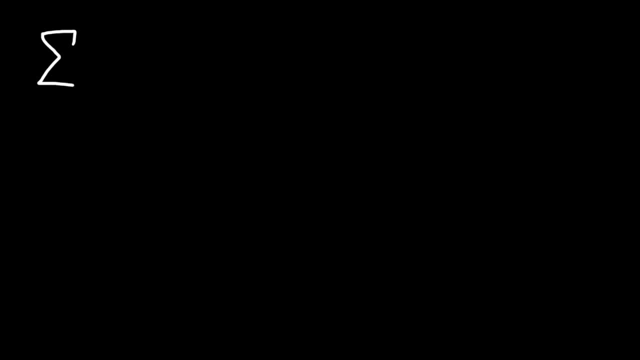 because it's equal to a finite positive, because it's equal to a finite positive number and not infinity. the original number and not infinity. the original number and not infinity. the original series we say converges. here's another one that you could try. here's another one that you could try. 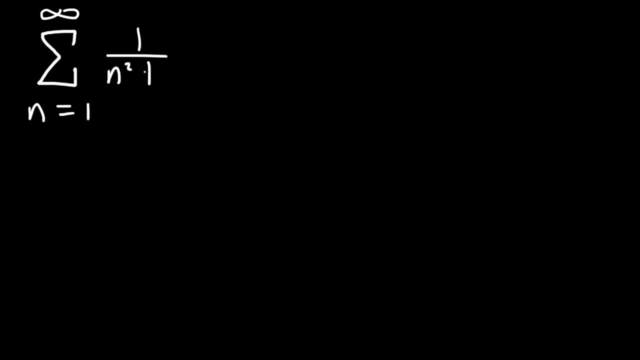 here's another one that you could try. let's say: if it's 1 over n squared plus, let's say: if it's 1 over n squared plus, let's say: if it's 1 over n squared plus 4, 4, 4. so 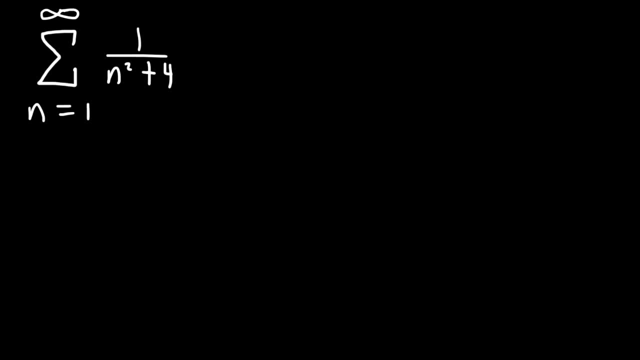 so. so what can we do for this problem? how? what can we do for this problem? how? what can we do for this problem? how can we determine if the series is going to? can we determine if the series is going to? can we determine if the series is going to converge or diverge? what test would 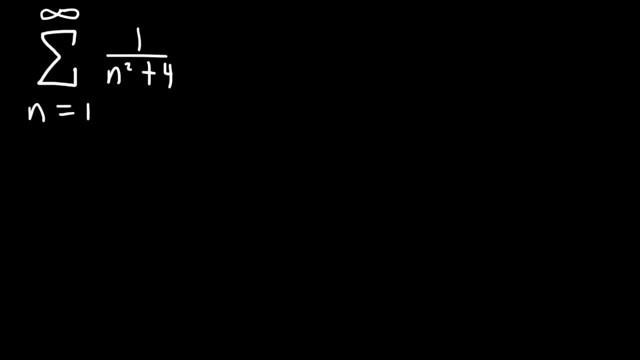 converge or diverge? what test would converge or diverge? what test would you recommend? the best thing to do is to you recommend. the best thing to do is to you recommend. the best thing to do is to compare it, to use the direct comparison. compare it to use the direct comparison. 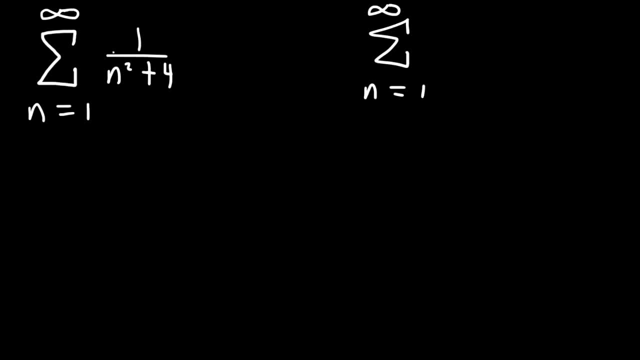 compare it to use the direct comparison test, notice that if we take away the 4 test, notice that if we take away the 4 test, notice that if we take away the 4, this becomes a p-series problem. now this becomes a p-series problem now. 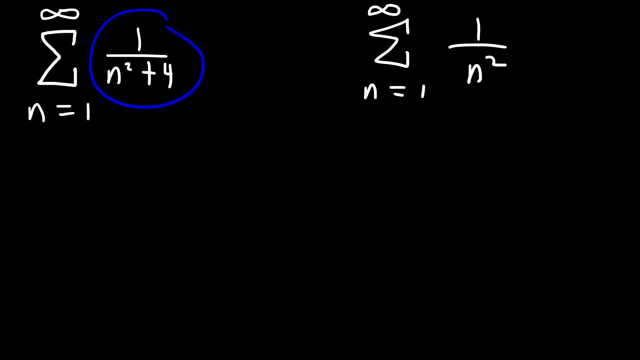 this becomes a p-series problem now. which sequence is bigger than 1 over n? which sequence is bigger than 1 over n? which sequence is bigger than 1 over n squared plus 4 or 1 over n squared, 1 over squared plus 4 or 1 over n squared 1 over. 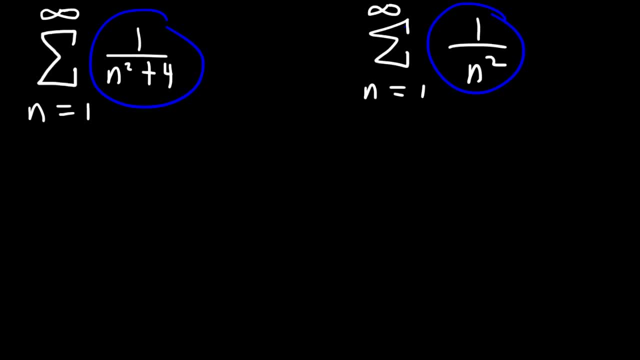 squared plus 4 or 1 over n squared. 1 over n squared is greater than 1 over n. n squared is greater than 1 over n. n squared is greater than 1 over n squared plus 4. if you plug in 1, this: 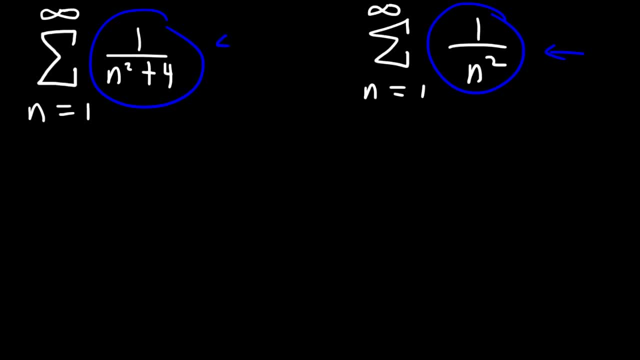 squared plus 4. if you plug in 1, this squared plus 4. if you plug in 1, this would be 1 and this is going to be 1. over would be 1 and this is going to be 1 over would be 1 and this is going to be 1 over 5. so this is always going to be. 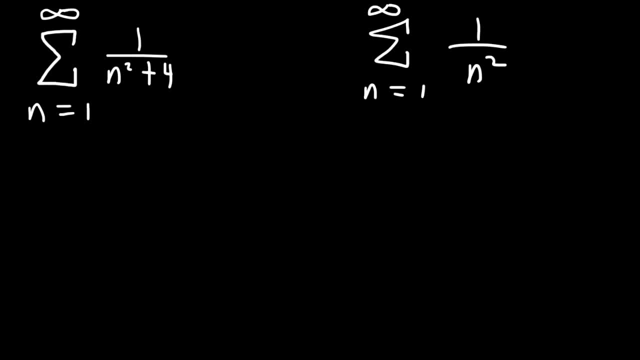 5, so this is always going to be 5, so this is always going to be bigger for all n. so therefore, we could say: bigger for all n. so therefore, we could say bigger for all n. so therefore, we could say: this is our a sub n term and this is: 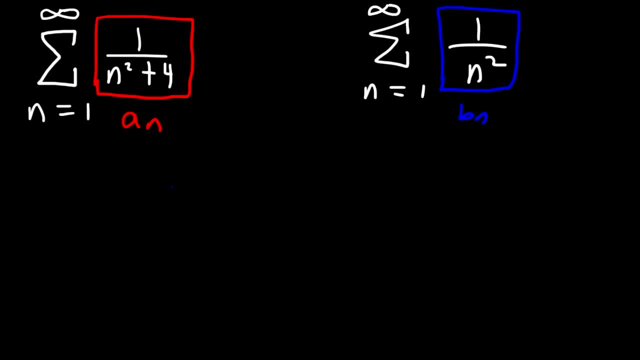 this is our a sub n term, and this is our a sub n term, and this is our b sub n term. so this, our b sub n term, and this is our b sub n term. so this, our b sub n term, and this is our b sub n term. so this series is bigger than this one. now, 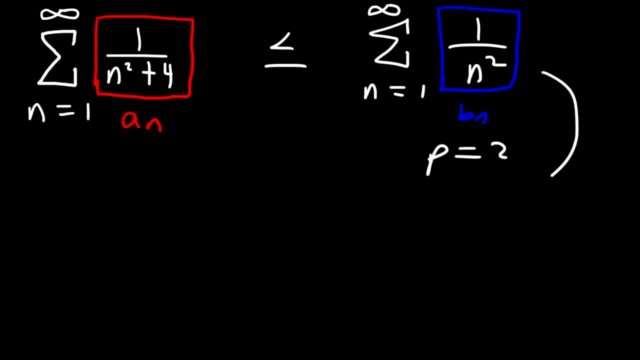 series is bigger than this one. now. series is bigger than this one. now, according to the p-series, we see that p. according to the p-series, we see that p. according to the p-series, we see that p is equal to 2. we know this series is equal to 2. we know this series. 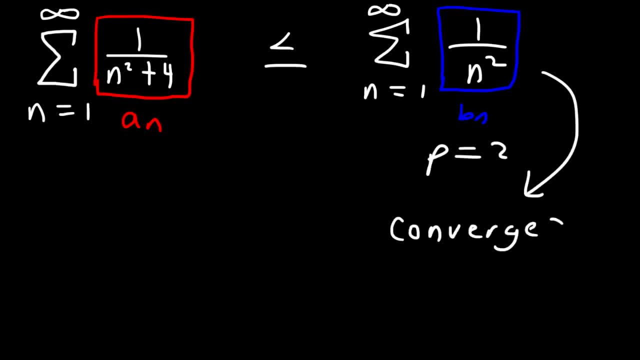 is equal to 2. we know this series converges because P is greater than 1, converges because P is greater than 1, converges because P is greater than 1. now, according to the direct comparison, now, according to the direct comparison, now according to the direct comparison tests, if the big series converges, then 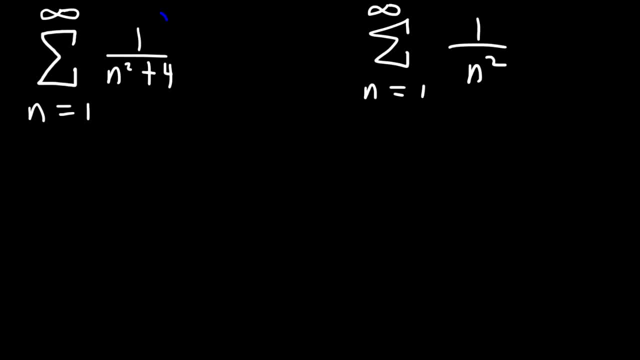 Now Which sequence is bigger: One over n squared plus four Or one over n squared? One over n squared Is greater than one over n squared plus four. If you plug in one, This would be one, And this is going to be one over five. 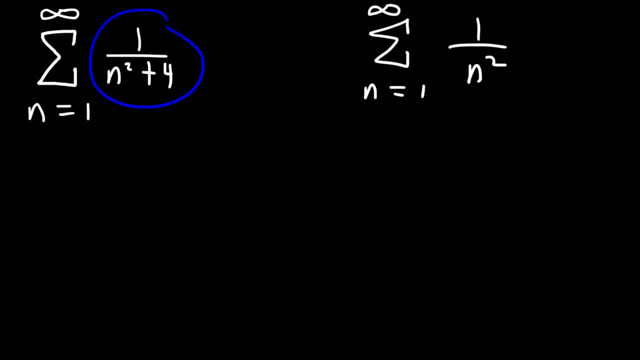 So this is always going to be bigger for all n. So therefore, we could say: This is Our a sub n term And This is Our b sub n term, So this series Is bigger Than this one Now. 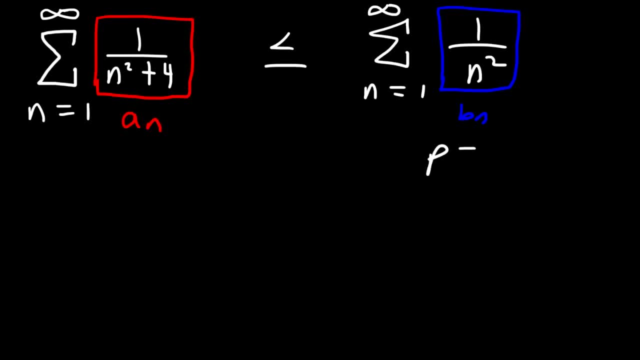 According to the p series, We see that p is equal to two. We know this series converges Because p Is greater than one. Now, According to the direct comparison test, If the big series converges, Then the small series. 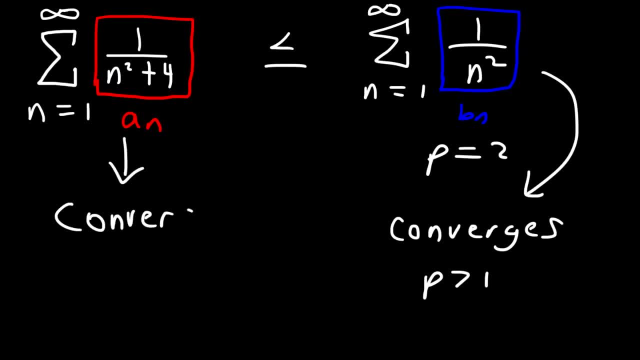 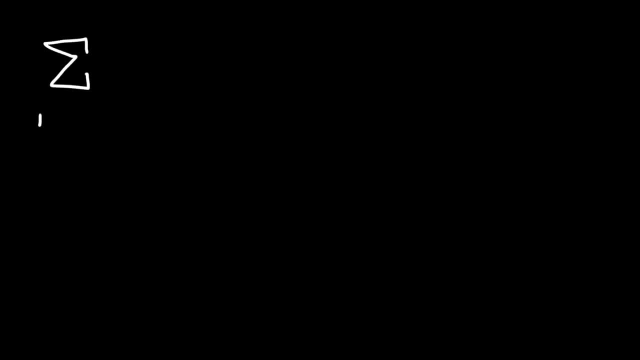 Will converge as well, And that's all we need to do for this problem. So this is going to be convergent. Now let's move on to our next problem. So let's say, If we have this series which starts from three, 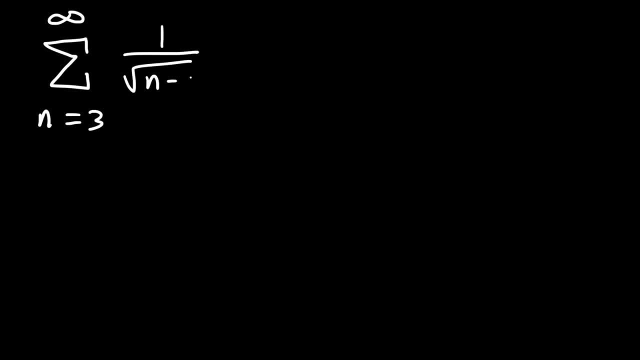 And goes to infinity, And is one over the square root of n minus two. So what sort of test Should we use In order to determine the convergence Of this series? Well, we can start with The divergence test, But when n becomes very large, 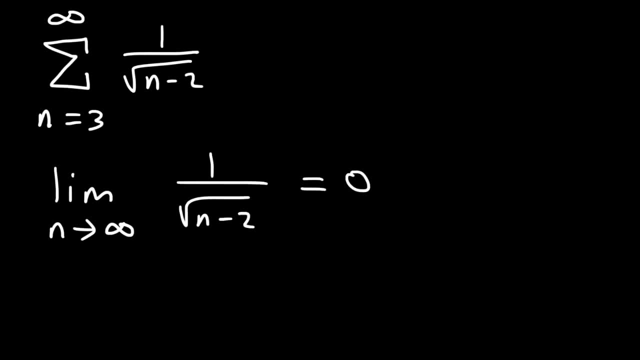 Because it's bottom heavy, The limit will go to zero And so, based on the divergence test, It may diverge or may converge. Next We could try the direct comparison test, Because if we get rid of the two, Then this becomes a p series. 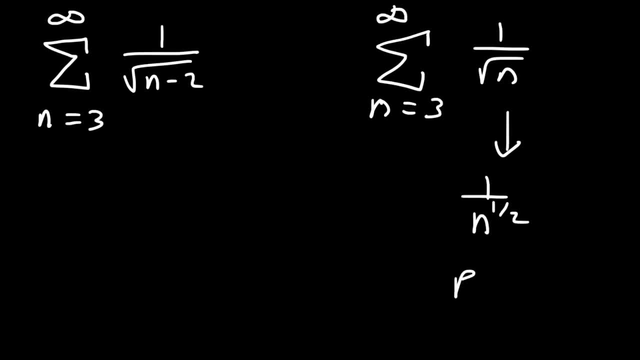 And the square root of n Is n to the one half, Which means that p is one half. So, because p is less than Or equal to one, This series Diverges. Now, which Series is bigger? Is it this one or this one? 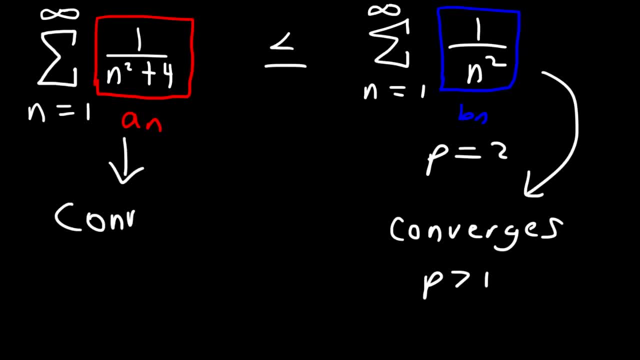 tests. if the big series converges, then tests. if the big series converges, then the small series will converge as well. the small series will converge as well. the small series will converge as well, and that's all we need to do for this, and that's all we need to do for this. 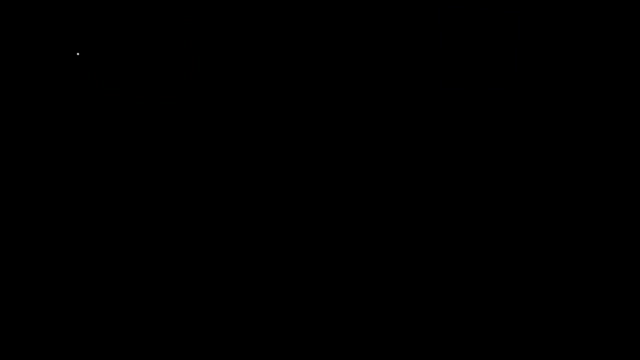 and that's all we need to do for this problem. so this is going to be problem. so this is going to be problem. so this is going to be convergent now, let's move on to our next convergent now, let's move on to our next. 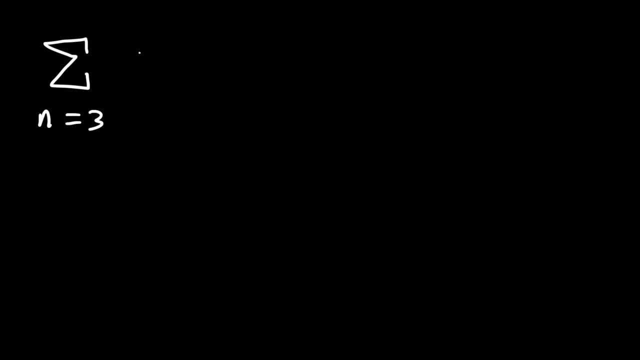 convergent. now let's move on to our next problem. so let's say: if we have the problem, so let's say: if we have the problem, so let's say: if we have the series which starts from 3 and goes to, series which starts from 3 and goes to, 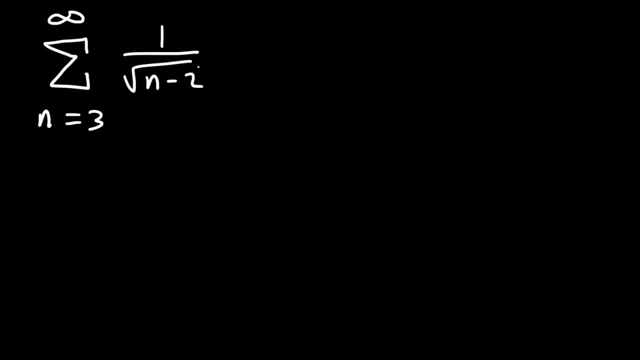 series which starts from 3 and goes to infinity, and it's 1 over the square root, infinity, and it's 1 over the square root, infinity. and it's 1 over the square root of n minus 2. so what sort of tests of n minus 2? so what sort of tests? 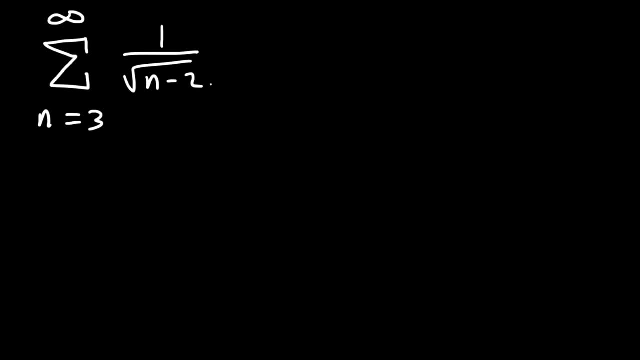 of n minus 2. so what sort of tests should we use in order to determine the? should we use in order to determine the? should we use in order to determine the convergence or the divergence of the convergence or the divergence of the convergence or the divergence of the series? well, we can start with the. 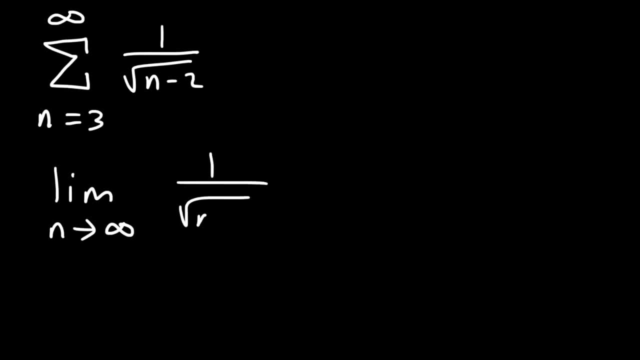 series. well, we can start with the series. well, we can start with the divergence tests. but when n becomes very divergence tests, but when n becomes very divergence tests, but when n becomes very large because it's bottom heavy, the large because it's bottom heavy, the large because it's bottom heavy, the limit will go to 0, and so, based on a, 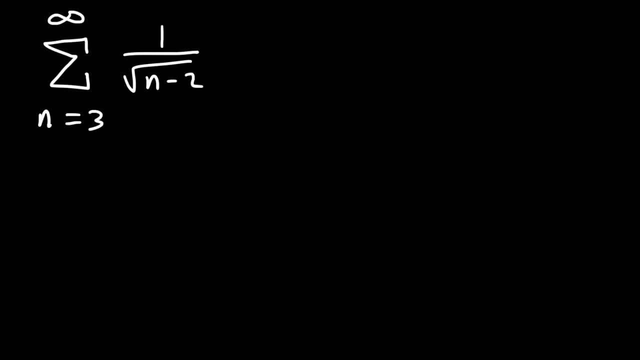 limit will go to 0, and so, based on a limit will go to 0, and so, based on a divergence test, it may diverge or may divergence test, it may diverge or may divergence test. it may diverge or may converge. next, we could try to divide. 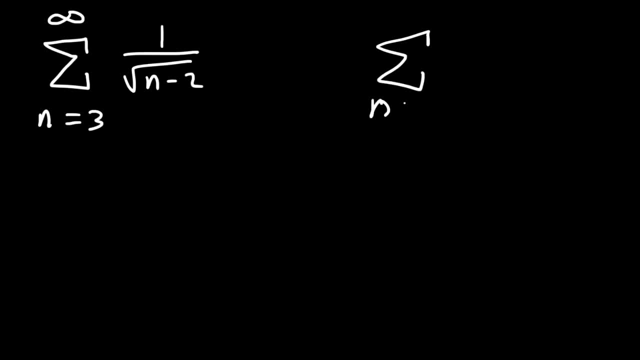 converge. next we could try to divide converge. next we could try to divide comparison tests. because if we get rid comparison tests, because if we get rid comparison tests, because if we get rid of the two, then this becomes a p-series of the two, then this becomes a p-series. 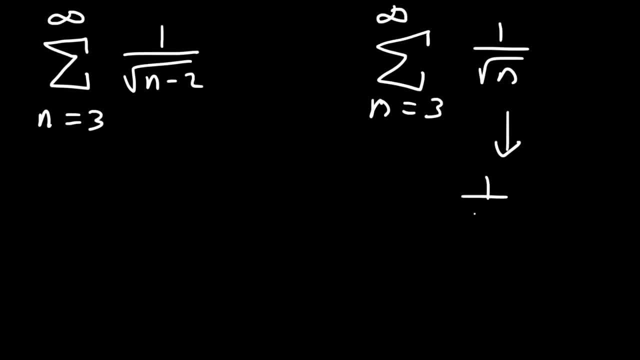 of the two. then this becomes a p-series, and the square root of n is n to the, and the square root of n is n to the, and the square root of n is n to the 1 1⁄2, which means that P is 1 1⁄2. so 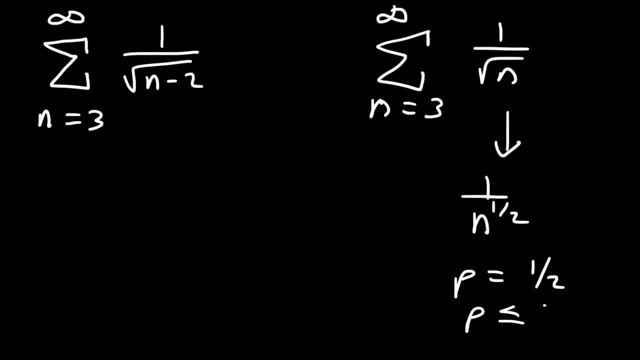 1 1⁄2, which means that P is 1 1⁄2. so 1 1⁄2, which means that P is 1 1⁄2. so, because P is less than or equal to 1, because P is less than or equal to 1, 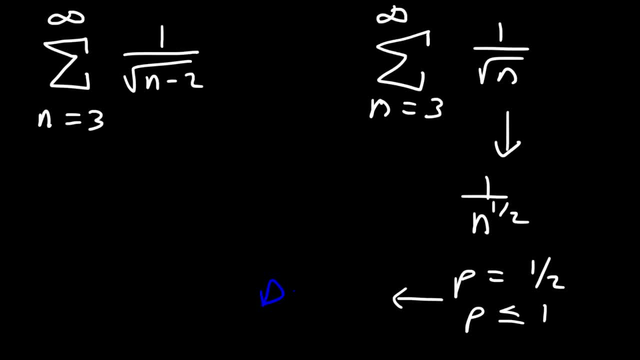 because P is less than or equal to 1. this series diverges. now. which series is bigger? is it this one? which series is bigger? is it this one? which series is bigger? is it this one or this one? because n minus 2 is less than, or this one because n minus 2 is less than? 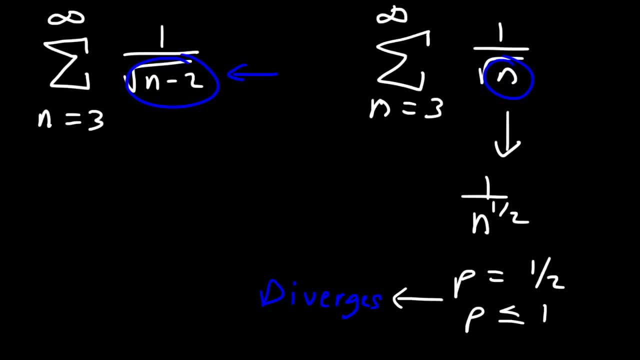 or this one, because n minus 2 is less than n, we have a smaller denominator. if you n, we have a smaller denominator. if you n, we have a smaller denominator. if you decrease the value of the denominator of decrease the value of the denominator, of decrease the value of the denominator of a fraction, the value of the whole. 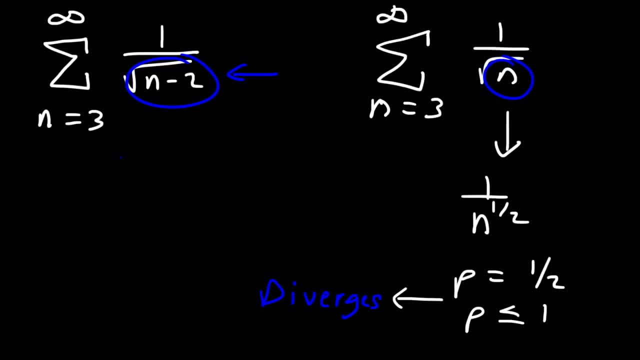 a fraction the value of the whole a fraction, the value of the whole fraction goes down. I mean, excuse me, the fraction goes down. I mean, excuse me, the fraction goes down. I mean, excuse me, the value of the whole fraction goes up. so value of the whole fraction goes up. so 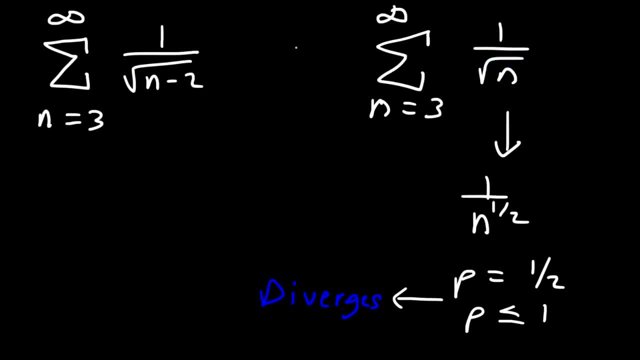 value of the whole fraction goes up. so, therefore, this series is larger. so we, therefore, this series is larger. so we, therefore, this series is larger. so we should write greater than or equal to. so should write greater than or equal to. so should write greater than or equal to. so this is going to be the big series B. 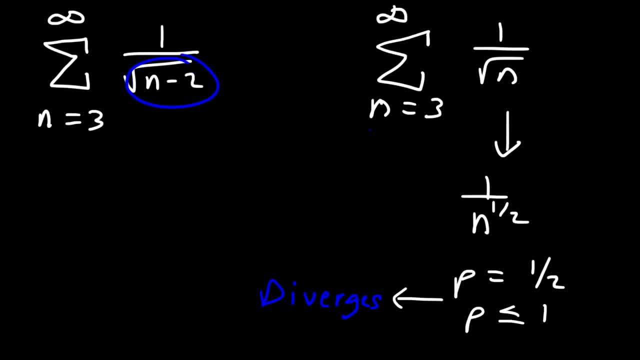 Because n minus two Is less than n. We have a smaller Denometer. So if we increase The value of The denominator of a fraction, The value of the whole fraction goes down. I mean, Excuse me, The value of the whole fraction goes up. 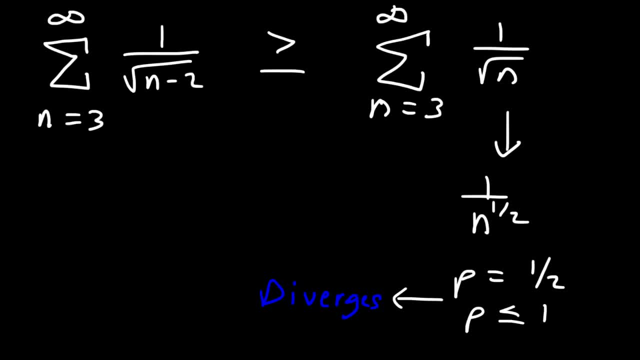 So therefore, This series is larger, So we should write greater than or equal to. So this is going to be the big series, B sub n. And this is going to be The small series, A sub n. Will the big series diverge as well? 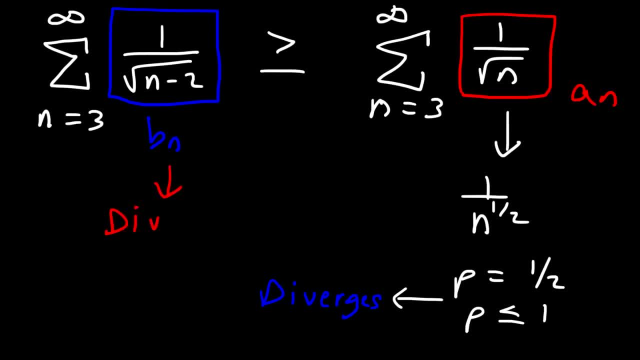 And the answer is yes. The big series must diverge as well, So this could work. Now there's another test That you could use if you want to, And that is The integral test. So let's say F of x. 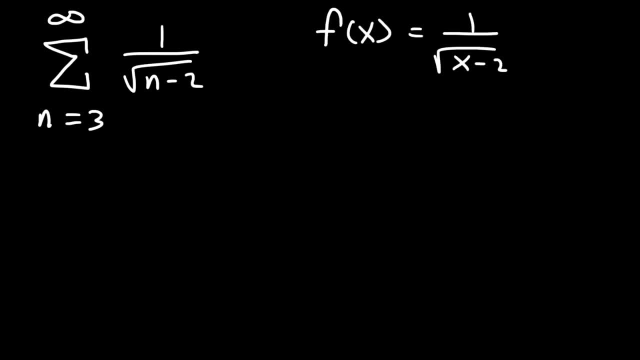 Is one divided by The square root of x minus two. Now the function Is not continuous At x equals two, Because that's a vertical asymptote. But we're starting from three, So it is continuous From three to infinity. 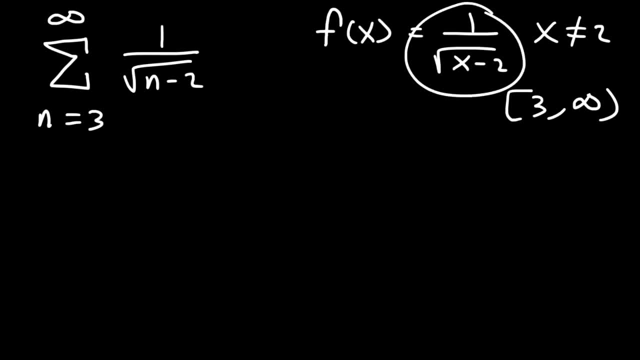 We need to show that it's continuous Decreasing and positive. This is always going to be positive, Especially when x is greater than three And Because we have a square root of x Minus two on the bottom, It's going to be a decrease in function. 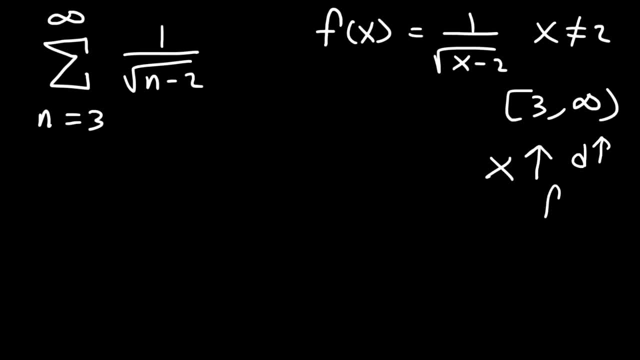 As x increases, The denominator will go up, And so the function will decrease. Now you can also find the first derivative And show that it's negative On this interval. If you do that, That tells you that the function is decreasing. 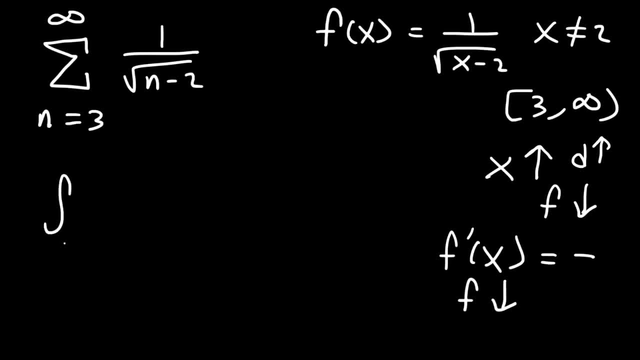 So now, Once those conditions are met, Once you show that it's positive, Continuous and decreasing On this interval, Take the integral In this case, Starting from three to infinity. Integrate f of x, dx From a to b. 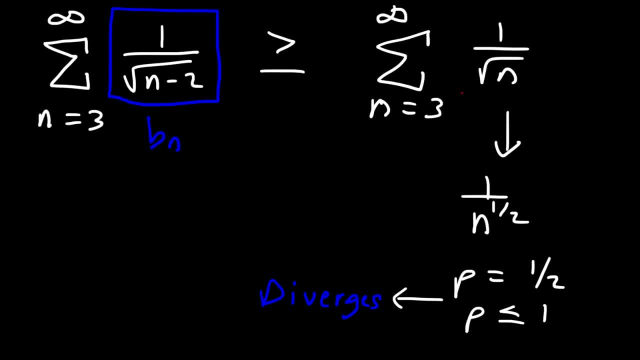 this is going to be the big series B. this is going to be the big series B sub n. and this is going to be the small sub n and this is going to be the small sub n and this is going to be the small series a sub n. so if the small series 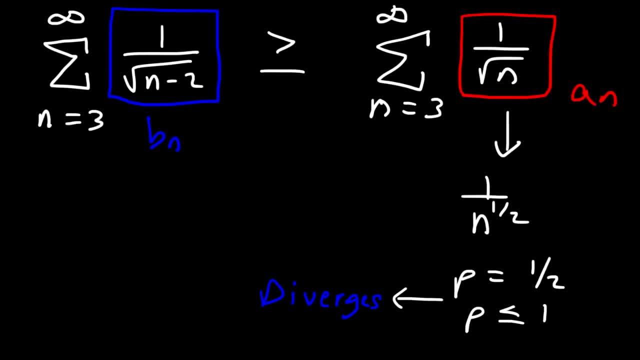 series a sub n. so if the small series series a sub n. so if the small series diverges, will the big series diverge as diverges? will the big series diverge as diverges, will the big series diverge as well? and the answer is yes, the big series. 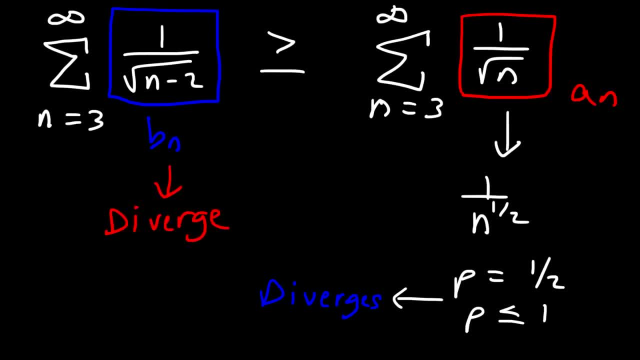 well, and the answer is yes. the big series, well, and the answer is yes, the big series must diverge as well. so this could must diverge as well. so this could must diverge as well. so this could work. now there's another test that you could. 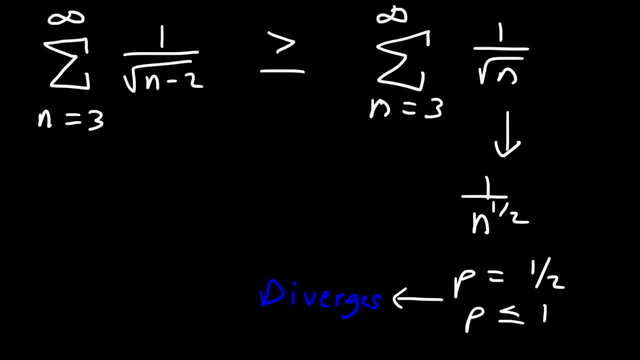 work. now there's another test that you could work. now there's another test that you could use if you want to, and that is the use if you want to, and that is the use if you want to, and that is the integral tests. so let's say f of X is 1. 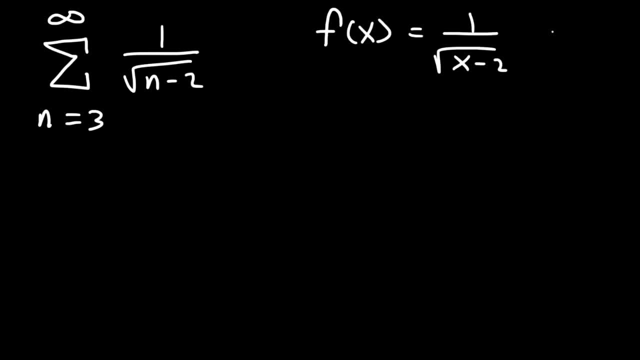 integral tests. so let's say f of X is 1. integral tests. so let's say f of X is 1 divided by the square root of X minus 2, divided by the square root of X minus 2, divided by the square root of X minus 2. now the function is not continuous at X. 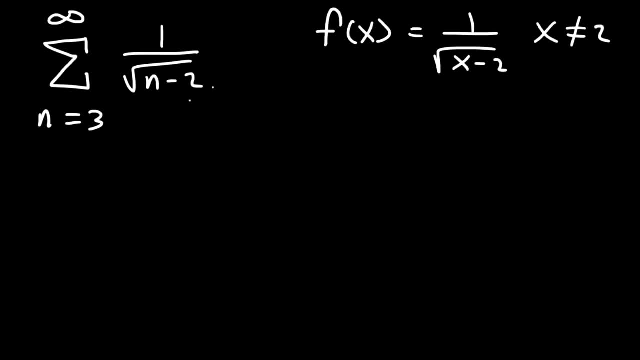 now the function is not continuous at X. now the function is not continuous at X. equals 2 because that's a vertical. equals 2 because that's a vertical equals 2 because that's a vertical asymptote. but we're starting from 3 asymptote, but we're starting from 3. 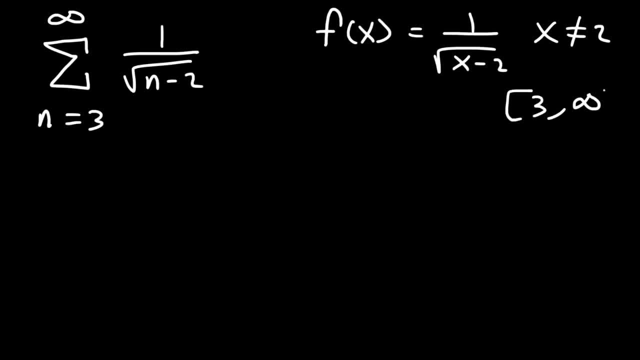 asymptote. but we're starting from 3, so it is continuous. from 3 to infinity. we, so it is continuous from 3 to infinity we, so it is continuous from 3 to infinity. we need to show that it's continuous, need to show that it's continuous. 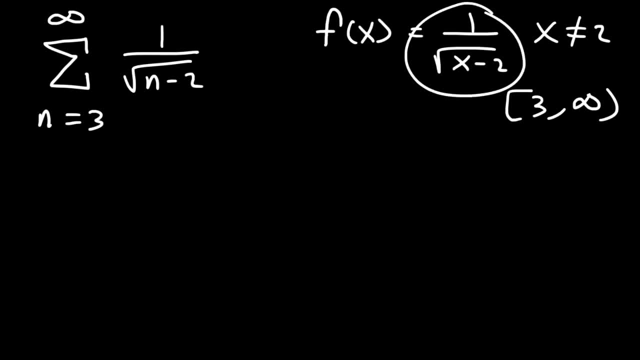 need to show that it's continuous decreasing and positive. this is always decreasing and positive. this is always decreasing and positive. this is always going to be positive, especially when X going to be positive, especially when X going to be positive, especially when X is greater than 3 and because we have a 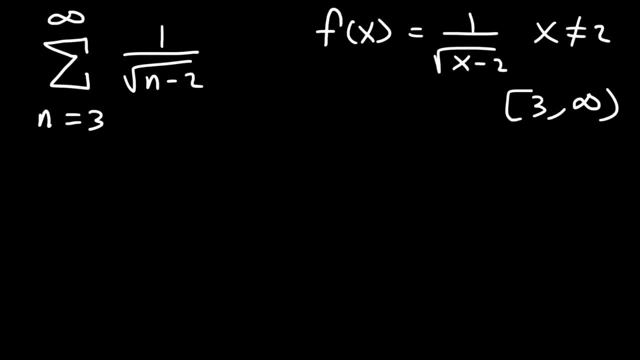 is greater than 3 and because we have a is greater than 3 and because we have a square root of X minus 2 on the bottom, square root of X minus 2 on the bottom, square root of X minus 2 on the bottom, it's going to be a decrease in function. 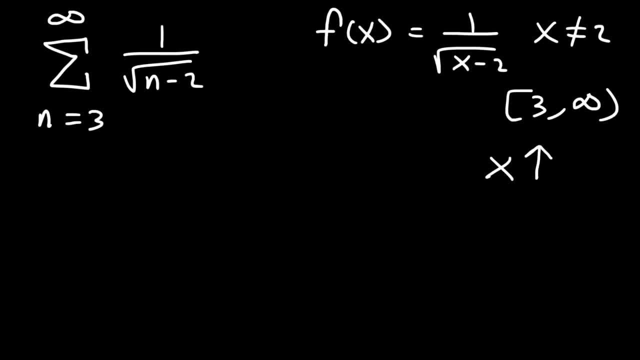 it's going to be a decrease in function. it's going to be a decrease in function as X increases the value of the. as X increases the value of the. as X increases the value of the negative on this interval. if you do that. negative on this interval. if you do that. 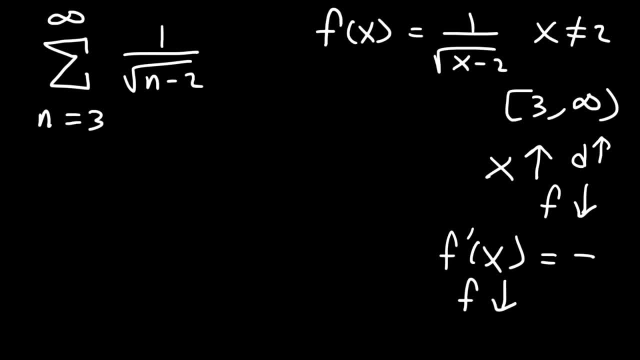 negative on this interval. if you do that, that tells you that the function is. that tells you that the function is. that tells you that the function is decreasing. so now, once those conditions decreasing, so now, once those conditions decreasing, so now, once those conditions are met, once you show that it's positive. 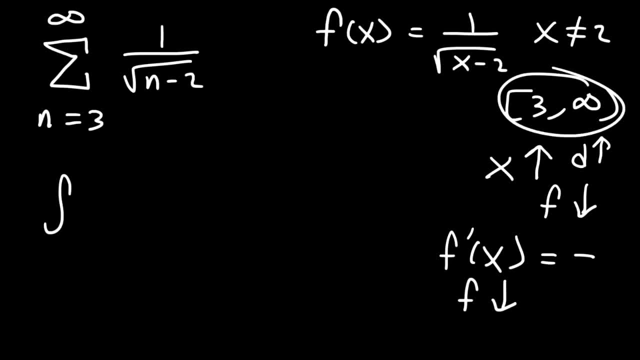 are met once you show that it's positive, are met once you show that it's positive. continuous and decreasing on this. continuous and decreasing on this, continuous and decreasing on this interval. take the integral in this case, interval. take the integral in this case, interval. take the integral in this case, starting from 3 to infinity sometimes. 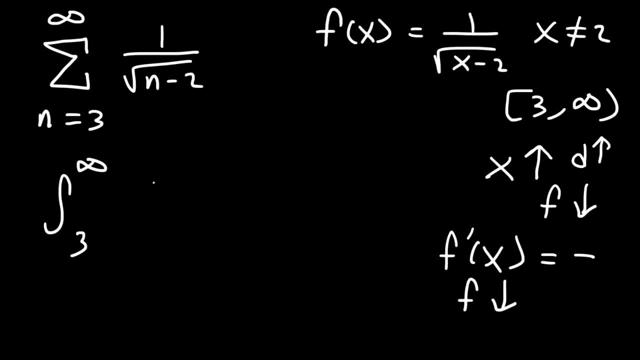 starting from 3 to infinity, sometimes starting from 3 to infinity. sometimes it's usually 1 to infinity. integrate f: it's usually 1 to infinity. integrate f: it's usually 1 to infinity. integrate f of X, DX, from a to B. so what we have here is an improper. 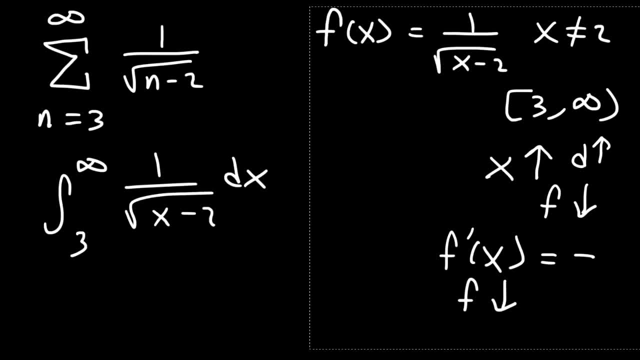 so what we have here is an improper, so what we have here is an improper integral. so first I'm going to find the integral, so first I'm going to find the integral, so first I'm going to find the indefinite integral, I'm going to use u. 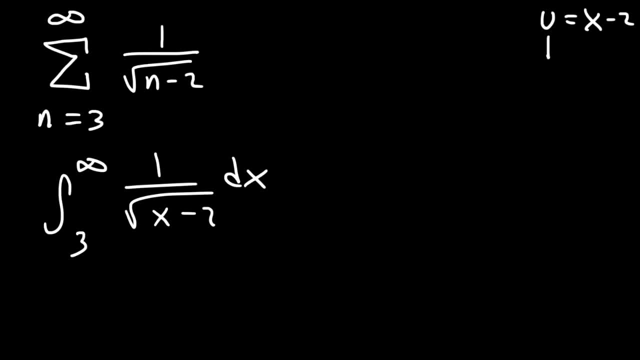 indefinite integral, I'm going to use u. indefinite integral, I'm going to use u substitution. so if I make u equal to X substitution, so if I make u equal to X substitution, so if I make u equal to X minus 2 D use can be equal to DX, and so 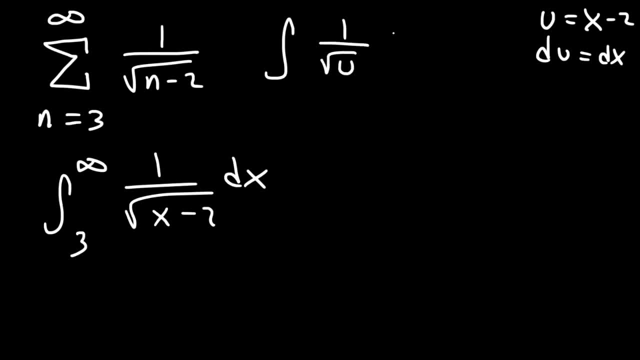 minus 2 D use can be equal to DX, and so minus 2 D use can be equal to DX, and so I can replace X minus 2 with you and DX. I can replace X minus 2 with you and DX. I can replace X minus 2 with you and DX with du, so I can rewrite this as u to. 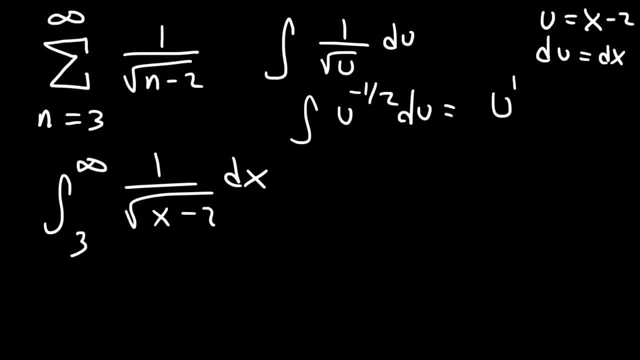 with du, so I can rewrite this as u to with du, so I can rewrite this as u to negative 1 half, and so that becomes u to negative 1 half, and so that becomes u to negative 1 half, and so that becomes u to the positive 1 half divided by 1 half. 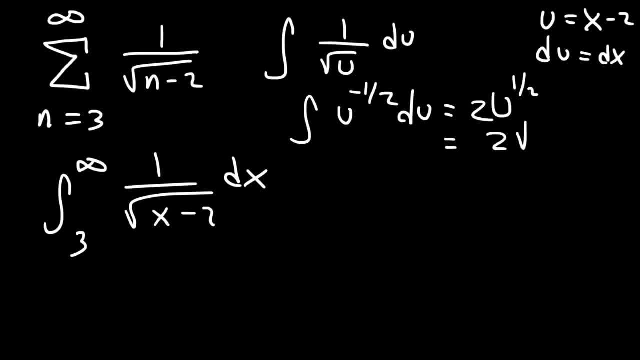 the positive 1 half divided by 1 half, the positive 1 half divided by 1 half, or multiplied by 2, and so this becomes 2. or multiplied by 2, and so this becomes 2. or multiplied by 2, and so this becomes 2 times the square root of X minus 2. 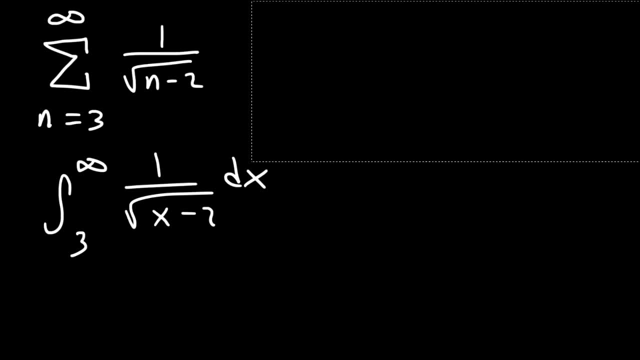 times the square root of X minus 2 times the square root of X minus 2. so this is equal to the limit as a goes. so this is equal to the limit as a goes. so this is equal to the limit, as a goes to infinity, of 2 times the square root. 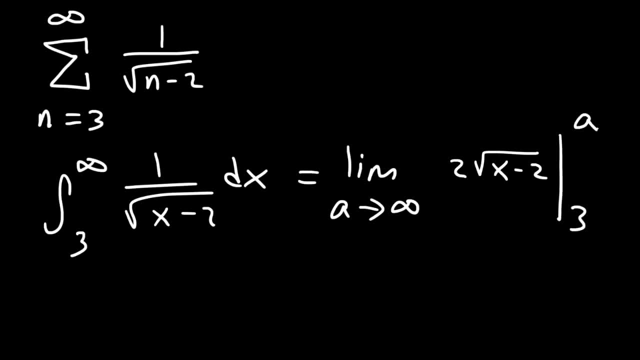 to infinity of 2 times the square root to infinity of 2 times the square root of X minus 2, evaluated from 3, to of X minus 2, evaluated from 3 to of X minus 2, evaluated from 3 to a. so now let's plug in a and 3, so we're. 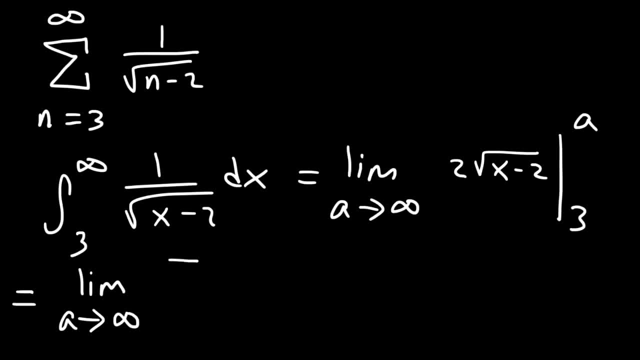 a. so now let's plug in a and 3. so we're a. so now let's plug in a and 3. so we're gonna have the limit as a goes into, gonna have the limit as a goes into, gonna have the limit as a goes into infinity, and this is going to be 2 times. 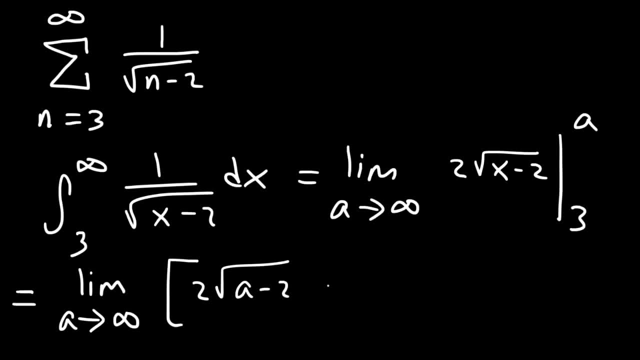 infinity, and this is going to be 2 times infinity, and this is going to be 2 times the square root of a minus 2 plus 2, the square root of a minus 2 plus 2, the square root of a minus 2 plus 2 times. I'm not plus, but minus minus 2. 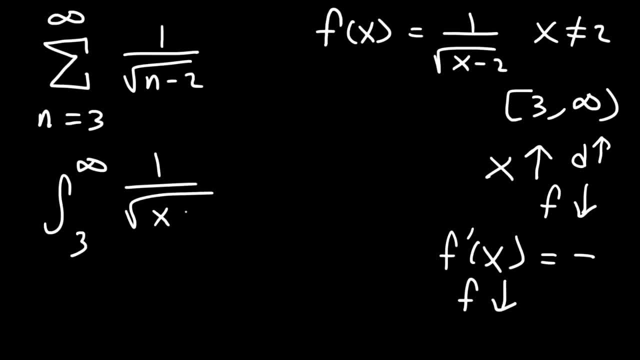 So what we have here Is an improper integral. So first I'm going to find the indefinite integral, I'm going to use u substitution. So if I make u equal to x minus two, Du is going to be equal to dx. 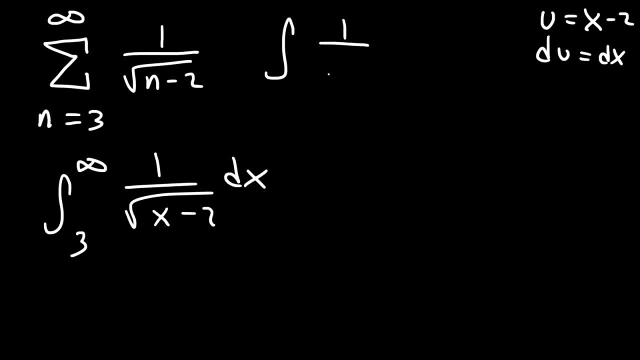 And so I can replace X minus two with u And dx with du, So I can rewrite this As u to negative one half, And so that becomes u to the Positive one half Divided by one half Or multiplied by two. 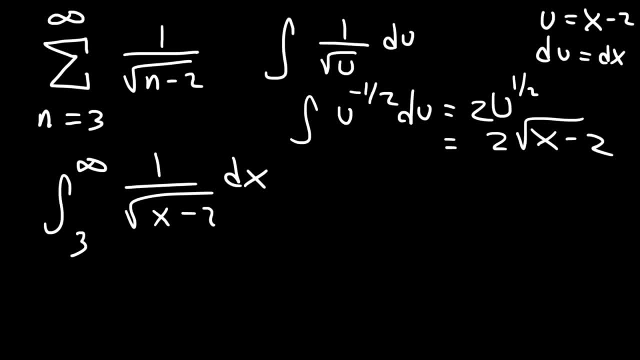 And so this becomes two times the square root Of x minus two. So this is equal to the limit, As a goes to infinity, Of two times The square root of x minus two, Evaluated from three To a. So now, 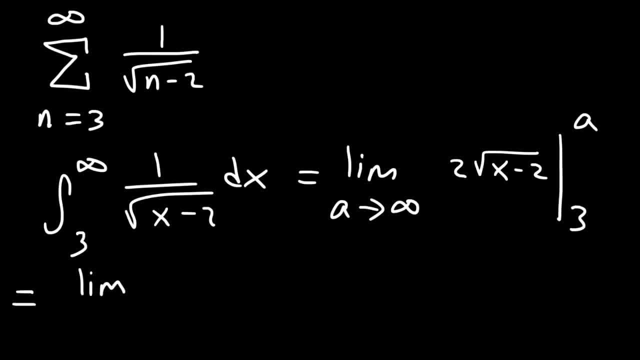 Let's plug in a and three, So we're going to have the limit As a goes into infinity, And this is going to be two times The square root of a minus two Plus Two times Minus, Minus, two times. 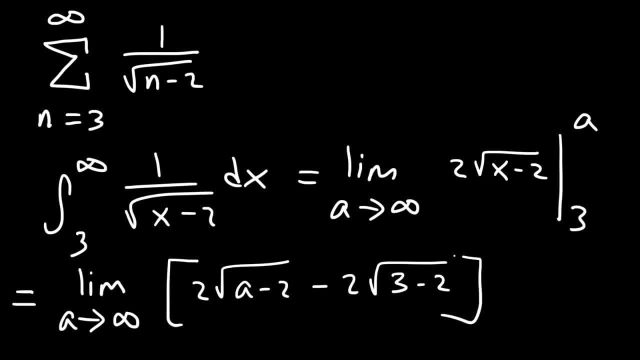 The square root of three minus two. Now, As a goes to infinity, This whole expression Becomes infinity. And so infinity minus Two times one Is just infinity. So if the integral test gives you infinity, That means that the original series. 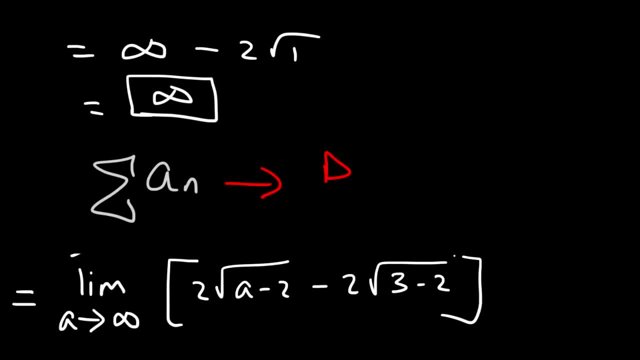 Diverges, Which was in harmony With the other conclusion that we got, Based on the direct comparison test. Let's say, If We have the series Of the square root of n Divided by n cubed plus two. 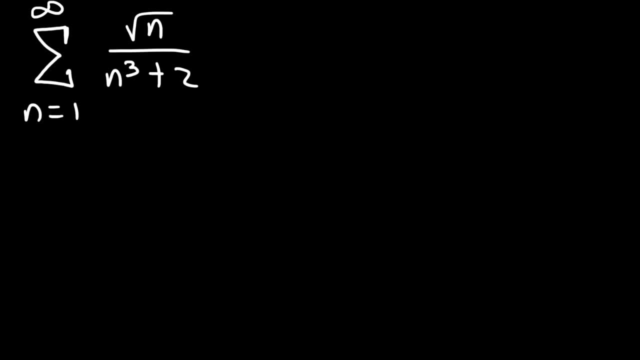 Which test should we use For this one? The test that I recommend using Is the limit comparison test, But we need two separate functions, One of which Is More simplified than the other, So for the other series, I'm just going to get rid of the two. 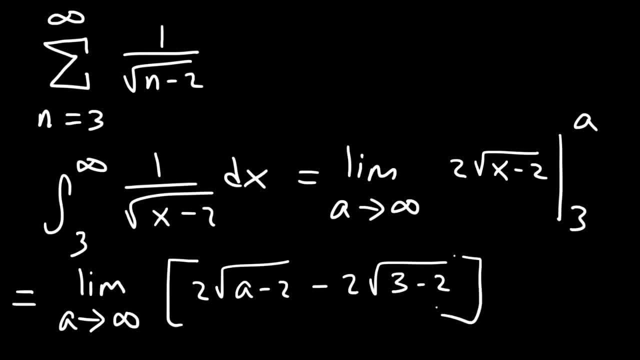 times I'm not plus, but minus minus 2 times I'm not plus but minus minus 2 times the square root of 3 minus 2. now. times the square root of 3 minus 2. now times the square root of 3 minus 2. now as a goes to infinity. 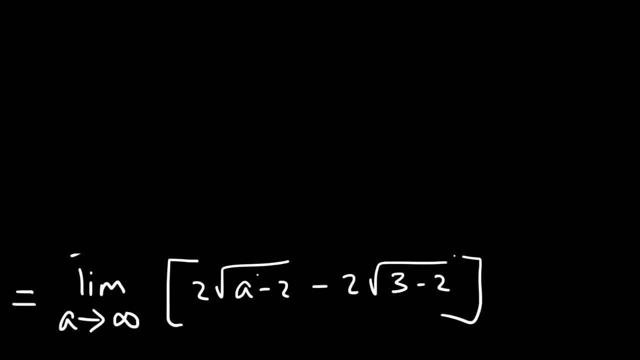 as a goes to infinity, as a goes to infinity, this whole expression becomes infinity. this whole expression becomes infinity. this whole expression becomes infinity. and so infinity minus 2 times 1 is just, and so infinity minus 2 times 1 is just, and so infinity minus 2 times 1 is just infinity. so if the integral test gives: 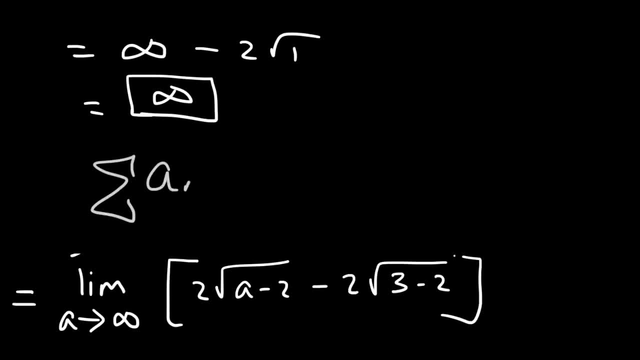 infinity. so if the integral test gives infinity, so if the integral test gives you infinity, that means that the original you infinity. that means that the original you infinity. that means that the original series diverges, which was in harmony series- diver increases. which was in harmony series- diver increases, which was in harmony with the other conclusion that we 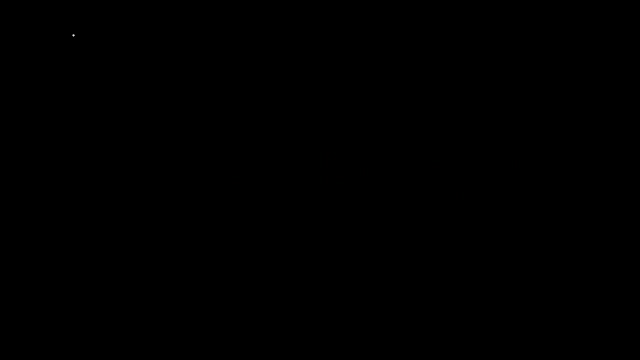 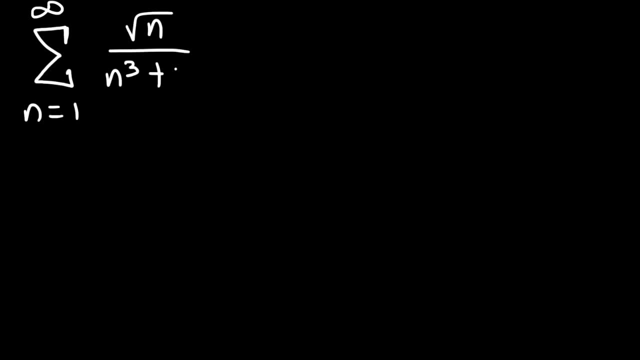 let's say, if we have the series of the square root of n divided by N Q plus 2. square root of n divided by N Q plus 2. square root of n divided by N Q plus 2, which test should we use for this one? 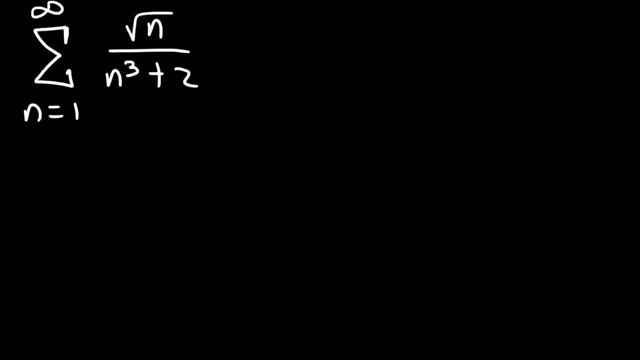 which test should we use for this one? which test should we use for this one? the test that I recommend using is the. the test that I recommend using is the. the test that I recommend using is the limit comparison test, but we need two limit comparison test, but we need two. 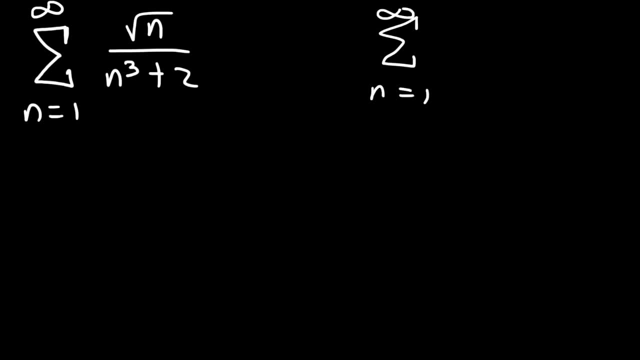 limit comparison test. but we need two separate functions, one of which is more separate functions, one of which is more separate functions, one of which is more simplified than the other. so for the simplified than the other, so for the simplified than the other. so, for the other series, I'm just going to get rid. 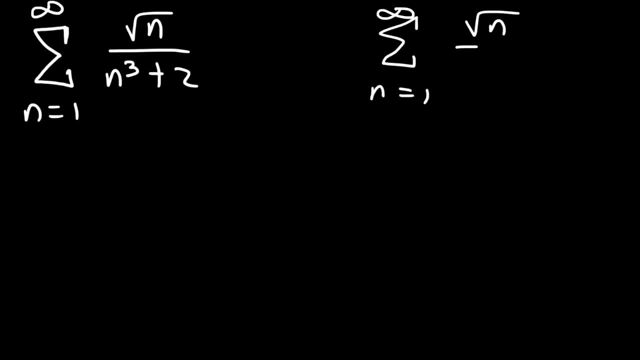 other series. I'm just going to get rid. other series. I'm just going to get rid of the two. so it becomes the square of the two. so it becomes the square of the two. so it becomes the square root of n divided by N cube, and according to: 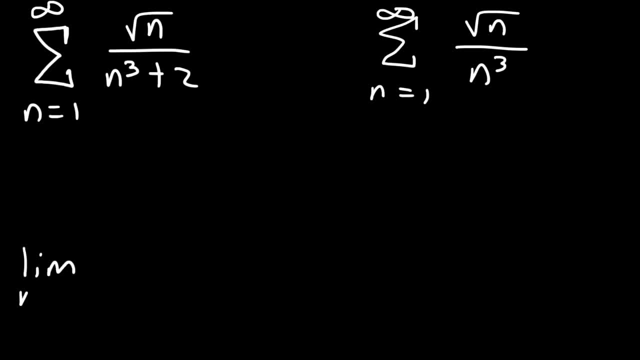 root of n divided by N cube and according to root of n divided by N cube. and according to the limit comparison tests, if we take the limit comparison tests, if we take the limit comparison tests, if we take the limit as n goes to infinity of the, the limit as n goes to infinity of the. 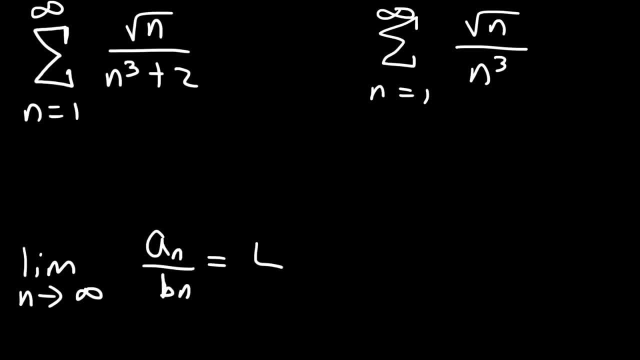 the limit, as n goes to infinity, of the ratio of the two sequences. if it's equal ratio of the two sequences, if it's equal ratio of the two sequences, if it's equal to a finite positive number, then both to a finite positive number, then both to a finite positive number, then both series will either converge or they will. 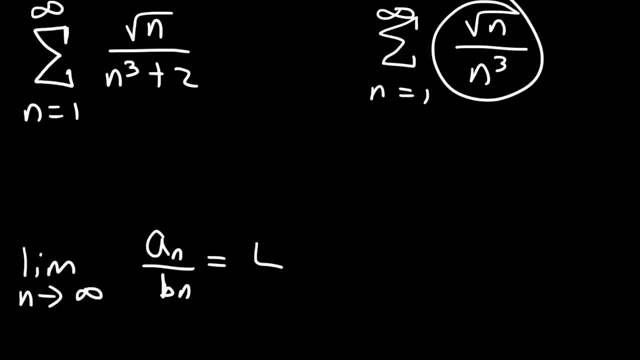 series will either converge or they will. series will either converge or they will both diverge. now we can reduce this to a both diverge. now we can reduce this to a both diverge. now we can reduce this to a p-series. so this is n to the one-half. 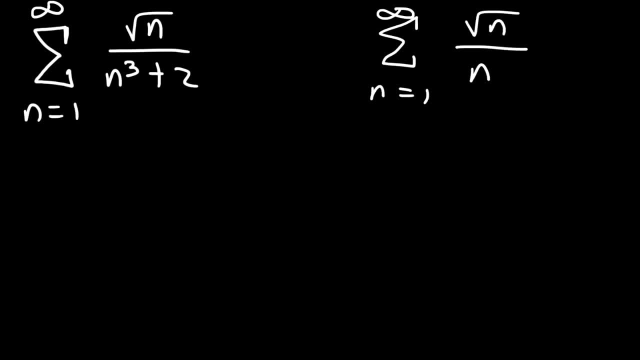 Because we're going to use The square root of n Divided by n cubed And according to the limit comparison test, If we take the limit As n goes to infinity Of the ratio of the two sequences If it's equal to a finite positive number. 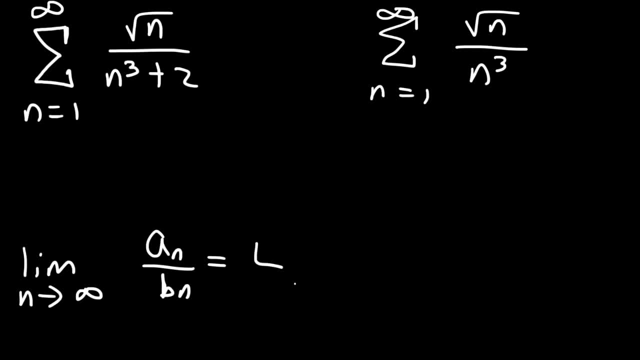 Then Both series will either Converge or they will both diverge. Now we can reduce this To a p series. So this is N to the one, Half Divided by n cubed, And so a half minus three is two point five. 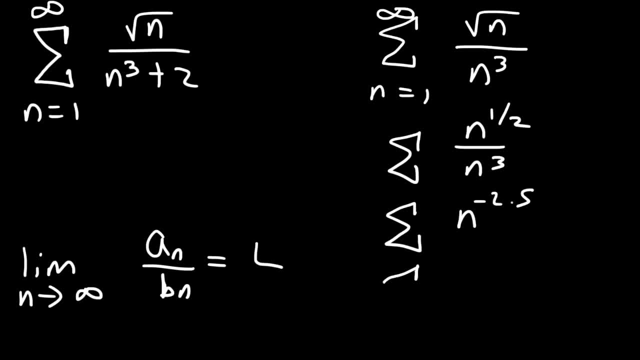 Negative two point five, And so this becomes One over n To the two point five. So p is two point five And that's greater than one. So according to the p series test, This series Converges. So if this passes the limit, comparison test. 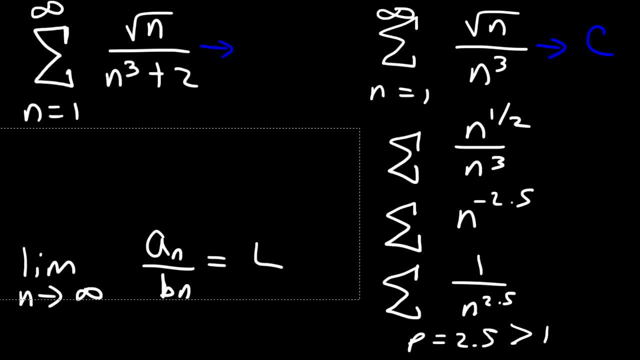 It will also converge. Let's find out The limit Of a sub n Divided by b sub n. Now let's take the limit, As n goes to infinity, Of a sub n Divided by b sub n. So let's call this: 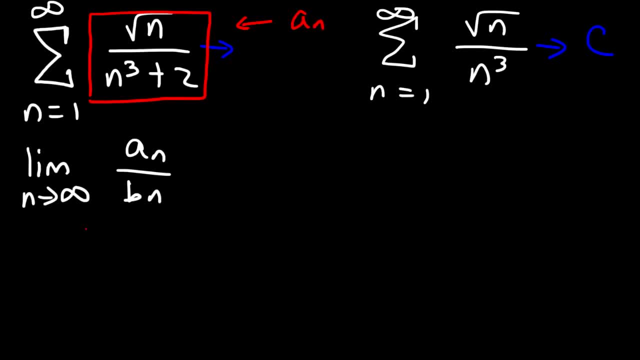 Our A sub n And this expression Is going to be our B sub n Sequence. So this is going to be the limit, As n goes to infinity And then a sub n. That's the square root of n. 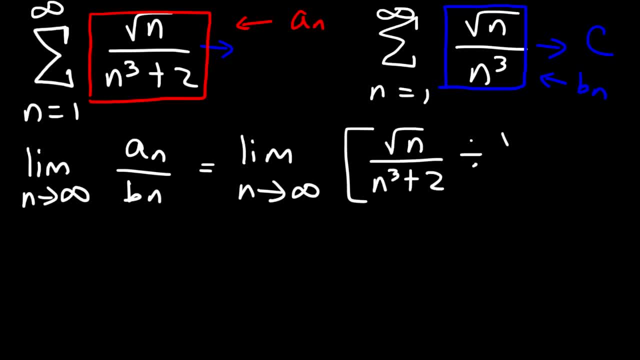 Divided by n to the third plus two, And then divided by B sub n, Which is the square root of n Over n cubed. Perhaps you heard of the expression Keep, change flip. Keep the first fraction the same, Change division to multiplication. 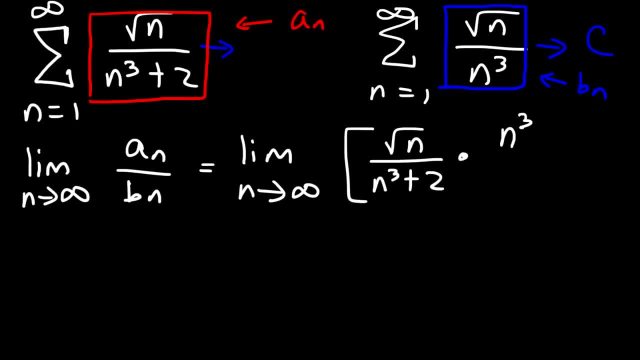 Flip the second fraction So we can rewrite this as Times. So these two will cancel, And so we have the limit, As n goes to infinity, Of n cubed Divided by n cubed Plus two. So let's multiply the top. 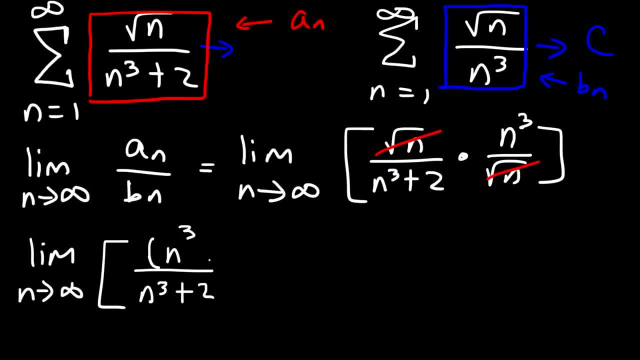 And the bottom By one over N cubed. So if we do that, We're going to get the limit As n approaches infinity, And this is going to be one Divided by one plus Two times one over n cubed. 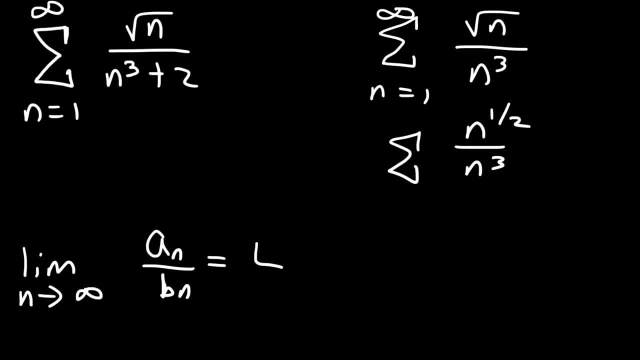 p-series. so this is n to the one-half p-series, so this is n to the one-half divided by n cubed, and so a half minus divided by n cubed, and so a half minus divided by n cubed, and so a half minus 3 is 2.5 negative 2.5, and so this: 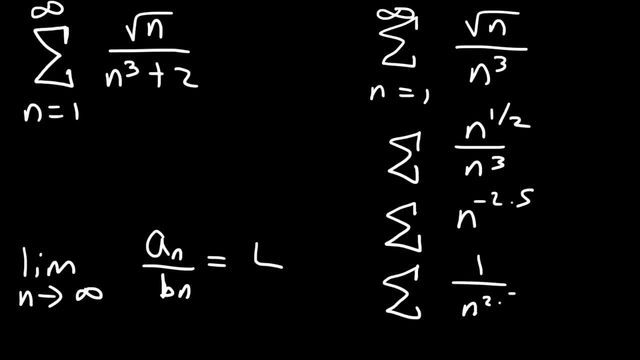 3 is 2.5 negative 2.5, and so this 3 is 2.5 negative 2.5, and so this becomes 1 over n to the 2.5, so P is 2.5, becomes 1 over n to the 2.5, so P is 2.5. 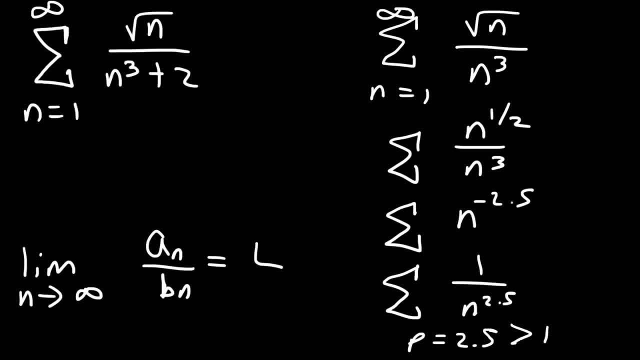 becomes 1 over n to the 2.5. so P is 2.5 and that's greater than 1. so according and that's greater than 1. so according to the p-series test, this series to the p-series test, this series to the p-series test, this series converges. so if this passes the limit, 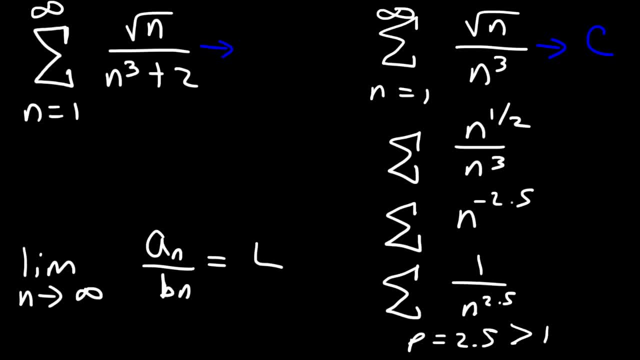 converges. so if this passes the limit converges. so if this passes the limit, comparison test, it will also converge. comparison test: it will also converge. comparison test- it will also converge. let's find out now. let's take the limit as n goes to now. let's take the limit as n goes to. 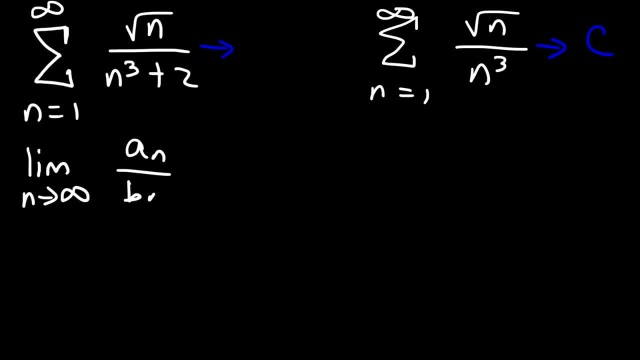 now let's take the limit, as n goes to infinity of a sub n divided by B sub n. infinity of a sub n divided by B sub n. infinity of a sub n divided by B sub n. so let's call this our. so let's call this our. 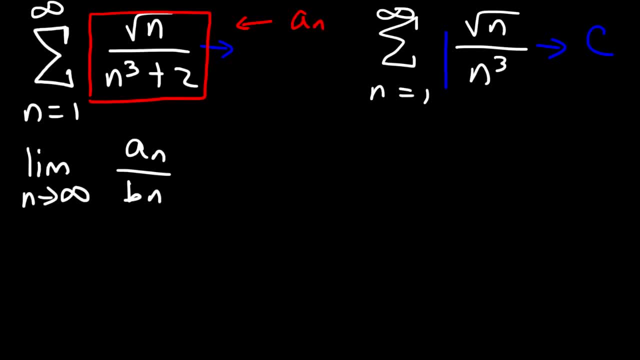 so let's call this our a sub n, and this expression is going to be a sub n, and this expression is going to be a sub n, and this expression is going to be our B sub n sequence. so this is going, our B sub n sequence. so this is going. 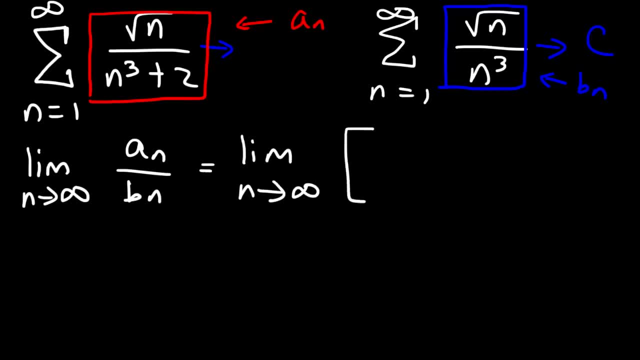 our B sub n sequence. so this is going to be the limit as n goes to infinity, and to be the limit as n goes to infinity, and to be the limit as n goes to infinity. and then a sub n. that's the square root, then a sub n. that's the square root. 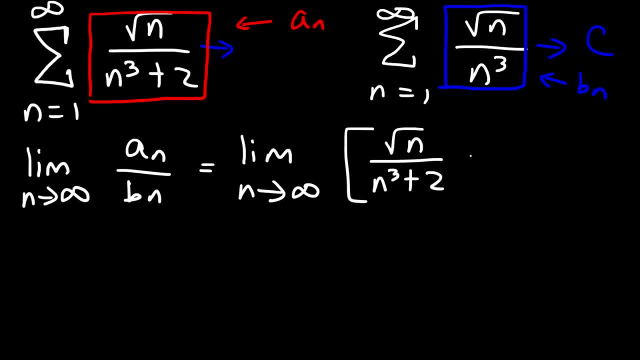 then a sub n, that's the square root of n divided by n to the third plus 2, and of n divided by n to the third plus 2, and of n divided by n to the third plus 2, and then divided by B sub n, which is the. 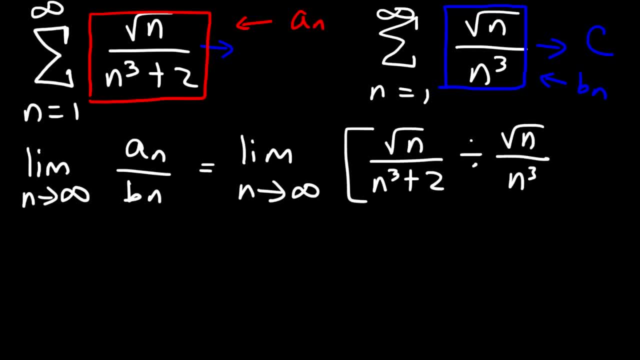 then divided by B sub n, which is the, then divided by B sub n, which is the square root of n over n cube. perhaps you square root of n over n cube. perhaps you square root of n over n cube. perhaps you heard of the expression keep change flip. 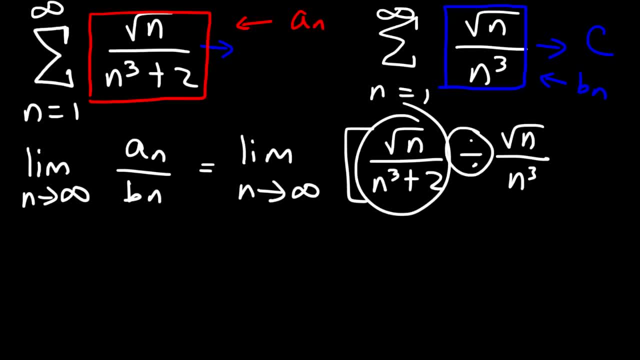 heard of the expression keep change flip. heard of the expression keep change flip. keep the first fraction the same change. keep the first fraction the same change. keep the first fraction the same change. division and multiplication: flip the division and multiplication. flip the division and multiplication. flip the second fraction. so we can rewrite this: 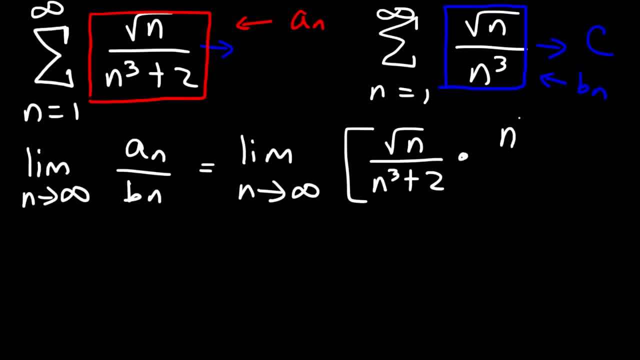 second fraction. so we can rewrite this second fraction. so we can rewrite this as times n to the third divided by the, as times n to the third divided by the, as times n to the third divided by the square root of n. so these two will square root of n. so these two will. 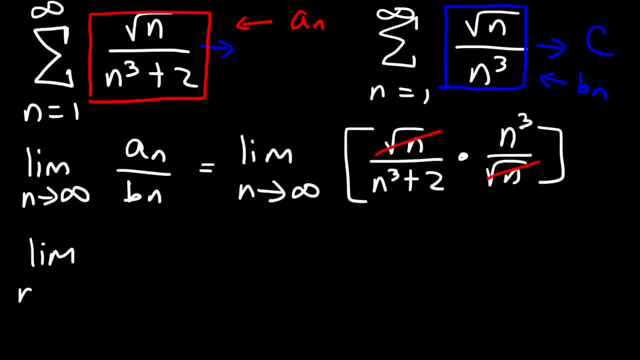 square root of n. so these two will cancel. and so we have the limit as n cancel. and so we have the limit as n cancel. and so we have the limit, as n goes to infinity, of n cubed divided by n cube plus 2.. So let's multiply the top and the bottom by 1 over n cubed, So if 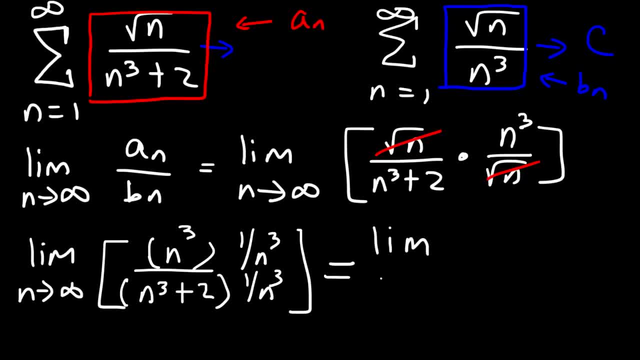 we do that, we're going to get the limit as n approaches infinity, and this is going to be 1 divided by 1 plus 2 times 1 over n cubed. So when n becomes very large, 1 over n cubed goes to 0. So it's 1 over 1 plus 2 times 0, which is 1 over. 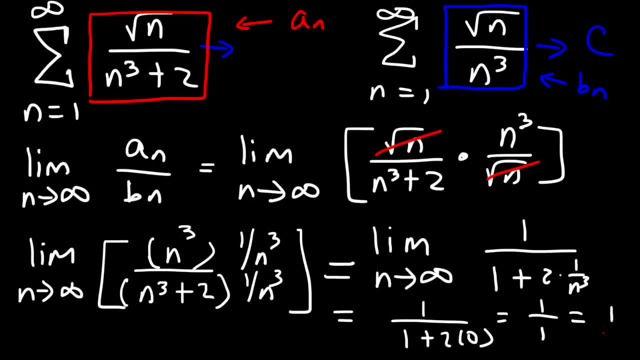 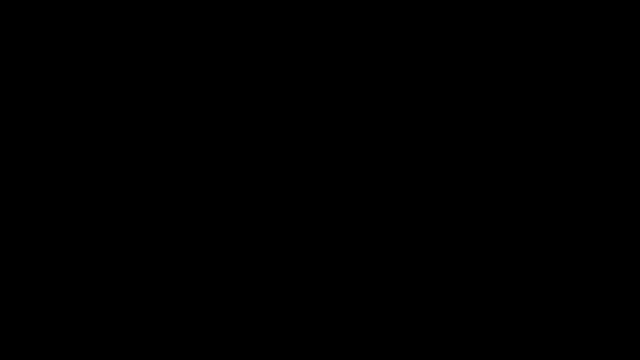 1 and that's 1.. So this is equal to a finite positive number. Therefore, according to the limit comparison test, because this series converges, this one must converge as well. Now consider the next example. Let's say it's 3n squared minus 9 divided by 7n. 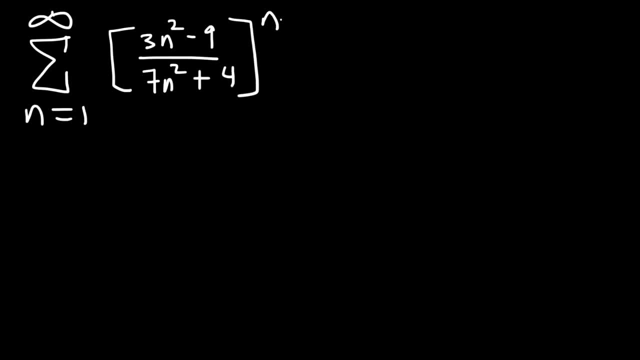 squared plus 4 raised to the n, Which test should we use? If you see something raised to the n power, it's a good indication that we need to use the root test. So recall that the root test is this: Take the limit as n goes to infinity. 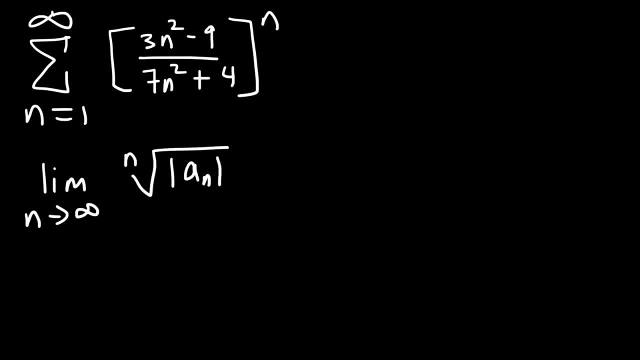 Of the nth root of the absolute value of the sequence a, sub n. Now, if it's less than 1, the series converges. If it's greater than 1, or if it's infinity, the series diverges. If it's equal to 1, then it's inconclusive. 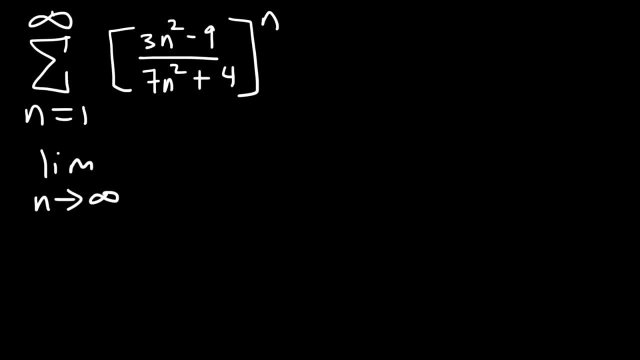 So if we take the limit as n goes into infinity of the nth root, which is the same as infinity, Notice that the degree of the numerator is the same as raising everything to the 1 over n, power n times one over n. those will cancel And so we have the limit as n goes to. 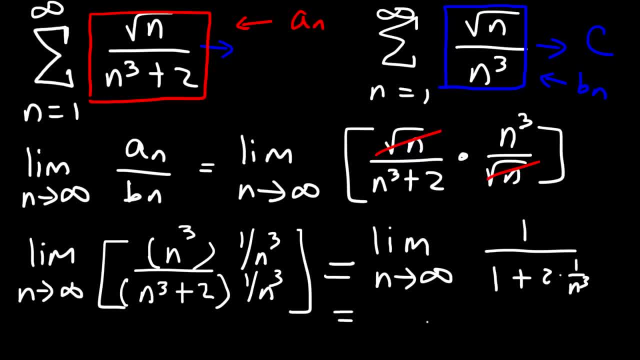 So when n becomes very large, One over n cubed goes to zero. So it's one over one plus Two times zero, Which is one over one And that's one. So this is equal to a finite positive number. Therefore, according to the, 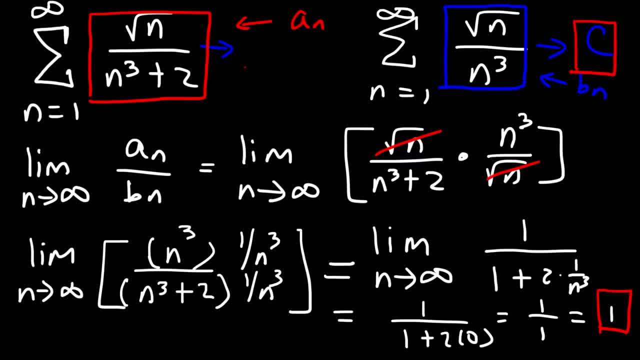 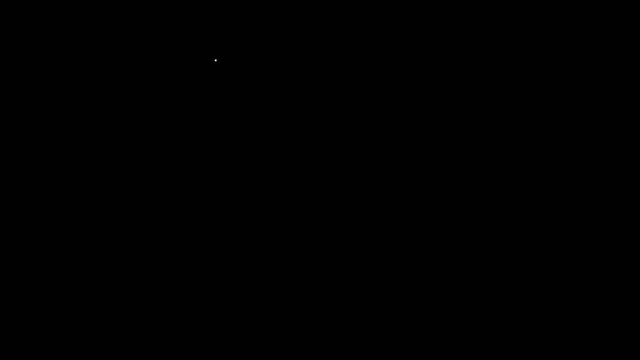 Limit comparison test. Because this series converges, This one must converge as well. Now consider the next example. Let's say it's three n squared Minus nine Divided by Seven n squared Plus four Raised to the n. 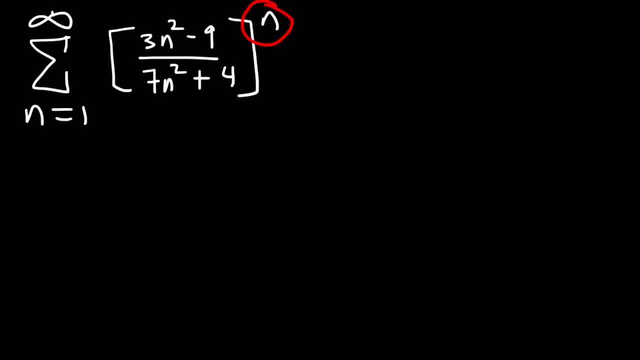 Which tests should we use? If you see something Raised to the n power, It's a good indication that We need to use the root test. So recall that The root test is this: Take the limit, as n goes to infinity. 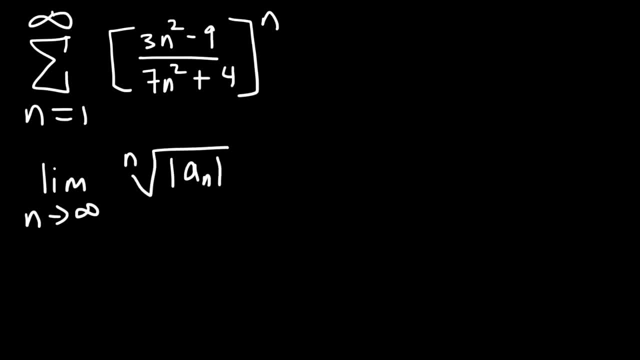 Of the nth root Of the absolute value Of the sequence a, sub n. Now, if It's less than one, The series converges. If it's greater than one, It's equal to one. Then it's inconclusive. So if we take the limit, 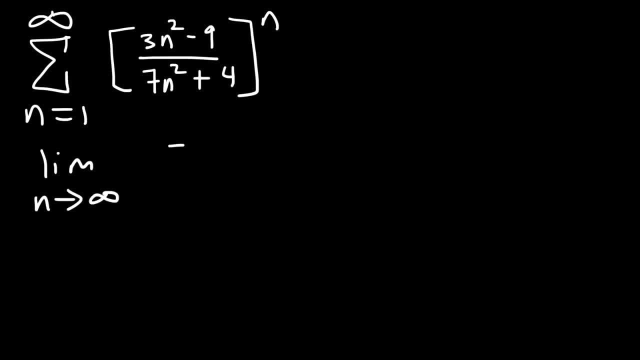 As n goes into infinity, Of the nth root, Which is the same as Raising everything To The one over n power Plus four N times one over n. Those will cancel, And so We have the limit As n goes to infinity. 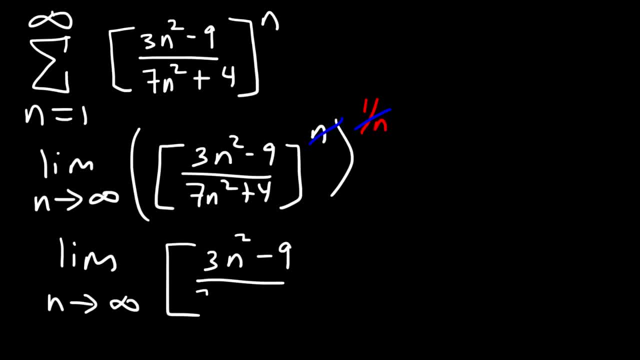 Of three n squared Minus nine, Divided by seven n squared Plus four. Notice that the degree of the numerator Is the same as that of the denominator. So you can see that the limit Is going to be three over seven. 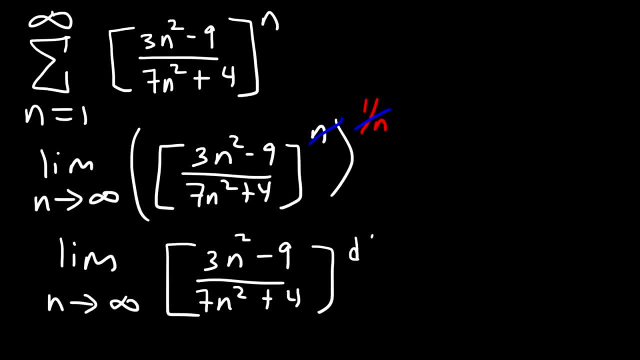 But if you want to show your work With n squared Or use L'Hopital's rule, Let's use L'Hopital's rule for this example. So the derivative Of three n squared is six n And the derivative of seven n squared. 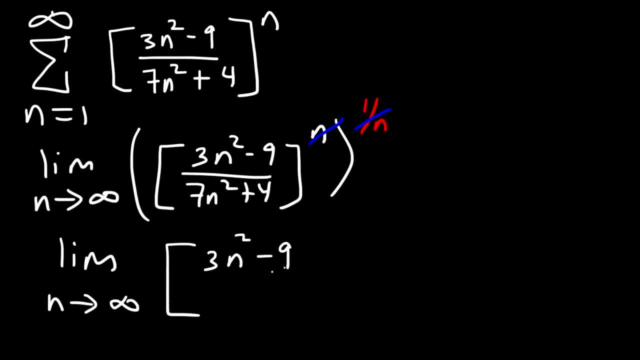 infinity of 3n squared minus 9, divided by 7n squared plus 4.. Notice that the degree of the numerator is the same as the degree of the denominator, that of the denominator. so you can see that the limit is going to be 3 over 7. 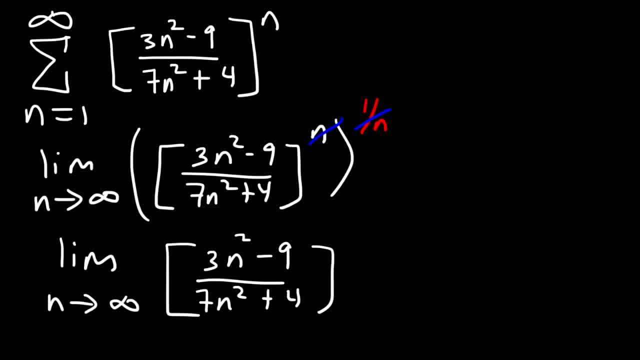 but if you want to show your work, you can multiply the top and the bottom by 1 over N squared, or use L'Hopital's rule. let's use L'Hopital's rule for this example. so the derivative of 3 N squared is 6 N and the derivative of 7 N squared. 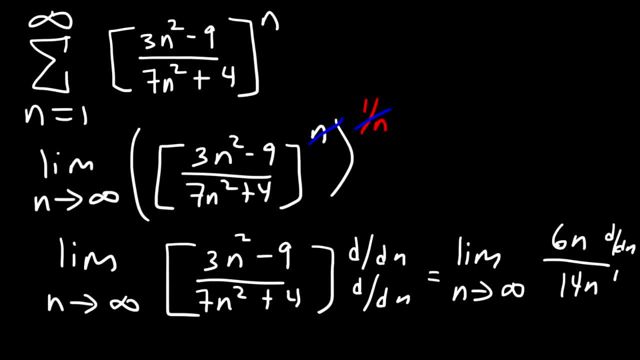 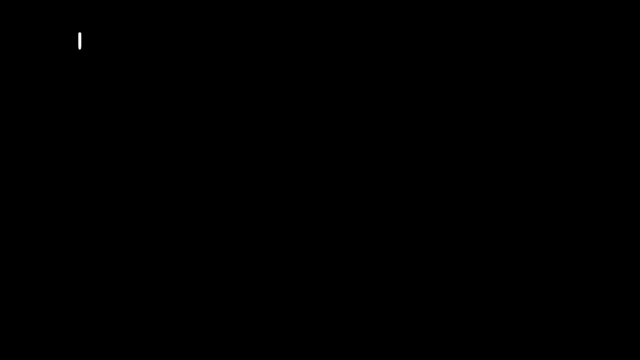 is 14 N. so using L'Hopital's rule again, this is going to become 6 over 14, which reduces to 3 over 7. so this is the answer. now, 3 over 7 is less than 1, so based on the root tests, the series converges. now let's work on our final. 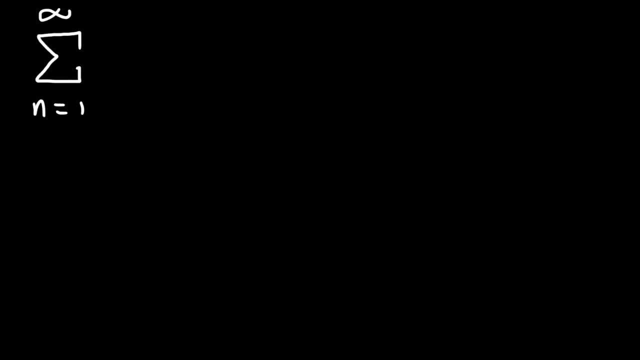 example, and so we're going to have the series of 2 raised to the N divided by N factorial. so what tests should we use for this example? so, since you know it's the last problem, it's going to be the test that we haven't used. 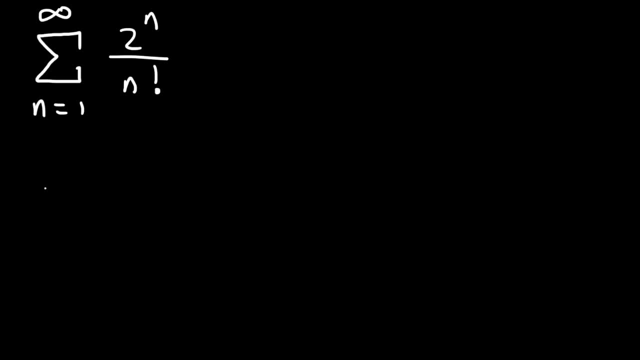 yet, which is the ratio test, and so the basic idea behind a ratio test is we need to take the a sub N plus 1 and divided by a sub N, all within an absolute value symbol, and if this is less than 1, the series converges. if it's a. 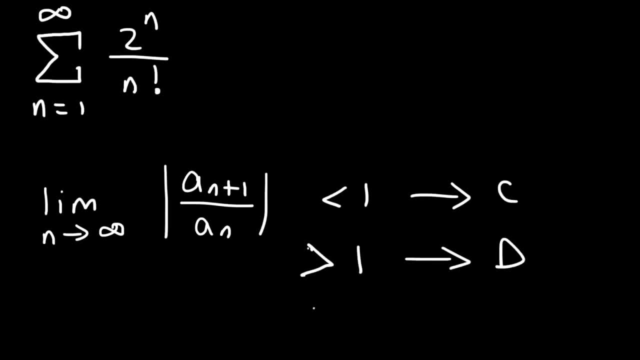 greater than 1 or equals infinity, the series diverges. now if it's equal to 1, then it's inconclusive. now we know that a sub N is 2 to the N over N factorial. but what's a sub N plus 1? all you need to do is replace N with N plus 1, so the 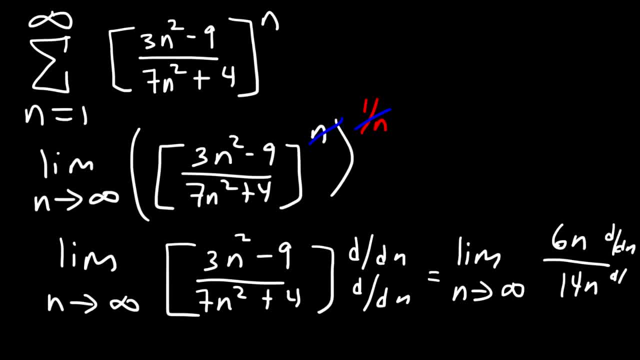 Is fourteen n. So using L'Hopital's rule again, This is going to become Six over fourteen, Which reduces To three over seven. So this is the answer. Now, Three over seven Is less than one, So based on the root test, 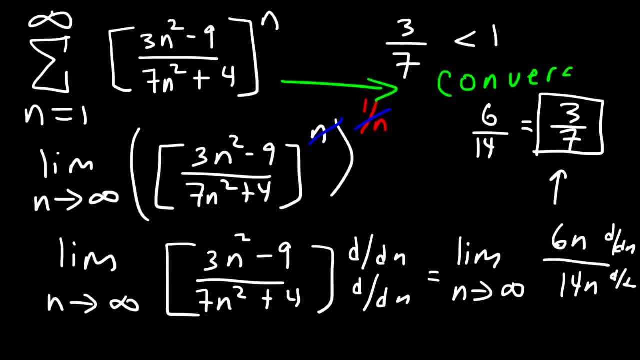 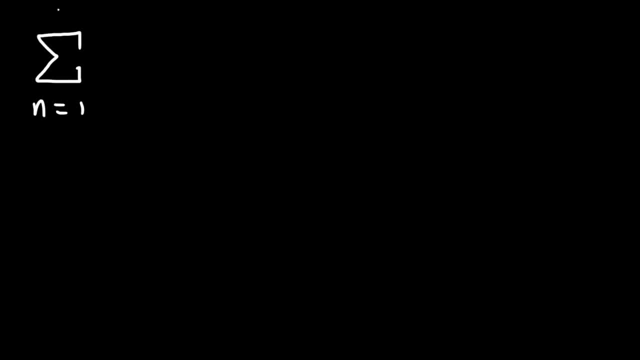 The series Converges. Now let's work on our final example. And so we're going to have the series Of two raised to the n, Divided by n- factorial. So what test Should we use for this example? So, since you know, 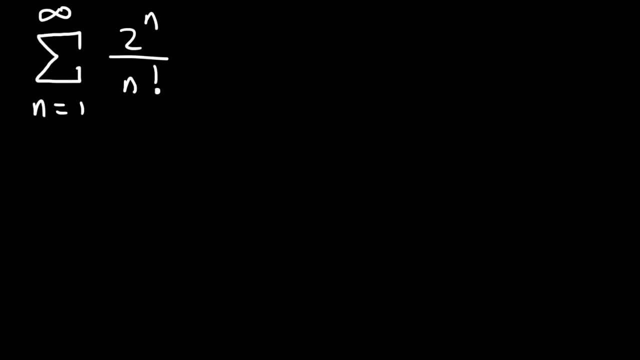 It's the last problem That we haven't used yet, Which is the ratio test, And so the basic idea Behind the ratio test Is we need to take The a sub n plus one And divide it by a sub n. 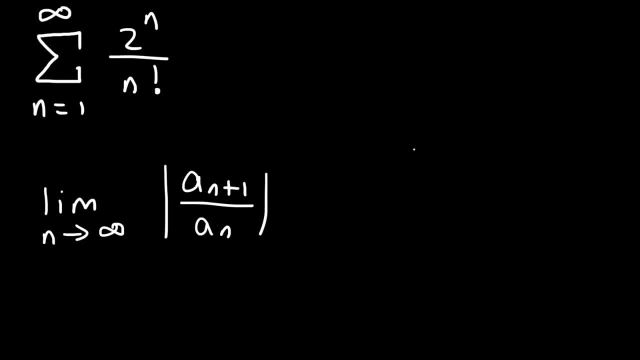 All within an absolute value symbol. And if this is less than one, The series converges. If it's greater than one, Or equals infinity, The series diverges. Now, if it's equal to one, It's inclusive. Now, we know that. 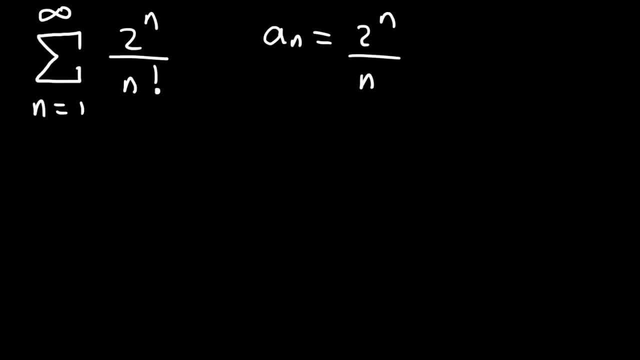 A sub n Is two to the n over n- factorial. But what's a sub n plus one? All you need to do is Replace n with n plus one. So the limit As n approaches infinity Is going to be a sub n. 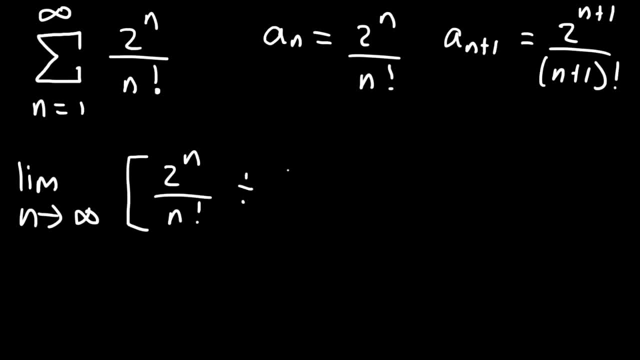 And then divide it by. I mean, I take that back. If it's a sub n plus one, We need to write that one first And then divide it by A sub n. Using keep change flip, We can say It's multiplied by: 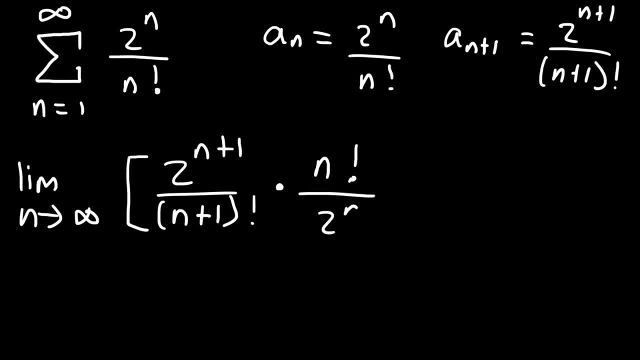 One over a sub n Or the reciprocal of a sub n. So this is A sub n plus one Times one over a sub n. So you can represent it that way If you want to. So how can we simplify the limit now?